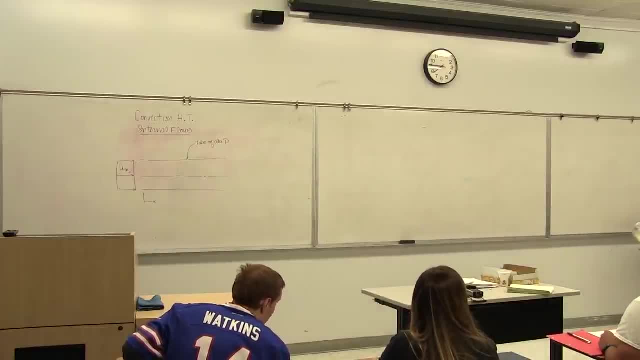 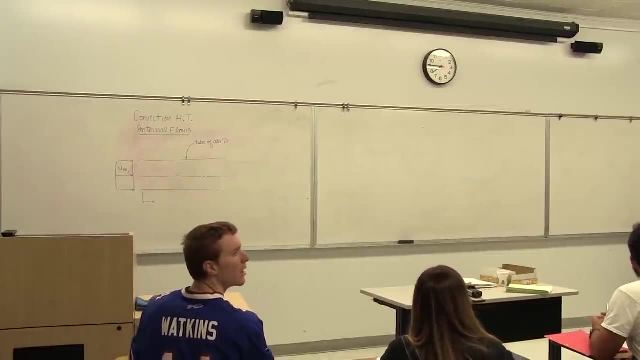 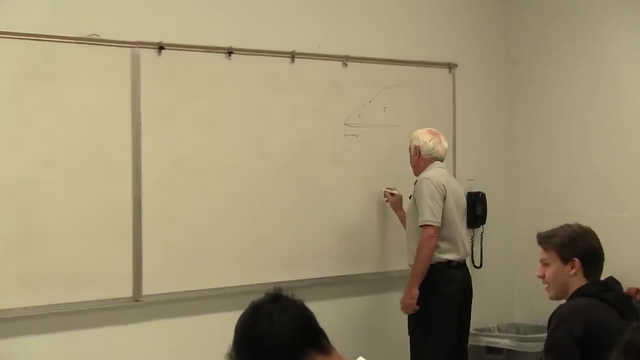 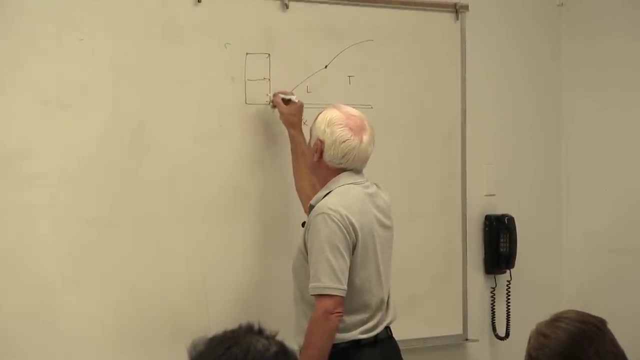 just a quick look at that. So chapter 7 had flow over flat plate. It may be laminar and turbulent, called mixed flow. maybe We measured x in that direction. Then we had flow over a cylinder. This was U infinity. Flow over a cylinder, the flow. 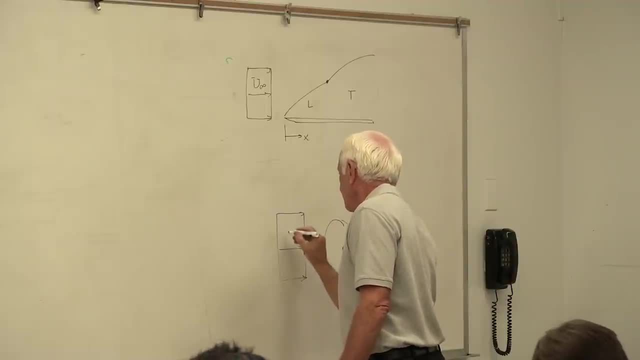 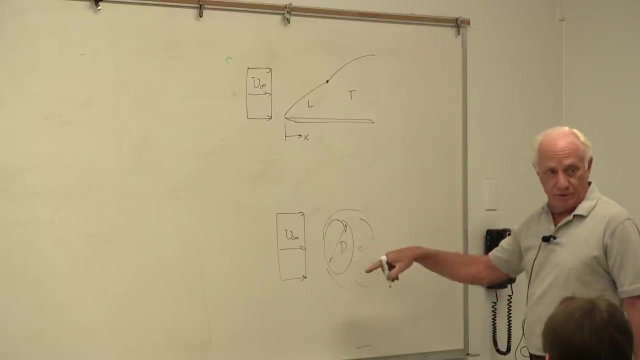 approached the cylinder with a velocity U, infinity, Okay, And this was a tube of diameter D. These were external flow. This was chapter 7.. This was a tube flow over a tube normal to the axis. This is flow- chapter 8, inside. 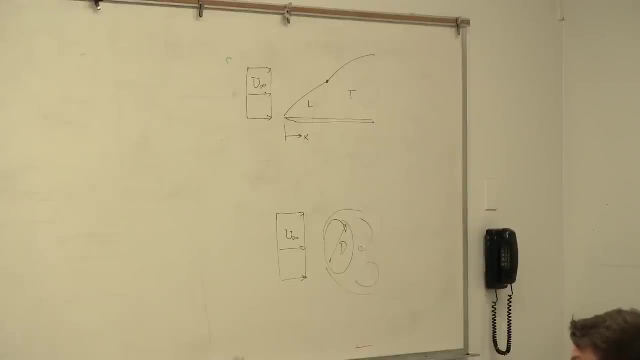 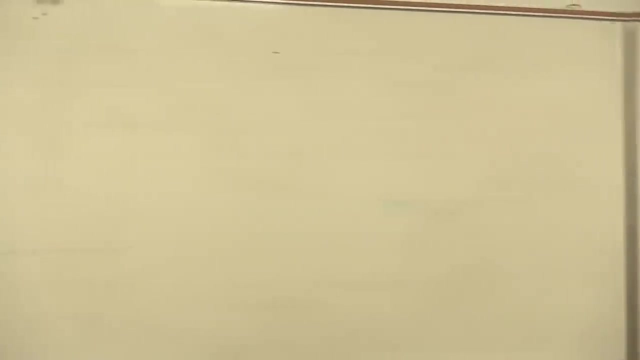 of a tube. So now we kind of shift gears. Chapter 7, we had flow over the outside of a tube. Chapter 8, we have flow on the inside of a tube. Same thing with chapter 7.. Before you do the heat transfer you have to understand a lot. 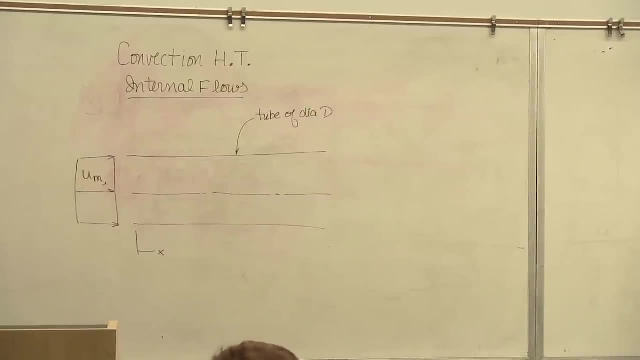 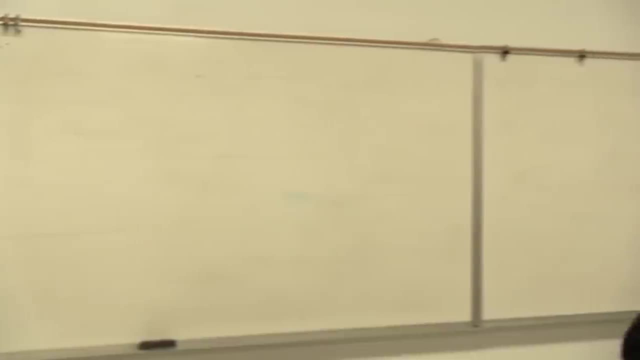 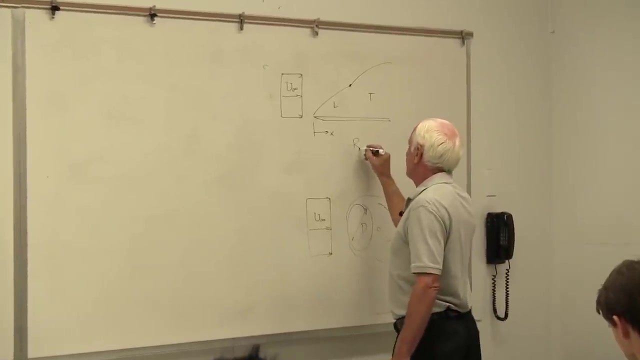 of the fluid mechanics. Okay, There's some magic Reynolds number. This is 500,000, the transition from laminar to turbulent, 5 times 10 to the fifth, 500,000.. This Reynolds number was based on the distance: x, U, infinity, x over nu. This Reynolds number 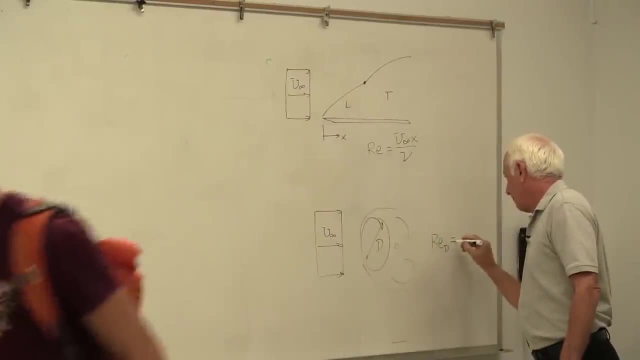 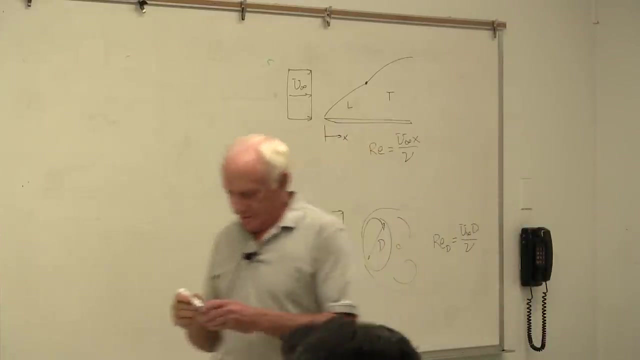 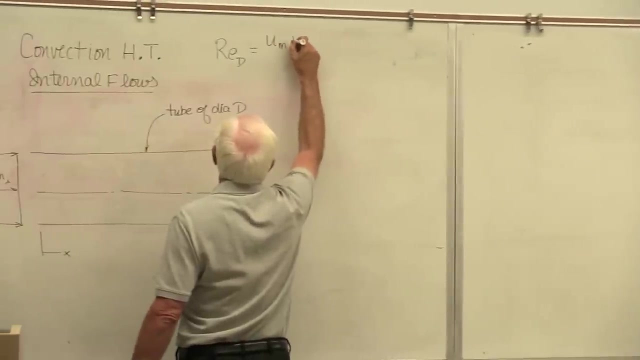 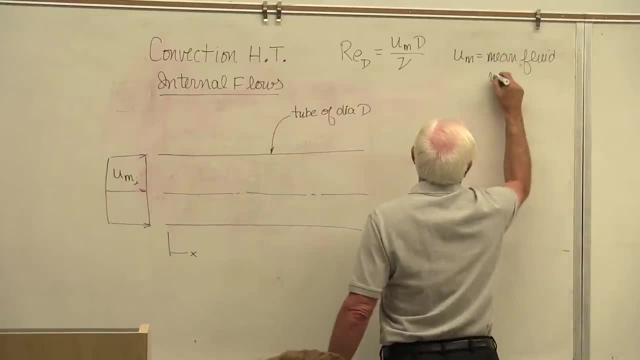 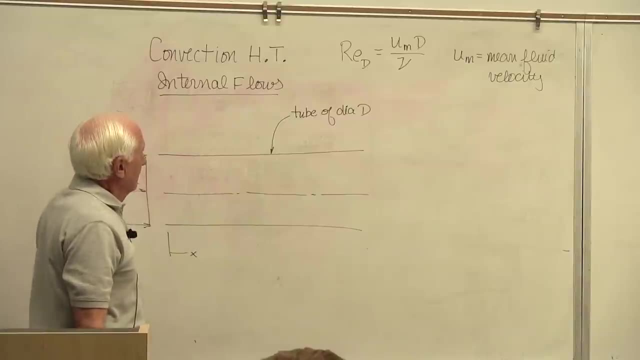 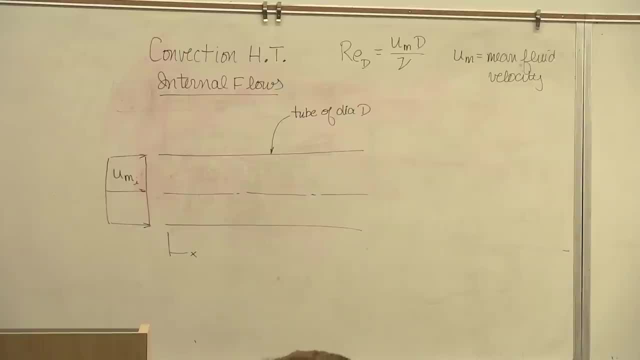 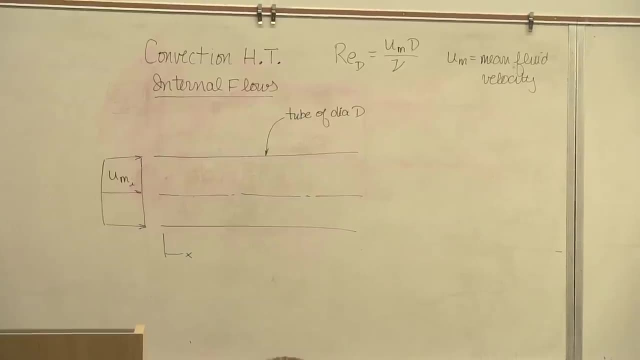 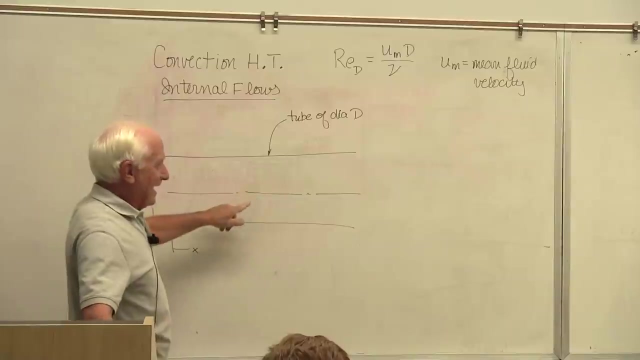 U M. Of course, in the real world, this D and that D are not the same thing. This is the outside diameter of a tube and that's the inside diameter of the tube You're. But we won't worry about that now, as long as you know that chapter 8, it's the ID. 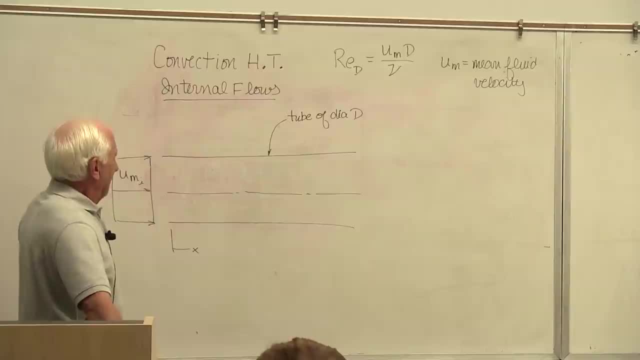 Chapter 7, it's the OD of the tube. If somebody says the mean velocity, if somebody says the velocity of the fluid in the tube is 10 feet per second, let's say it's laminar flow. Here's the velocity profile. 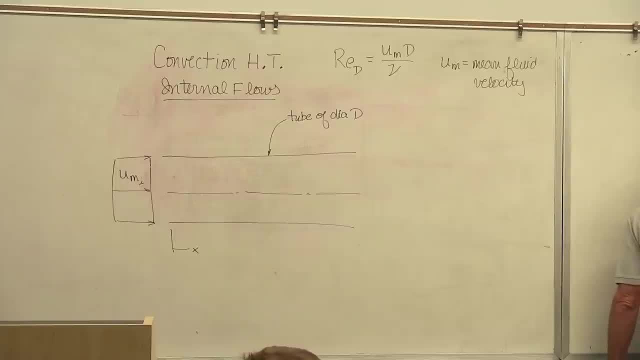 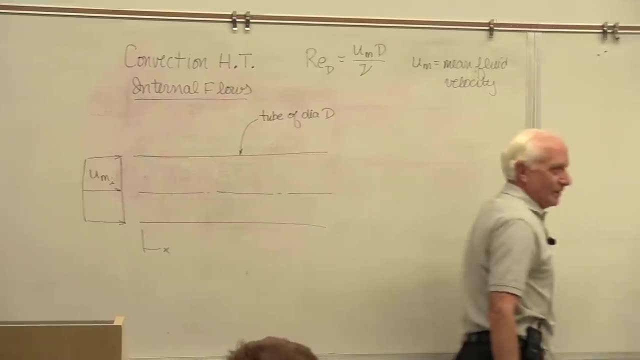 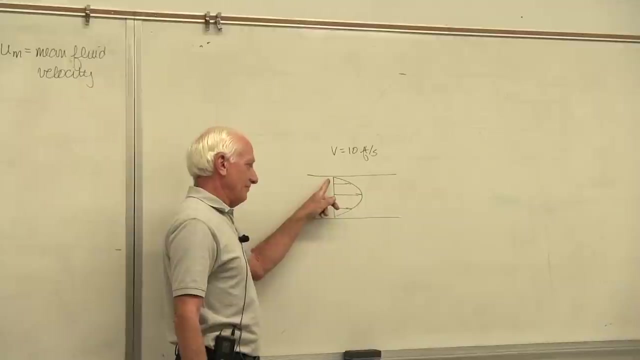 It's parabolic for laminar flow in a tube. And if somebody says the velocity in the tube is 10 feet per second, well they sure don't mean the center line velocity is 10 feet per second. They don't mean the velocity at the tube surface is 10 feet per second. zero, no slip condition. 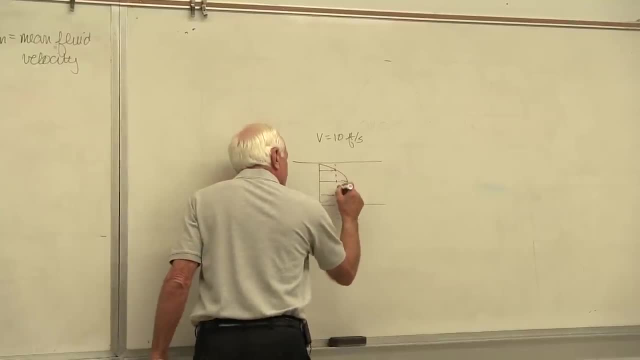 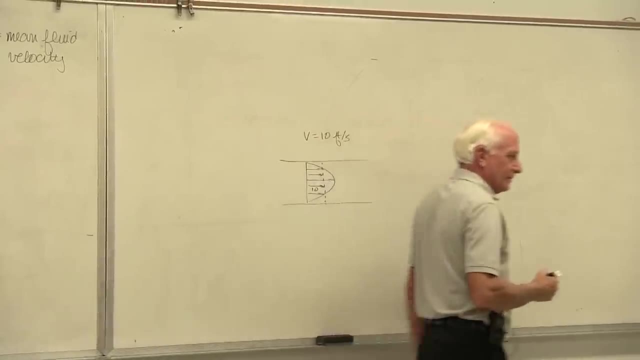 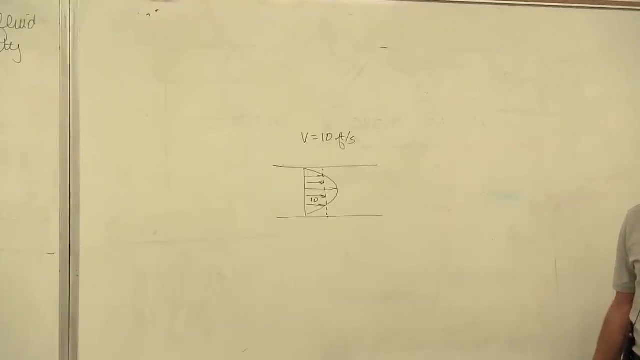 What do they mean? They mean that this would be 10 right there. So that's the mean fluid velocity. Do you just average it? a 10 plus zero, divided by whatever two? No, no. For instance, if this velocity on the center line, if that center line velocity is 12 feet, 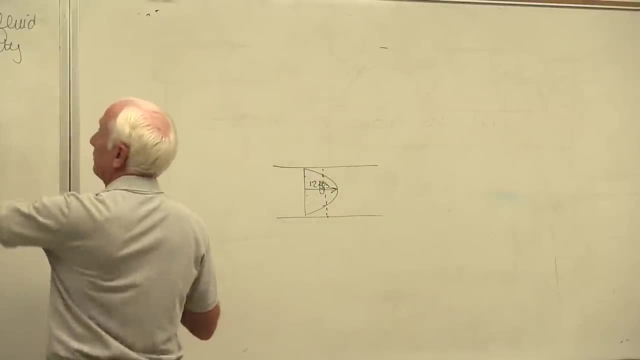 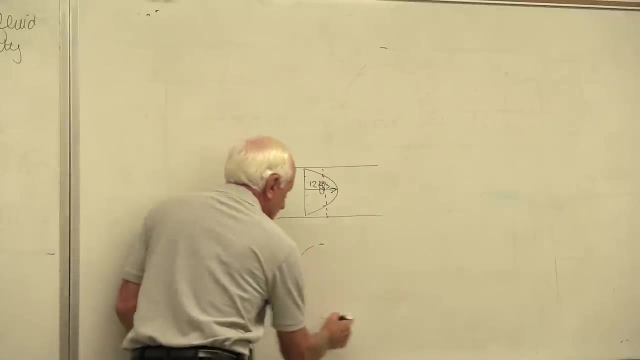 per second is the mean fluid velocity 12? Divided by two? Uh-uh No, no, Uh-uh No. It's because the cross section looks like a circle And there's a lot more area out here than there is in the middle. 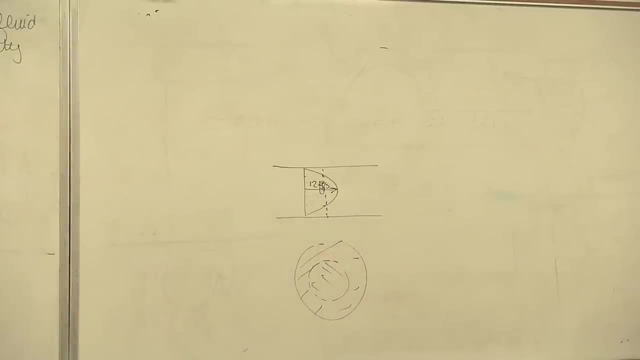 So it's called a weighted average. It's a weighted average. You just don't take the center line velocity. It's not like this. Well, I'm not even going to draw it. OK, Go back to math. OK, So, 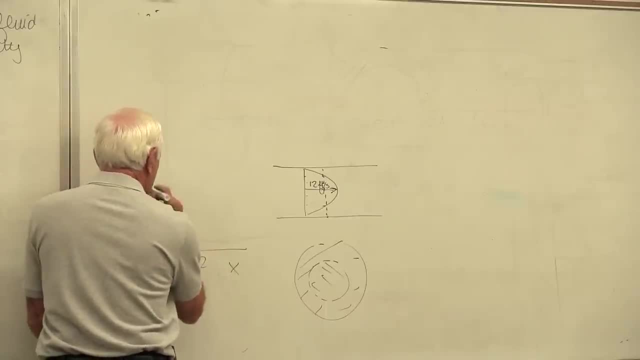 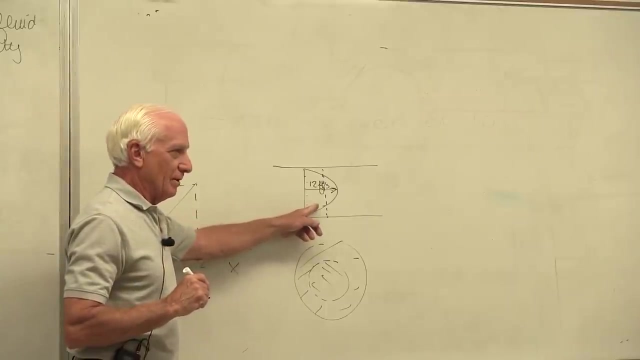 What's the average value of y from zero to two? Oh, it's five. 10 divided by two, It's five. I guarantee it's five. No, it won't work here. It won't work here. This is not a linear profile and it's not a one-dimensional profile. OK, 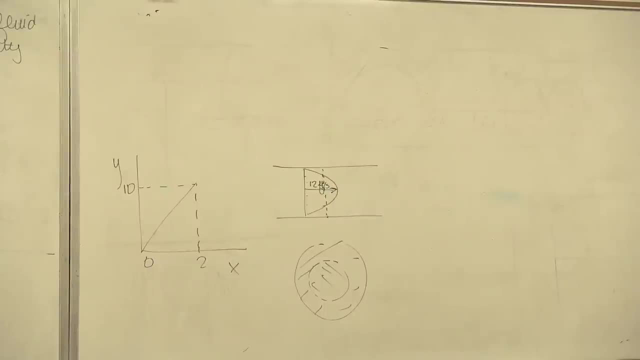 So anyway, that's what the word mean is. That's why they don't use the word average, And sometimes that confuses people. They think average, oh, take this, divide it by that and that's the average Half of that value. 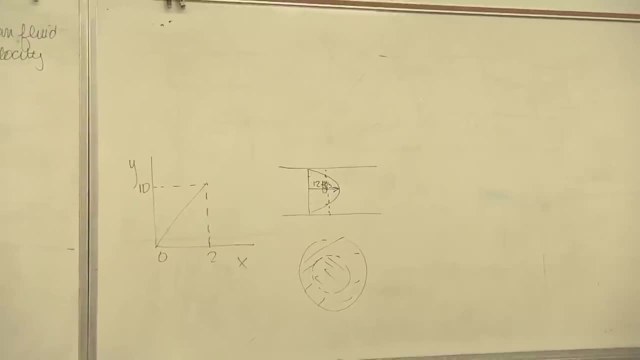 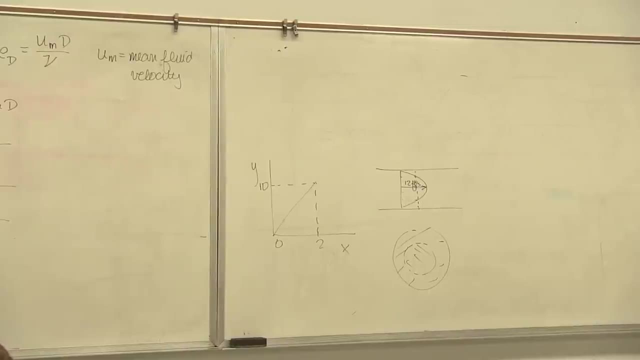 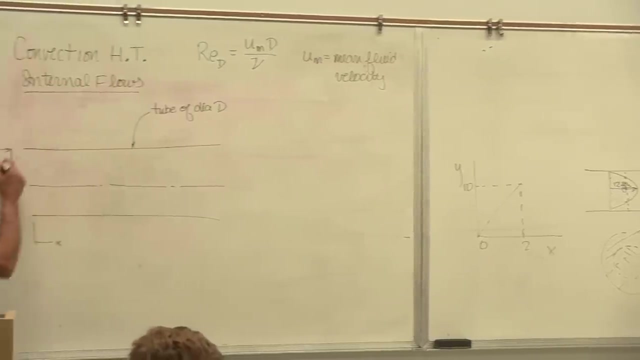 No, That's not the average, And you did that in ME 311, so I'm not going to revisit that. OK, Anyway. So here's what happens. We assume we've got the tube. There's an approaching fluid stream whose velocity is um the subscript i means inlet. 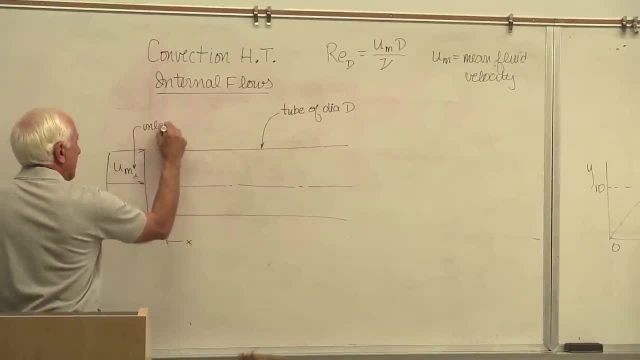 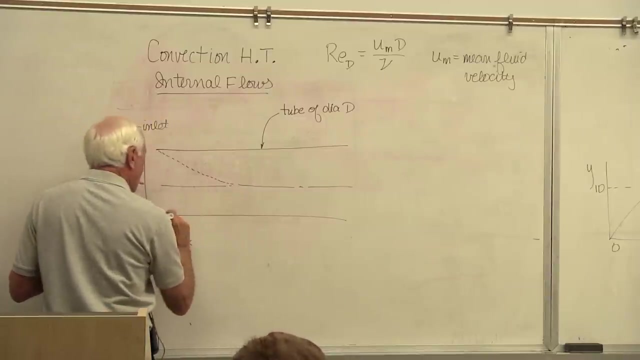 So i means inlet, m means mean. So this is the mean velocity at the inlet When it hits the tube. at x equals zero, a boundary layer starts to build up around the perimeter of the tube, a boundary layer. That boundary layer develops from all around the perimeter, all around the perimeter. 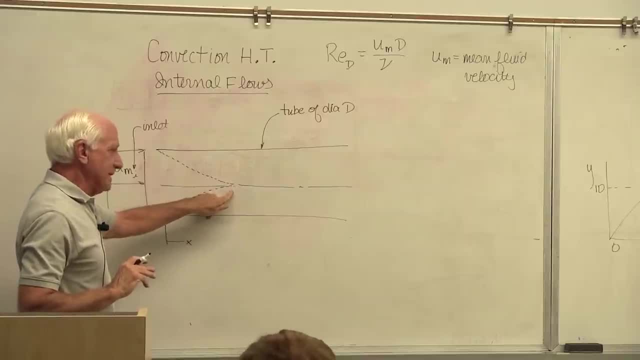 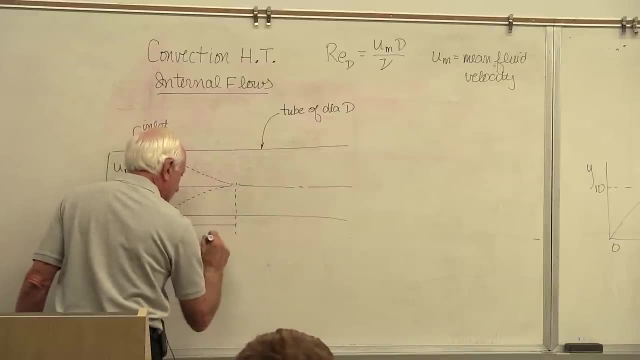 It develops When the boundary layers meet at the center line. that's a special region called the entrance region. That's where the entrance region ends And that distance is x, fully developed. XFD is the fully developed distance And what it's developing inside this. 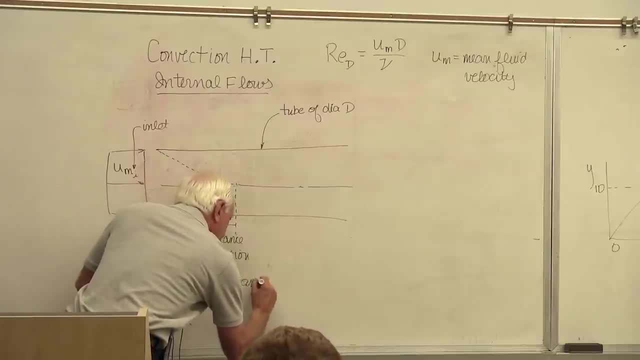 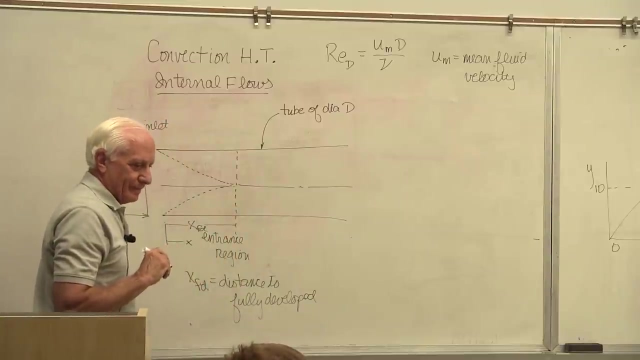 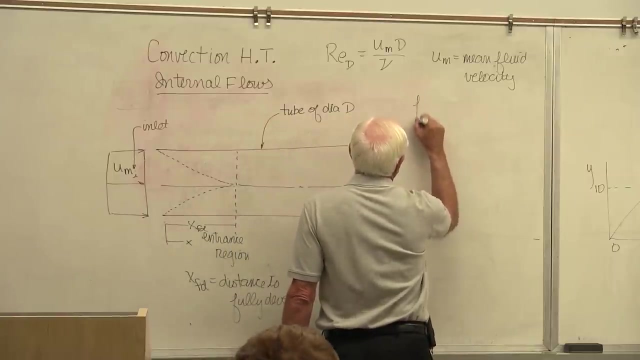 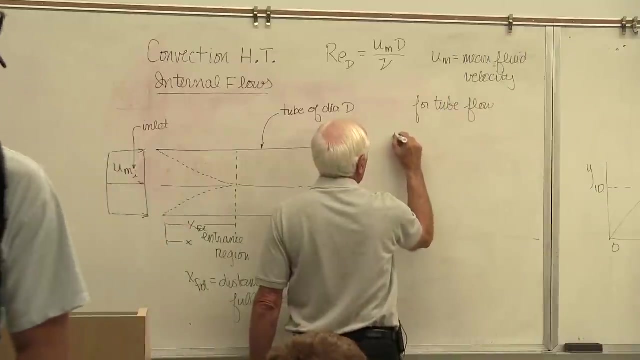 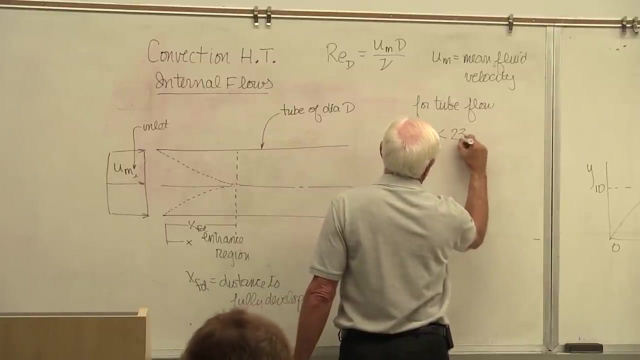 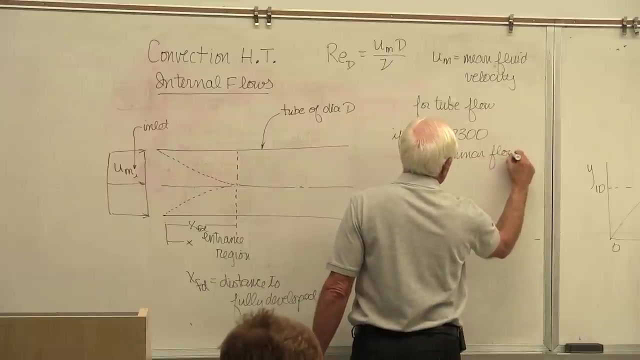 Attry occupation is high methods of processing, operating and the Wissenschaft of出來 Milliwagi standard Neurologist Spe walls, lt, l, l, b, C, L, a. Let's just assume it's laminar. Let's talk about in a tube ME311, if the Reynolds number is less than 2300, we're going to assume. 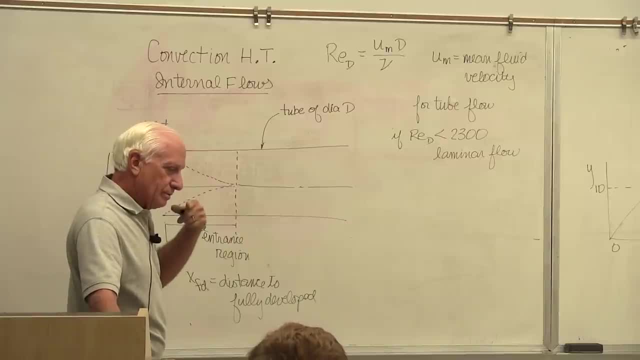 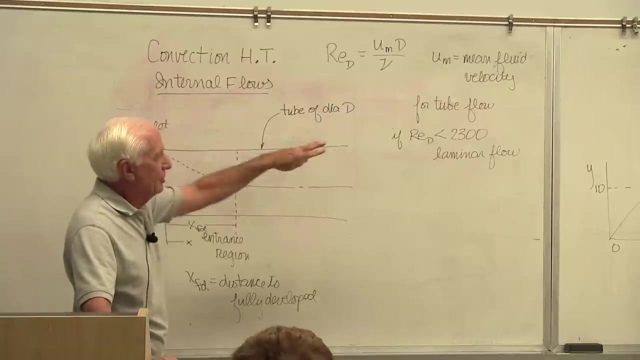 it's laminar flow. Different textbooks sometimes use different numbers. One textbook uses 2100.. Our textbook uses 2300.. There's no one universally accepted value, So our book uses 2300.. So for this class we'll use 2300.. If it's greater. 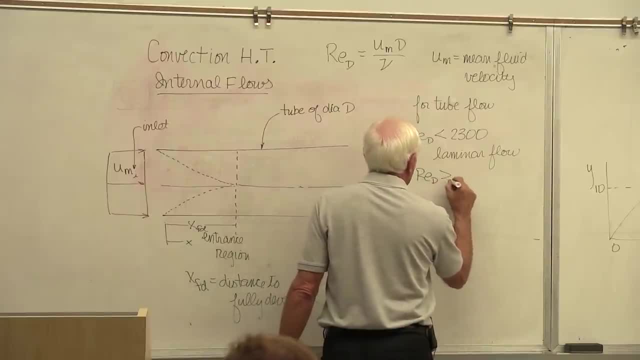 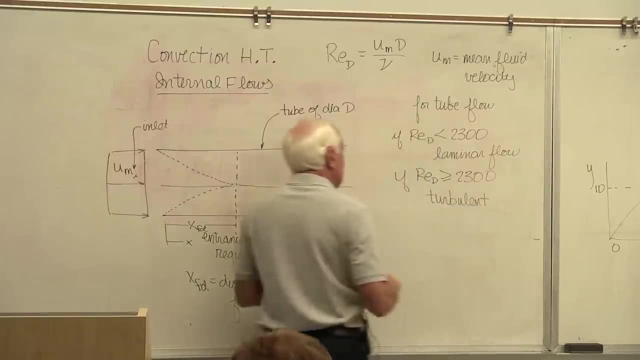 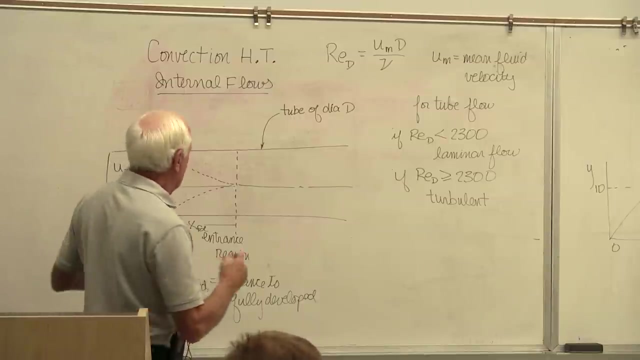 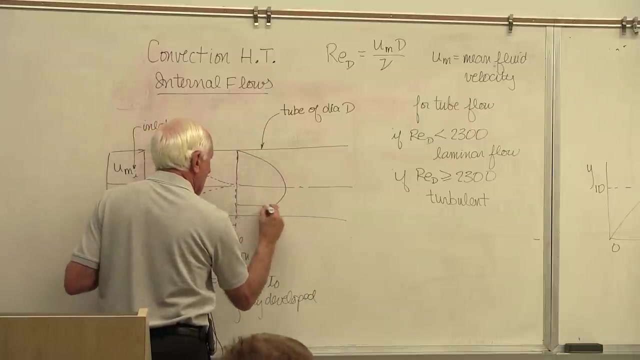 than that, of course it's turbulent. Okay, So for right now we'll just assume laminar flow. make it easy on ourselves. If it's laminar flow in a tube, we know from fluid mechanics that the velocity profile is parabolic. Parabolic, Fully developed means, if I go down a ways and look at it again, 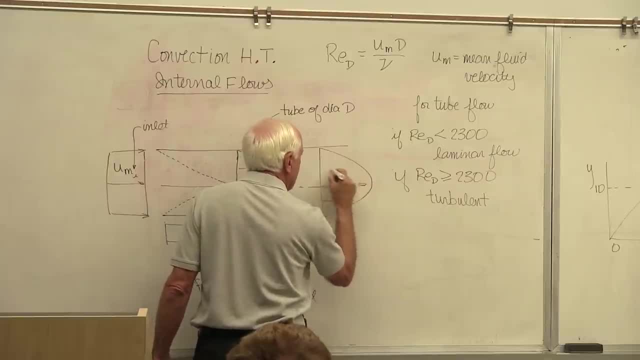 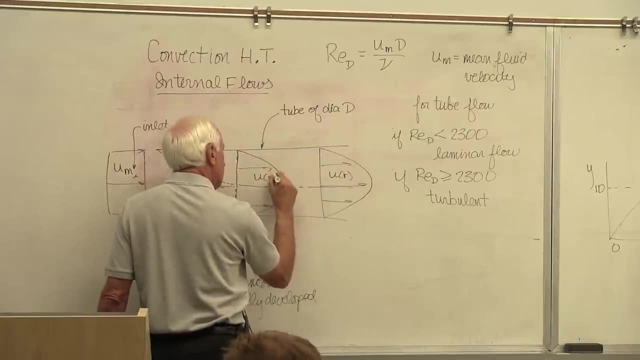 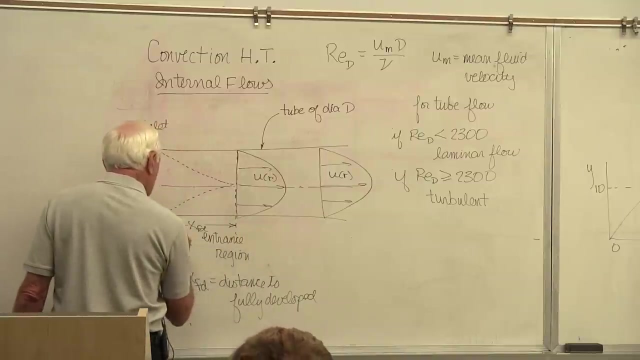 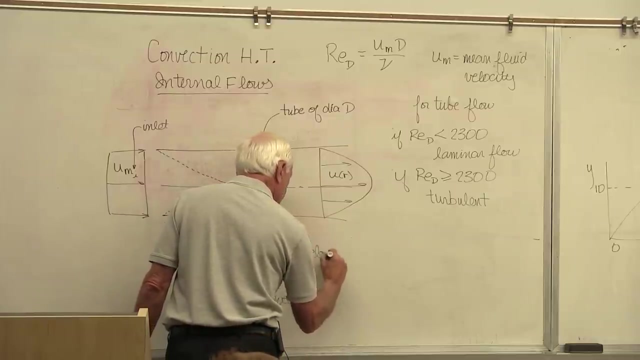 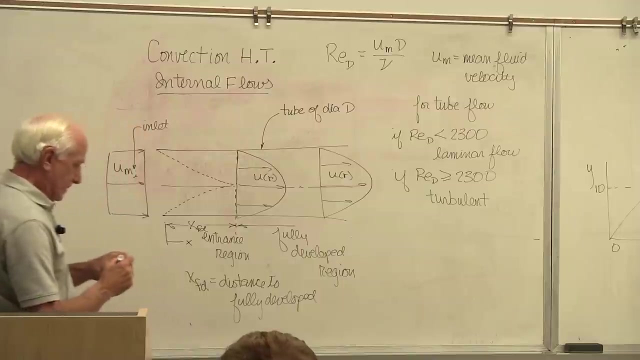 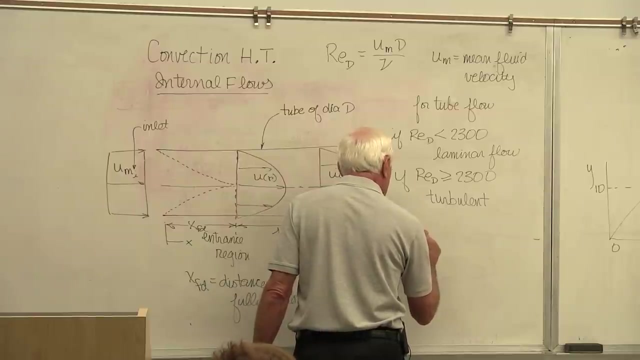 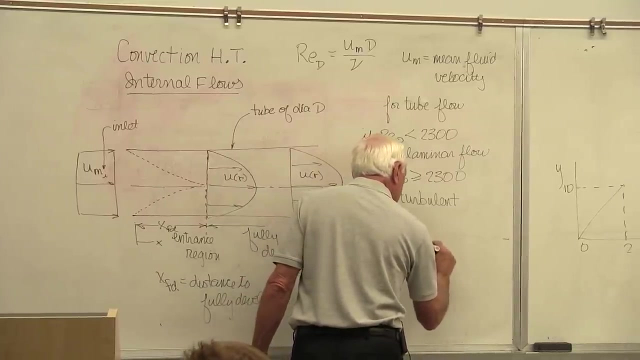 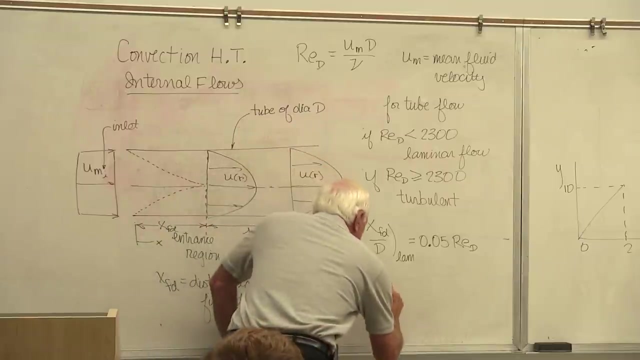 it's the same shape parabola. It didn't change. This is the velocity U as a function of R. the profiles don't change. That's why that's called the fully developed region. Okay, The distance it takes to become fully developed for a laminar flow: 0.05 Reynolds D If it's. 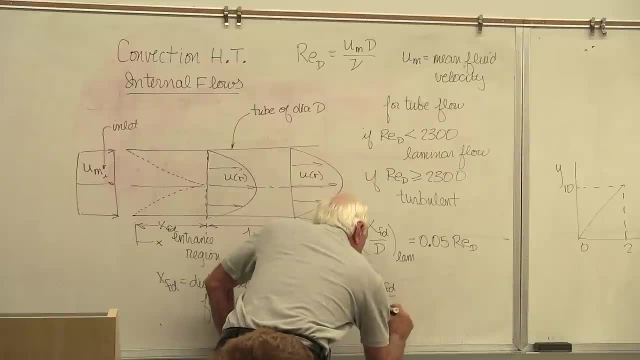 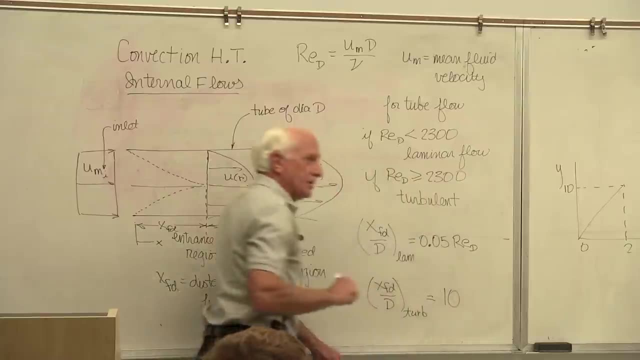 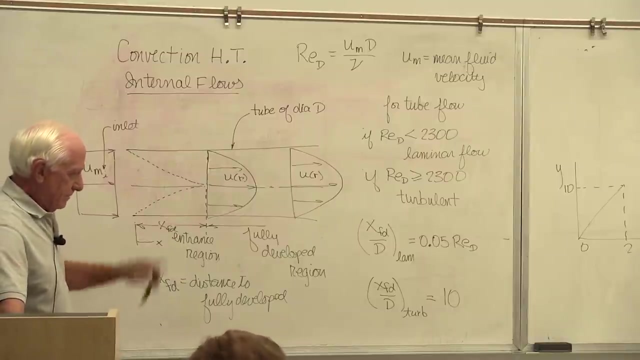 turbulent flow. the book says we're going to use 10.. Okay, It's typically accepted between somewhere from 10 to 60. That's how you'd find X fully developed. Our textbook says, to be conservative, we'll say 10. Okay, So that's the two equations. 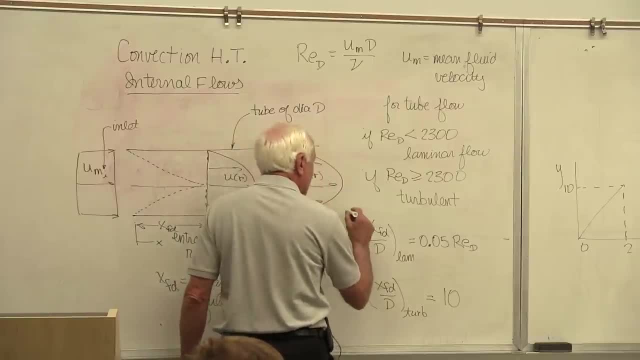 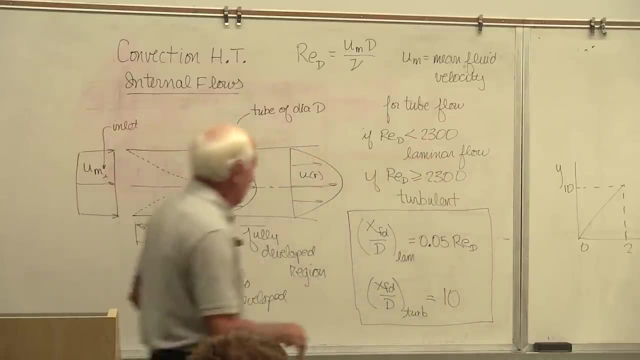 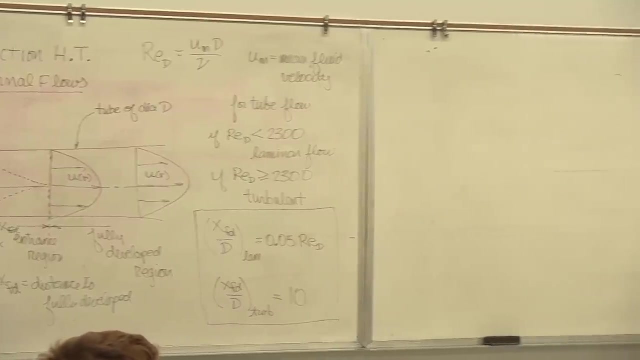 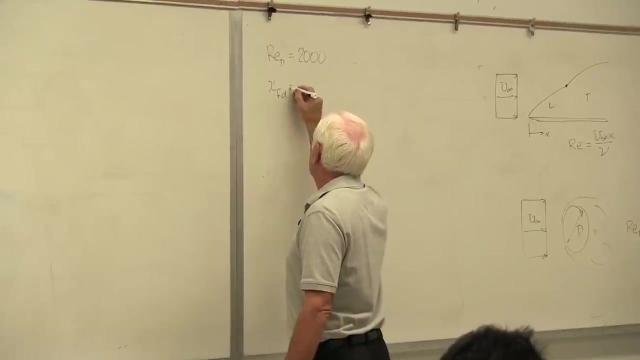 you use to find this distance XFD. So how do you find XFD? Okay, Fluid mechanics. there they are Now. Okay, Let's say the Reynolds number is 2,000.. So I'll say it's laminar flow X, fully developed. 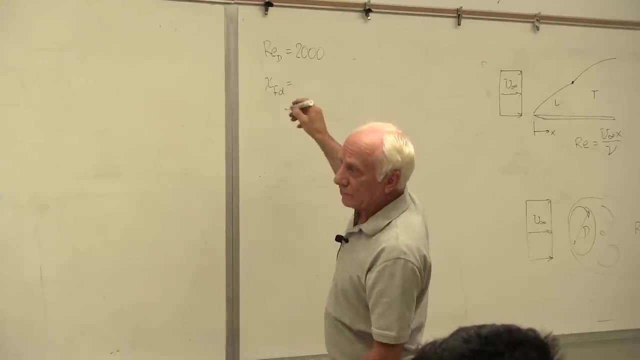 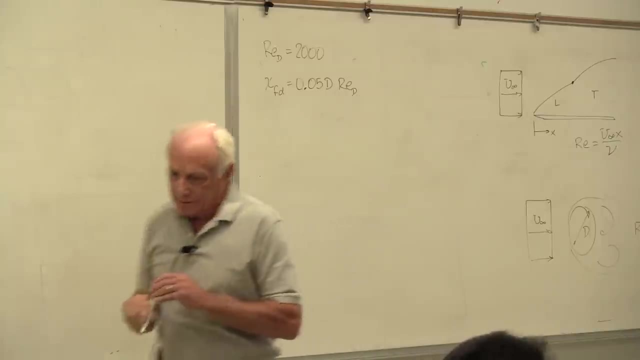 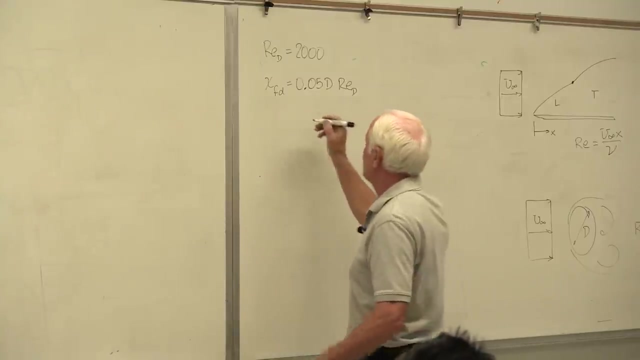 equal the 0.05 times the diameter times the Reynolds number based on D. Let's see what I assumed here. Okay, Okay, I said let it be a 1-inch diameter tube. If D is 1 inch, then X fully developed from. 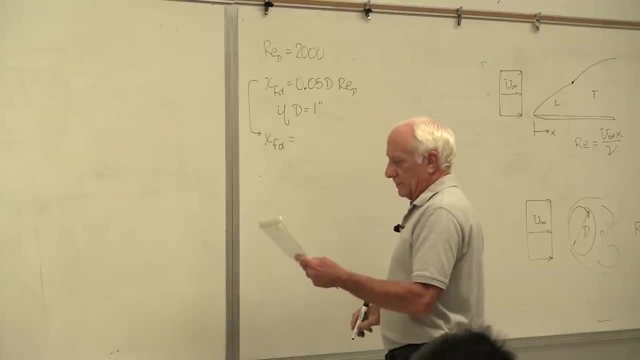 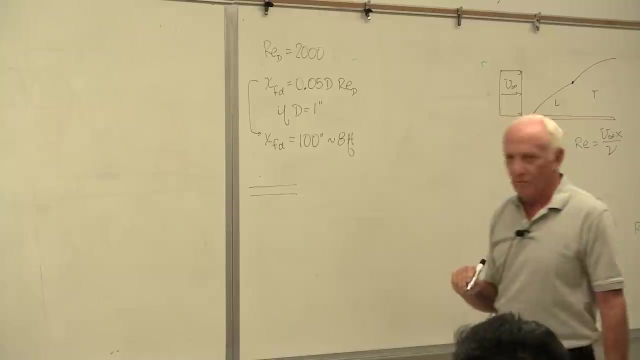 this equation: right here, X, fully developed, is 100 inches, which is on the order of 8 feet. Okay, Okay, Okay, Okay, From there to there, that's a little more than 1 inch. Okay, There's 1-inch tube and. 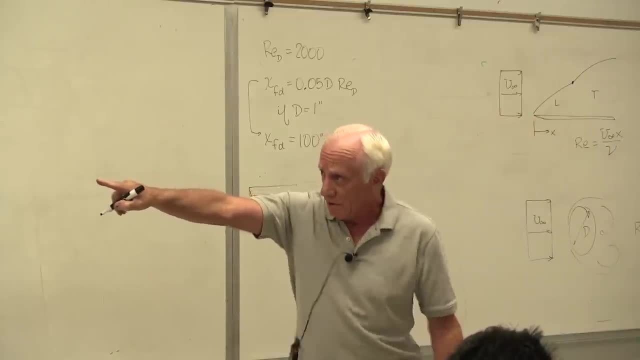 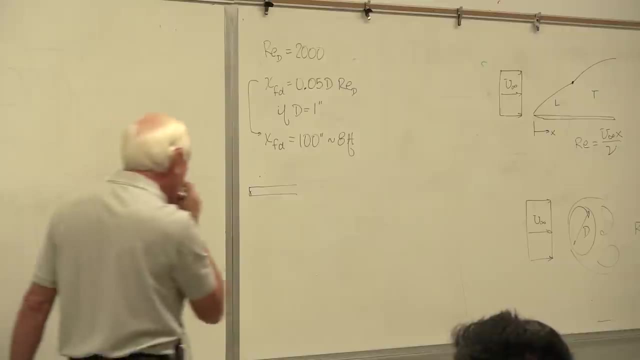 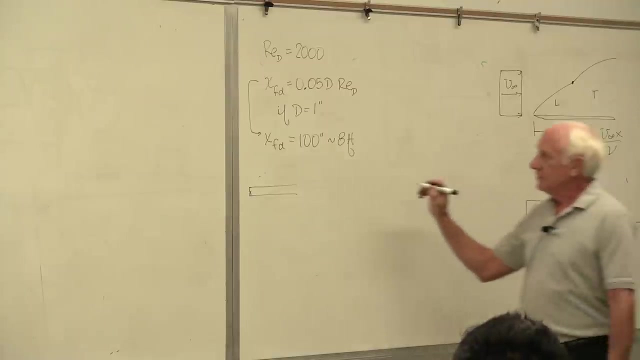 those boundary layers build up from the entrances over there. Where do these two dash lines meet, the centerline of the 1-inch tube? Oh boy, Three, six, seven, eight, right here, Okay, Okay, Okay. So it would take that flow this long a distance before, finally, the boundary layers meet at. 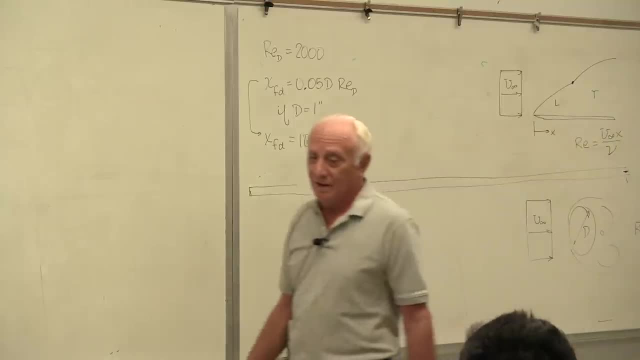 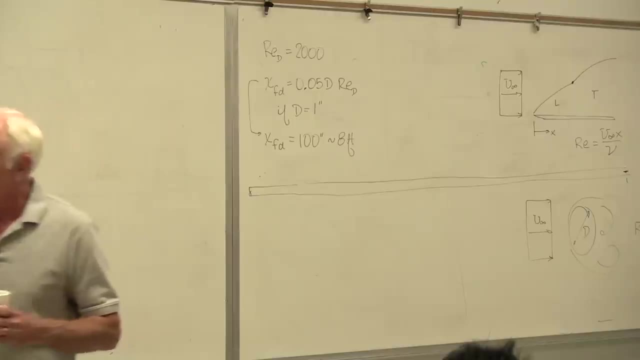 the center line of the tube. Oh, it's a long, long way, a long long way. Should we engineers be worried about what happens in the entrance region of a tube? Oh you better, because you know, a one-inch tube with a Reynolds number of 2,000 has to. 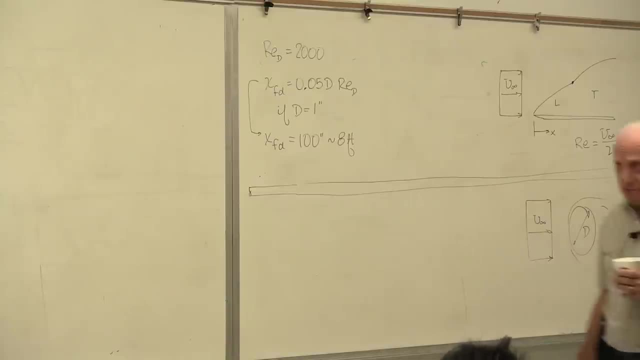 be eight foot long before you get out of the entrance region, before you get out of the entrance region and into the fully developed region. So, oh yeah, Take turbulent flow. Take a Reynolds number based on D. I think I took D. 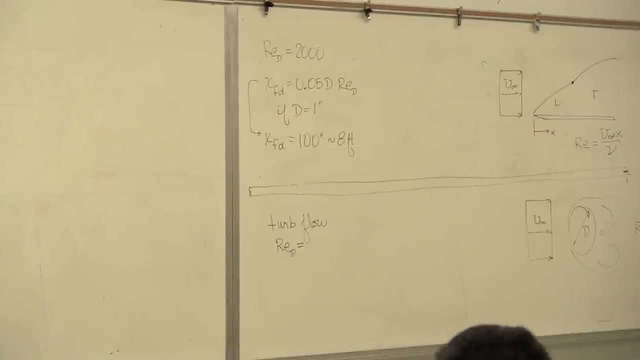 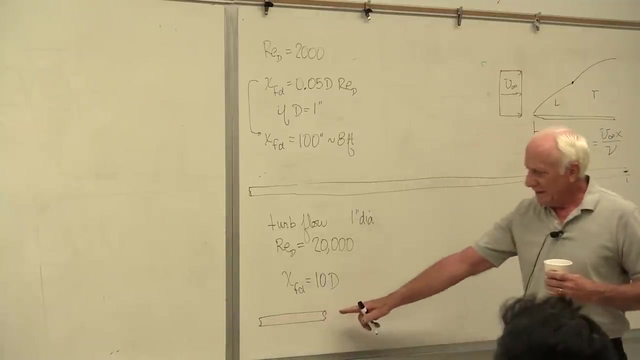 20,000, 2 times 10 to the 4th X is X fully developed D times 10.. What's D? one inch, A one-inch tube, 10 inches, wow, wow, For turbulent flow. those profiles develop very fast and meet at the center line very 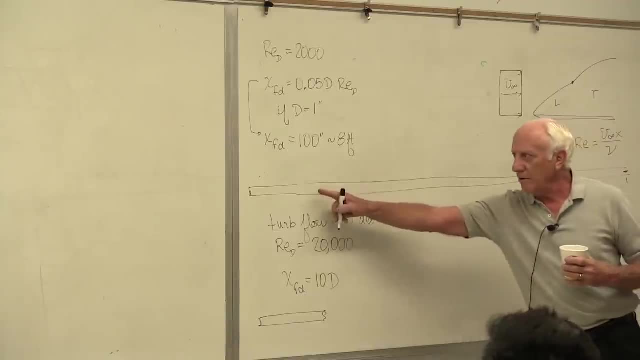 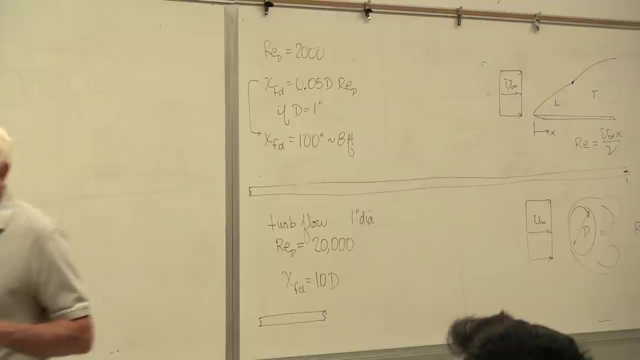 very short distance, 10 inches- compared to laminar flow, a hundred inches long. Oh yeah, Oh yeah, It's a big difference in laminar and turbulent flow. Oh yeah, Where do you worry about that? Oh, I'll just give you one idea. 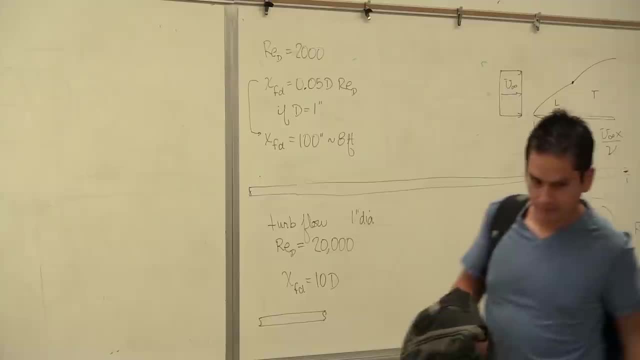 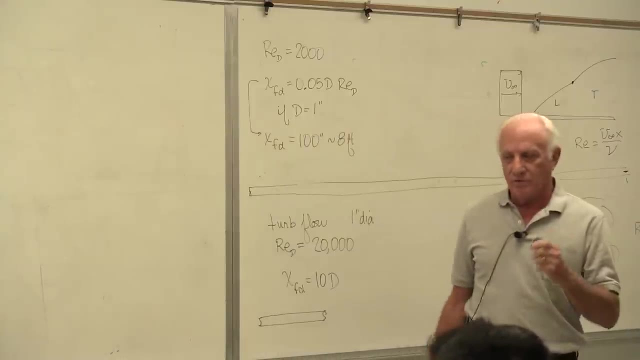 Your automotive radiator. Is there tubes in that thing? Oh, of course there is. They're vertical. What do they carry? Yeah, hot water. How do you cool them? Blow air over them with fins. Is the flow in those tubes laminar or turbulent? 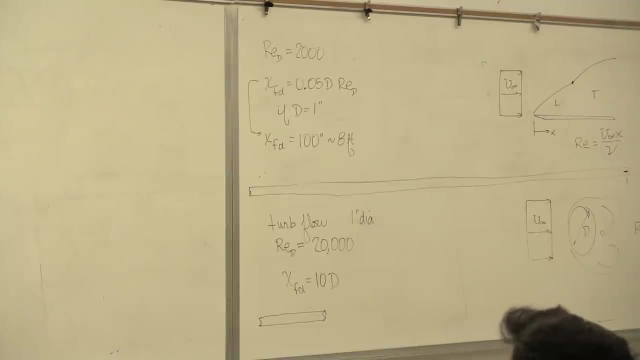 Oh, I suspect it's turbulent. you know It's hard to get laminar flow in anything. I'm at a real good intuitive guess, An engineering intuitive guess: It's turbulent. Okay, What's those diameters of those tubes? 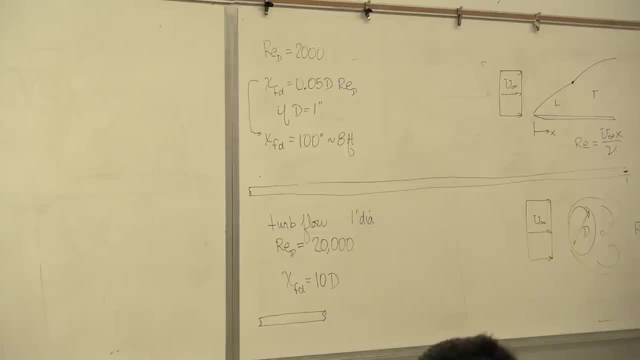 I don't know, Maybe that big, maybe a quarter inch, three-eighths of an inch, I don't know. Ten times a quarter inch, two and a half inches. Oh, they develop pretty quick, don't they? The flow that comes in the tubes in the radiator develop pretty quick, I think, to fully develop. 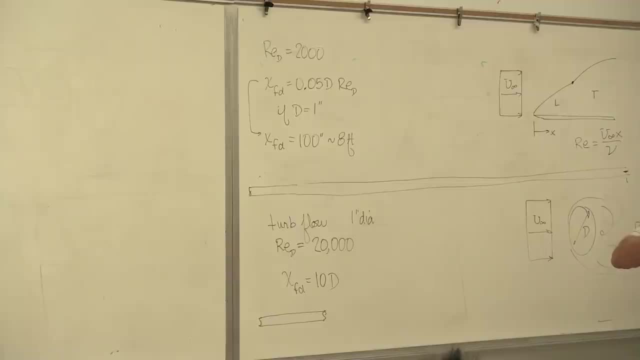 because you might have 12 inches or 14 inches of the radiator height And they develop in two and a half inches maybe. So, anyway, that's the kind of decisions you've got to make: to see what's going on in your automotive radiator or your trans oil cooler or your oil cooler. 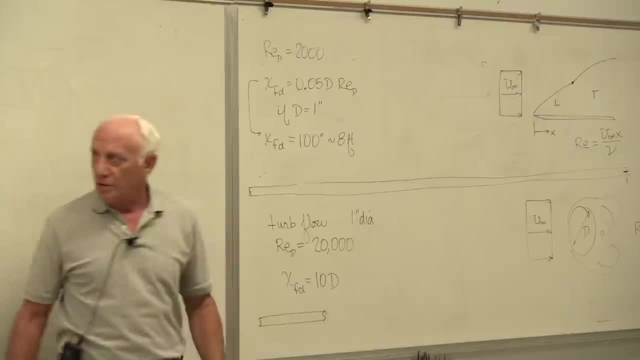 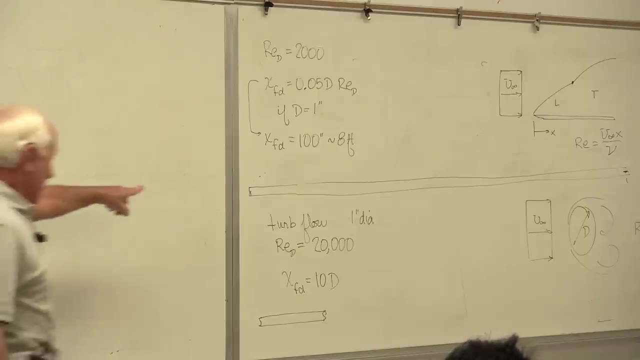 How quick do the boundary layers build up to where you have fully developed flow, Or is most of your tube in the entrance region? If this is laminar flow and my tube is two feet long, chop it off here. It's all in the entrance region. 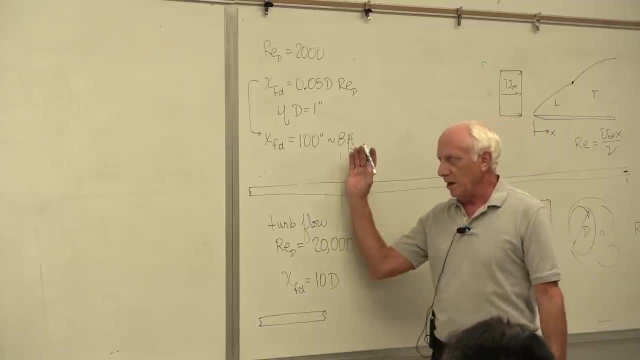 It's all in the entrance region. There is no fully developed for a tube that long. One inch tube two feet in length. no, It's all in laminar flow. It's all going to be in the developing region. So that's why it's important to know what's going on in these regions. 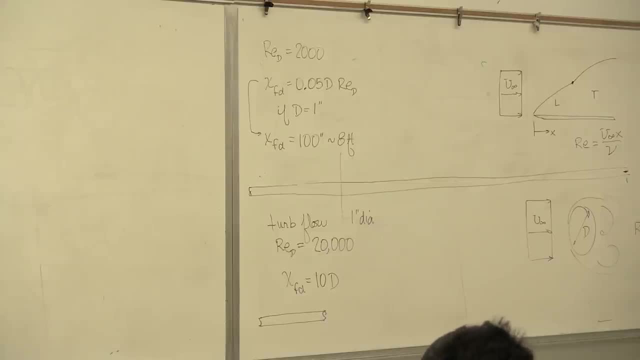 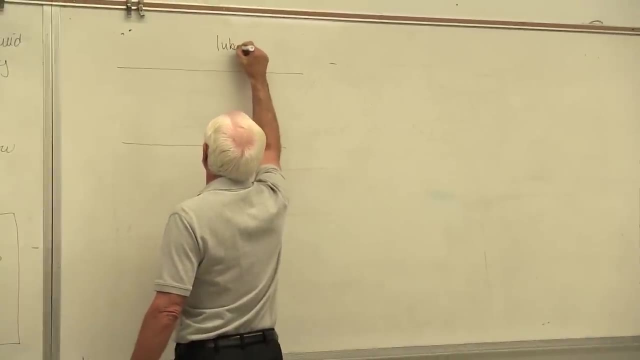 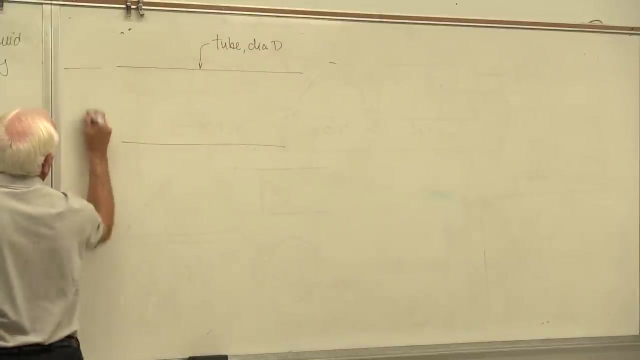 This is a fluid mechanics case. Now we do the temperature. same kind of picture. Here's the tube: diameter D: Okay, But now we're looking at the thermal situation, which is what's approaching the fluid or the tube. The fluid is at a temperature T mean in. 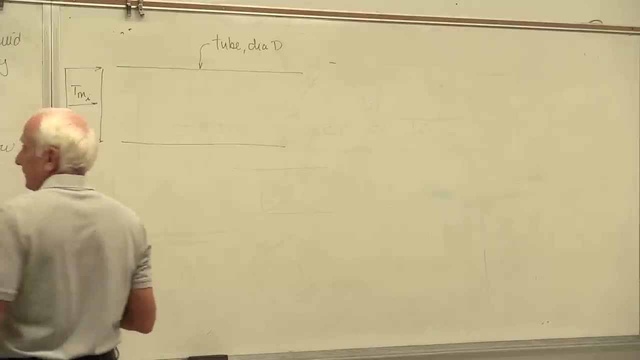 Let's go back to Chapter 7 one more time. What's approaching the flat plate? U infinity. What's coming into the tube? Don't say U infinity. There's no such thing as a free stream temperature in a tube. Umi flat plate external flow over a tube. 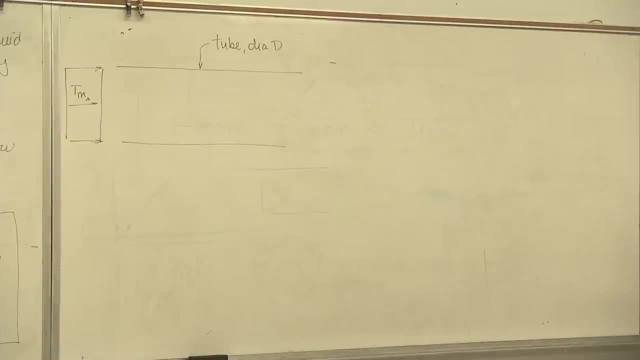 What's the approaching temperature? T infinity, the free stream temperature. There is no free stream temperature in a tube. We call it the inlet temperature of the tube. yeah, Tmi inlet temperature of the tube. When, At profile hits the tube, a boundary layer starts to develop a temperature boundary. 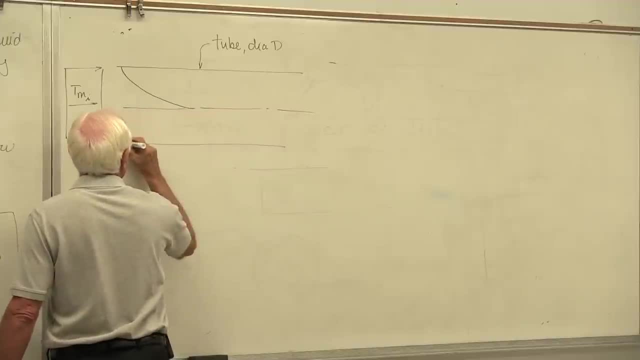 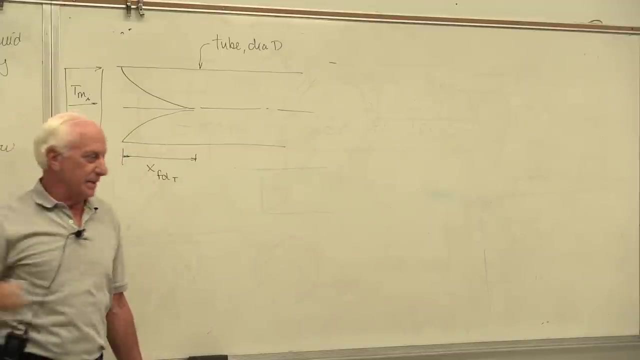 layer And eventually that boundary layer meets at the center line. The distance from the tube entrance to the center line is called X, fully developed. Sometimes they put T on there for temperature. If there's no subscript, they mean velocity. And this is the entrance region. 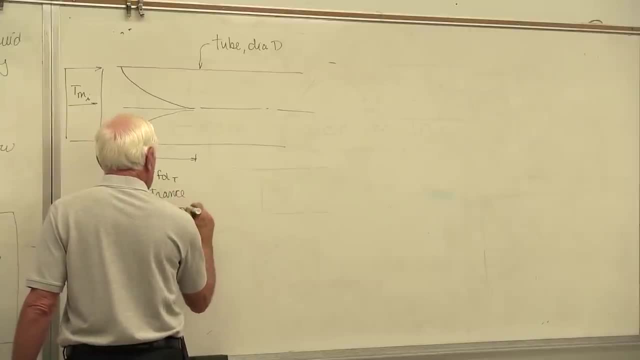 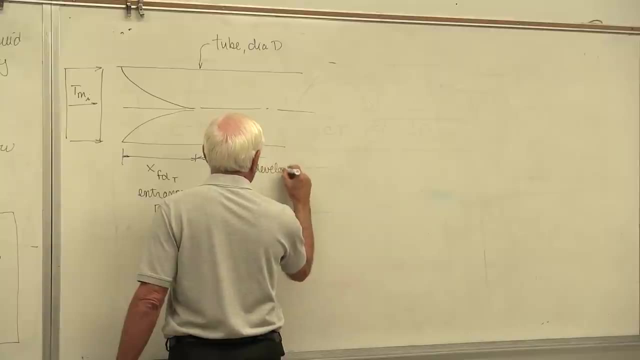 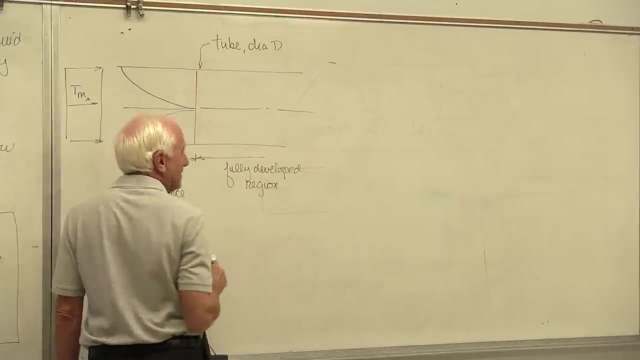 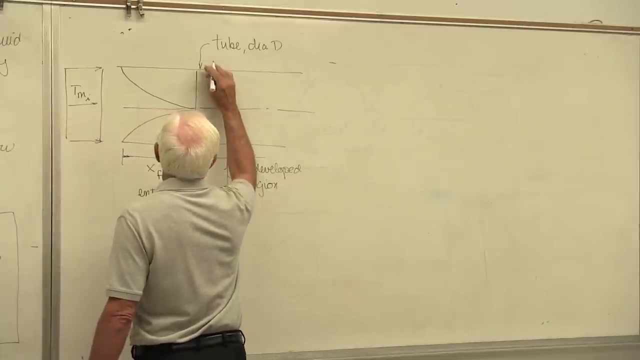 Okay, And this is the fully developed region, And this is the fully developed region. Okay, Now there's different conditions with the temperature. Let's draw a profile here. where the tube surface temperature is constant, This is T. This is T. 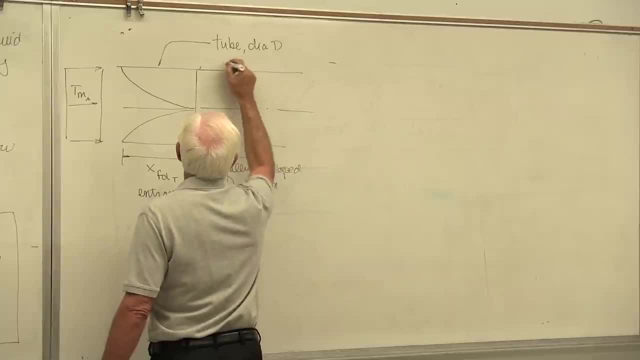 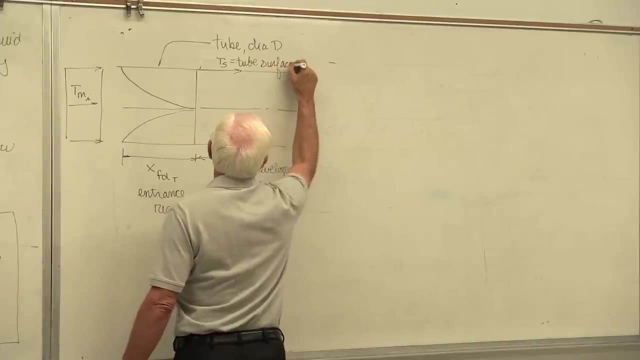 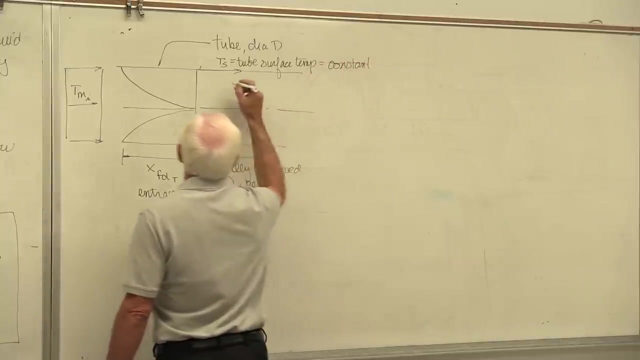 This is the temperature in the tube. This is the temperature in the tube. We're going to draw a profile here. This is Ts tube surface temperature and we'll call that constant. Let's say the fluid that comes in is cooler, a colder fluid. 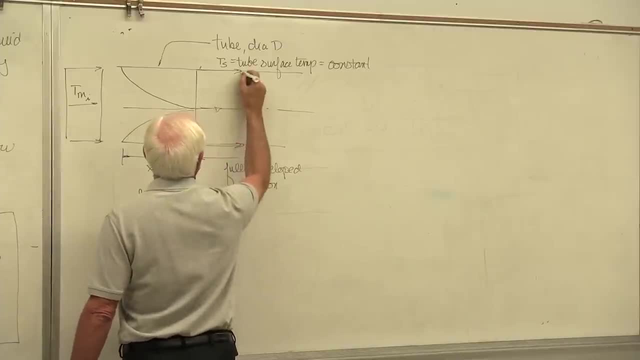 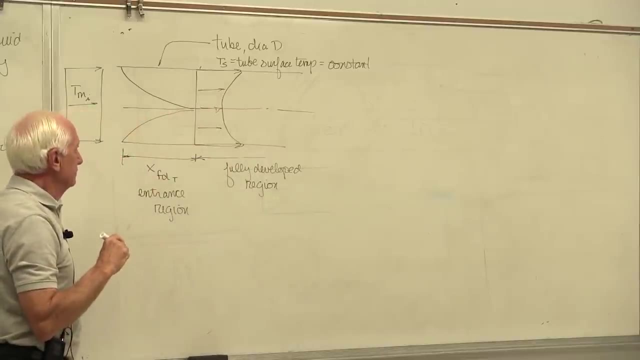 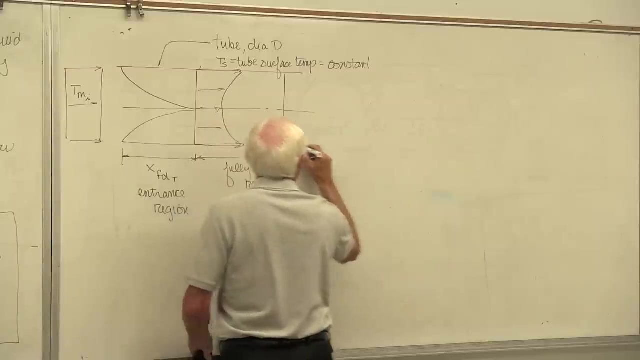 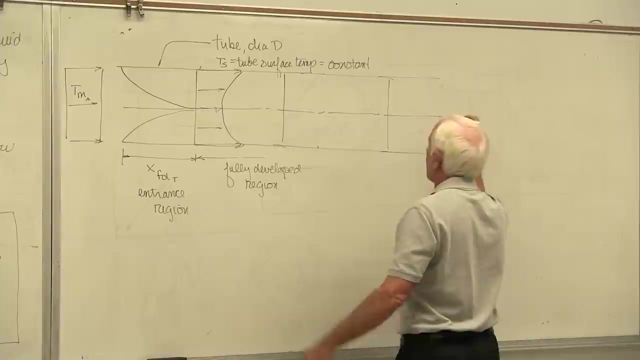 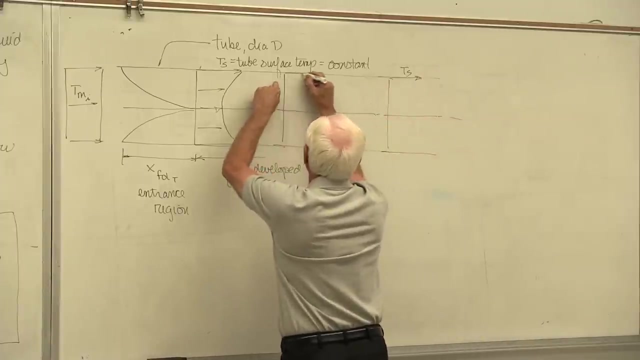 You're heating the fluid, So here's the temperature profile, Just like that. You go down a ways. The two surface temperatures are constant, constant, constant. Go down a ways, constant, constant, constant. Ts here, Ts here, constant. 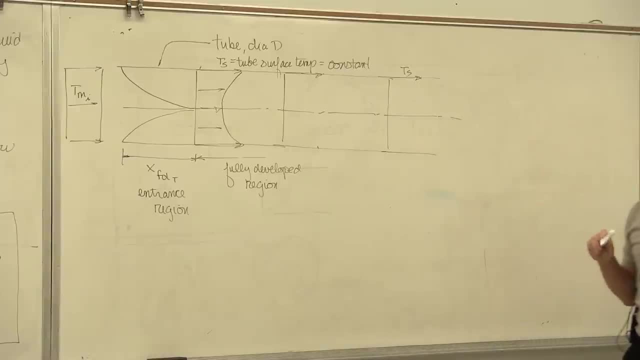 Constant, constant, constant. The fluid in the tube starts to get hotter- You're heating it. comes in cold Tube surface temperature hot: You're heating the fluid. This is how it looks. Go down a ways further. This is how it looks. 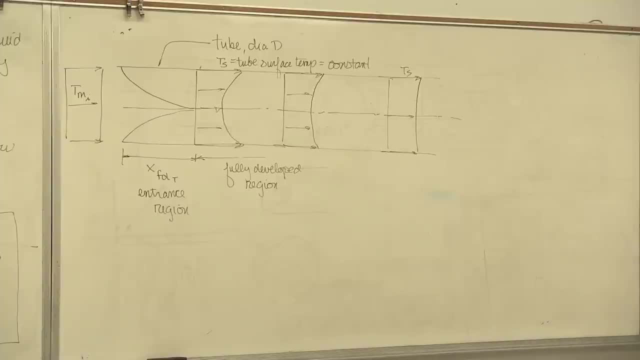 Oh, you can see how it's changing. It's getting flatter and flatter the middle. All the fluid in there is approaching the tube surface temperature, T-S. All the fluid temperature is approaching T-S. if you go down far enough, That's the fully developed. 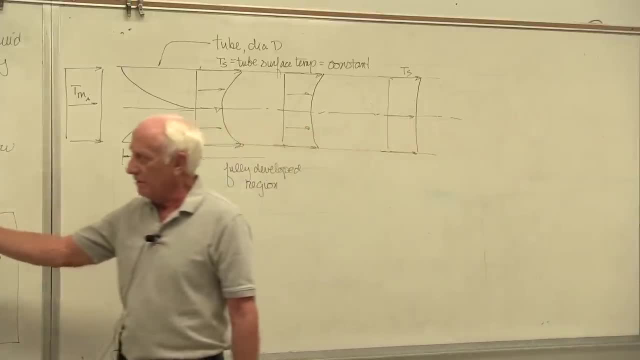 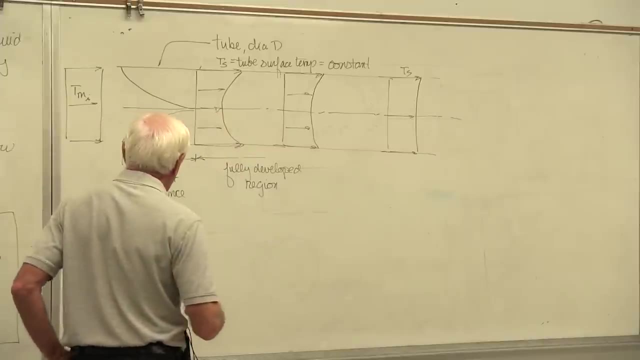 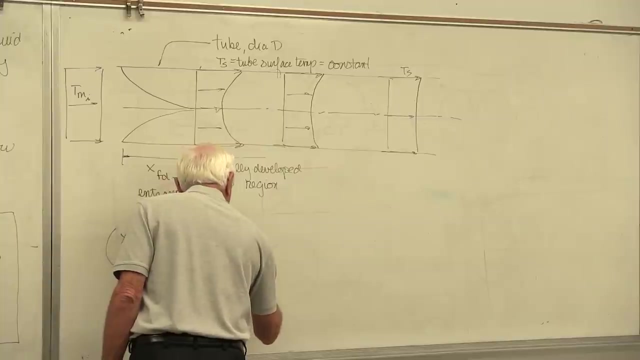 region for temperature. Here's the fully developed region for velocity. Okay, here we go again. How do we find this? X fully developed temperature. Okay, X fully developed temperature for laminar flow, for turbulent flow, same as velocity 10 to the power of T. 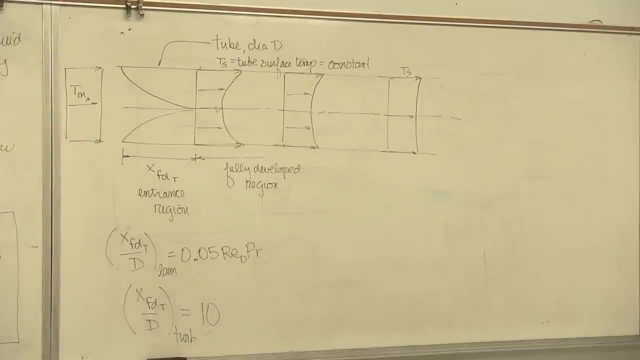 10 diameters. Turbulent flow is so mixed up that it doesn't change between these two pictures, But laminar flow or but the X fully developed laminar flow does vary. All you do is you tag on a Prandtl number after the Reynolds number here. We did that in Chapter. 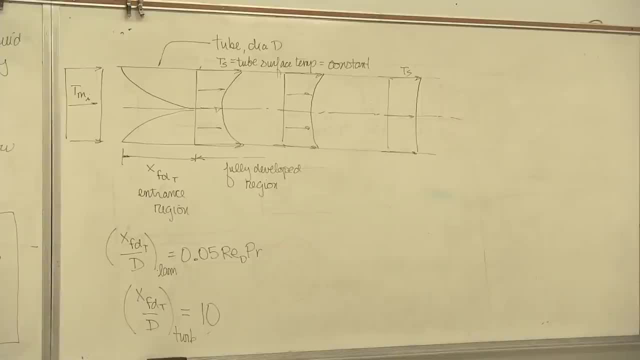 7. A lot of our equations- Chapter 7, had the Prandtl number tagged on to the right-hand side of the equation. It's characteristic of Prandtl numbers. It's characteristic of thermal analysis. Okay, let's box these guys in, All right. so now? 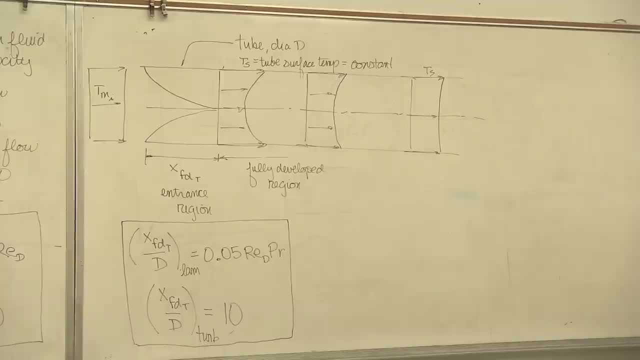 we have that. There's several objectives of looking at a tube like this. Number one is: you'd like to find the 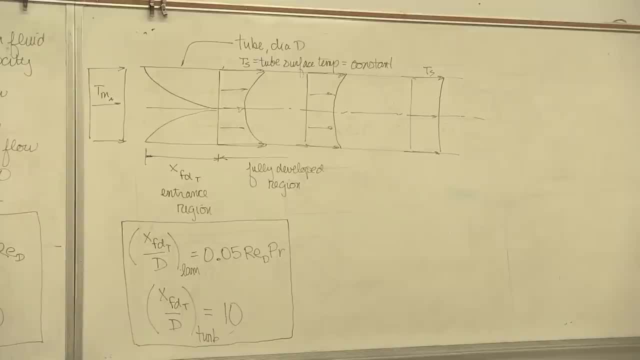 temperature at any distance along the tube. obviously, Find the temperature of the fluid anywhere down the tube. Number two: you want to find the heat transfer. Yeah, that's heat transfer, ME 415,. find the heat transfer. And you probably want to find H, because H 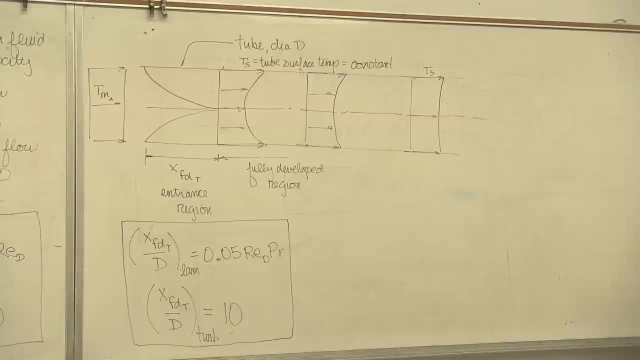 is important: convection, heat transfer coefficient- Probably three things you want to look at. How do I find the temperature as a function of X, Okay. How do I find the heat that's been transferred to the fluid from the tube? And then, how do I find the convection coefficient, H- Okay, All right, now this is constant tube. 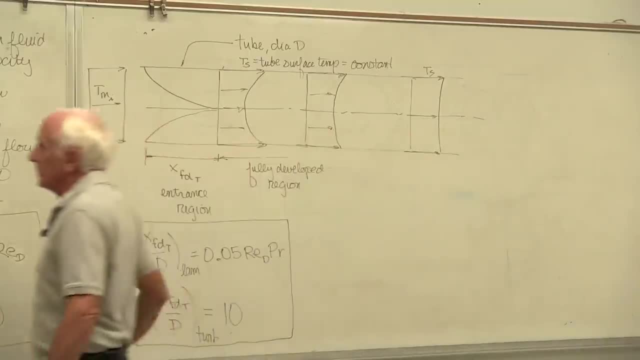 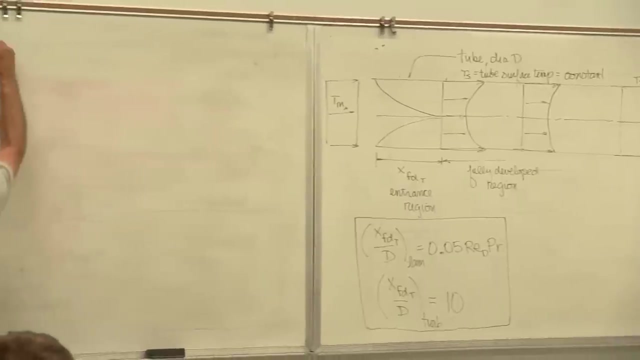 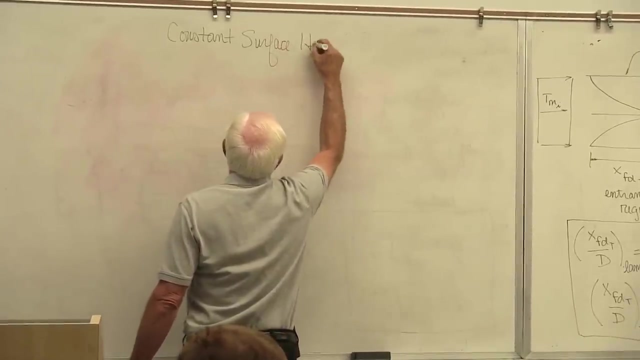 surface temperature. I'm going to start over here now. There's different kinds of boundary conditions on the tube surface. Number one is you can have constant tube surface temperature. Number two is you can have constant surface heat flux. So this will be constant surface heat flux, QS double prime. 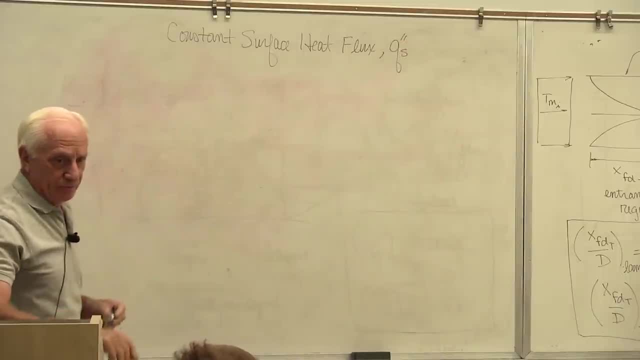 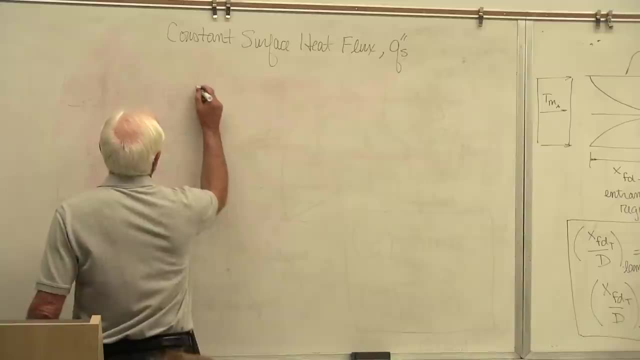 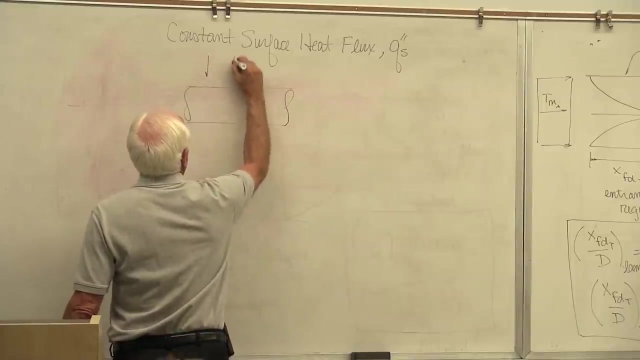 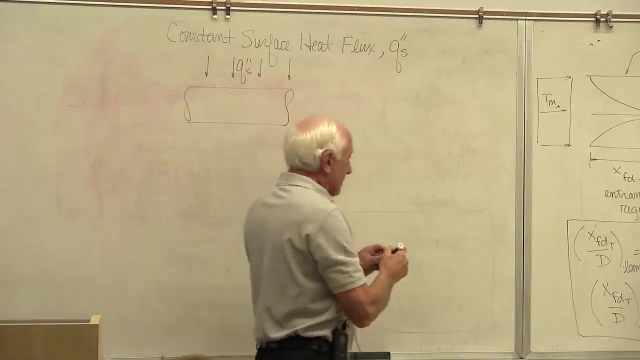 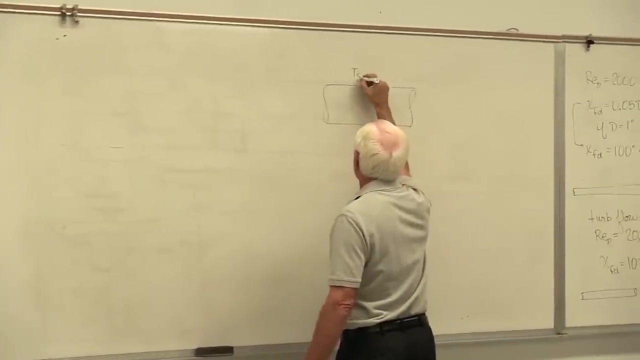 Double prime means watts per square meter, S means on the surface. Okay, so in this particular tube case you have a constant QS double prime. In that case you have a constant surface temperature. So that picture I'll put over here looks like this: No matter. 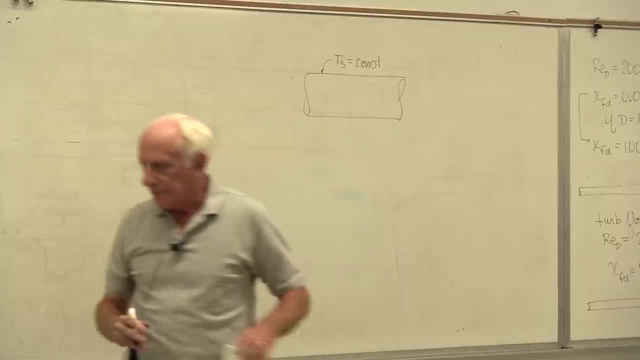 what the X value is. it's the same surface temperature. This is. these are the two cases that our textbook looks at. There are other cases, more complicated cases, and so on and so forth. These are the two simplest cases. These are: 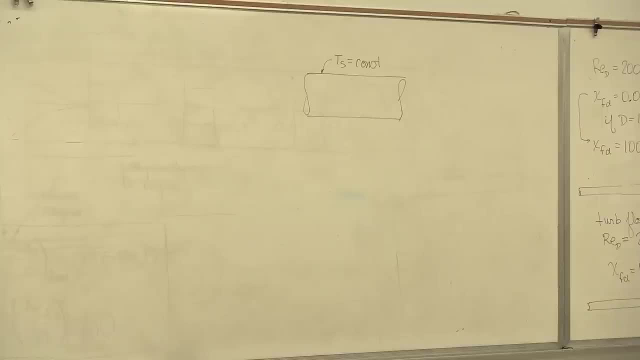 the two cases we focus on in Chapter 8.. Do they occur in the real world? Yeah, They're out there. Let's take one at a time. Let's take the constant surface heat flux. Let's get to it. Constant surface heat flux- this is a tube carrying water, for instance. I take a little. 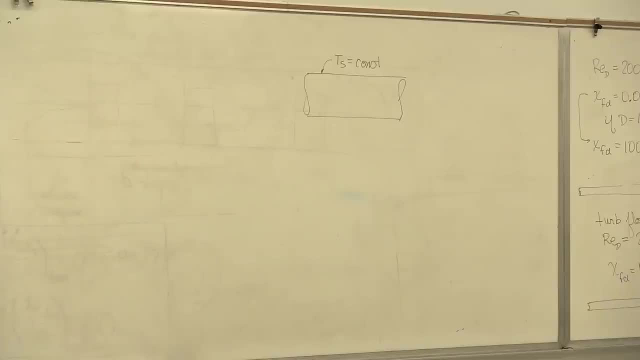 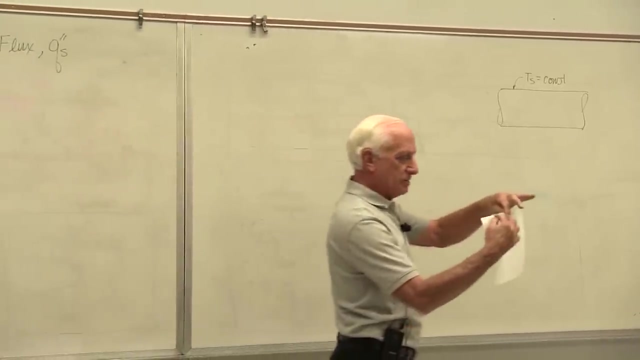 electric heating sheet. you can buy them. They have little resistance wires in them. back and forth, like your toaster inside, plus and minus plugged into the wall, The thing heats up. It puts out so many watts per square inch, square centimeter. So this is a little. 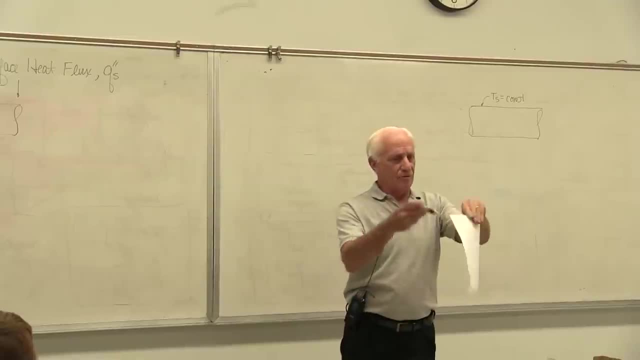 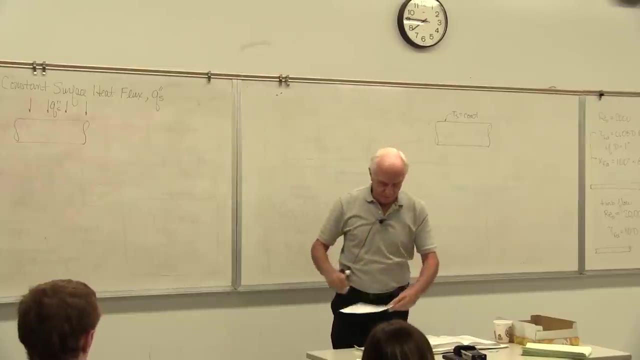 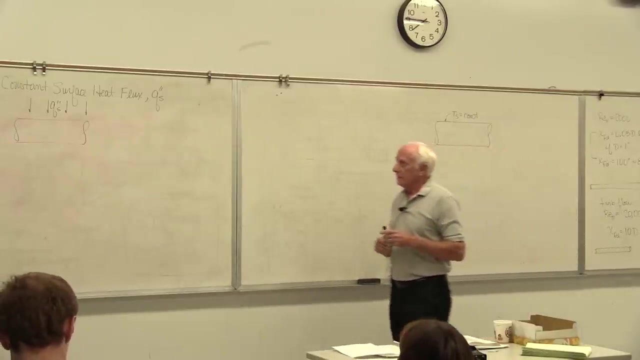 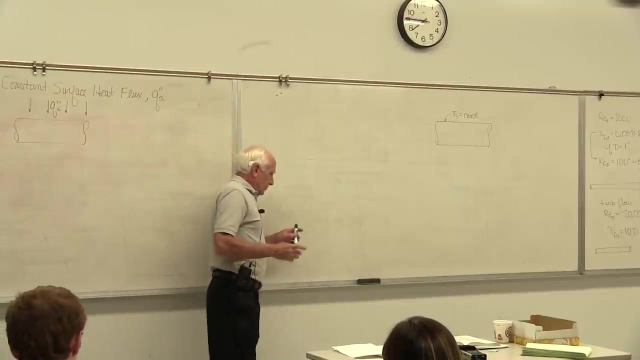 I take this little blanket, I wrap it around the tube and now I've got constant surface heat flux. That's one way. okay, It's not quite the same, but in a boiler you have these tubes carrying water and they're. 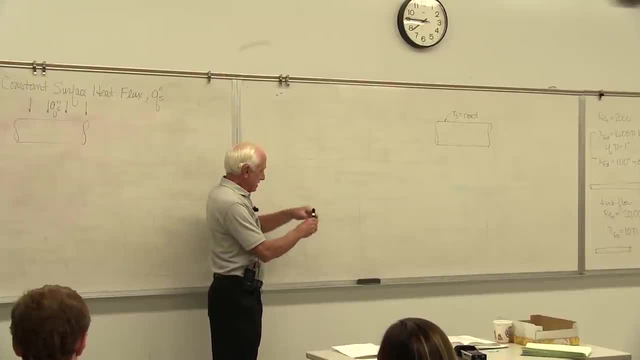 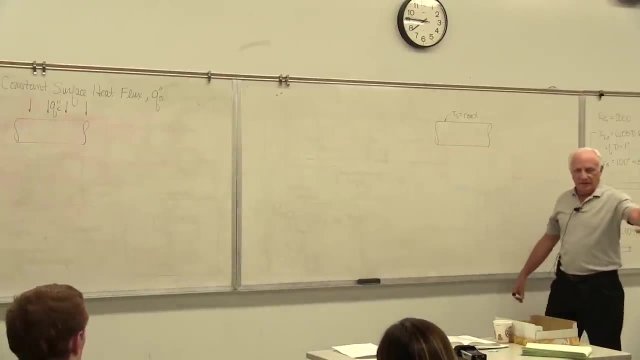 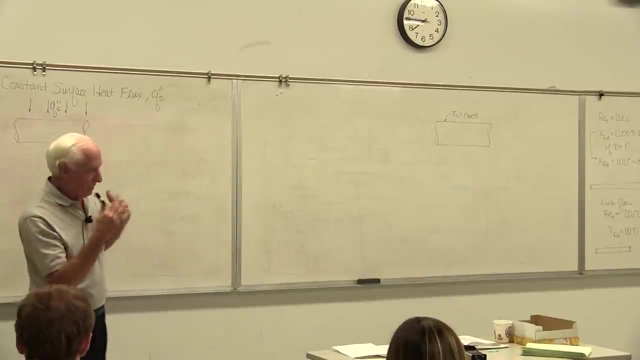 vertical on the walls and the wall's adiabatic. it's insulated and the tubes go up the wall, hundreds of tubes. There's a big flame out here. you're burning natural gas. That natural gas provides a flame. it's radiation and part convection, but it's so many watts. 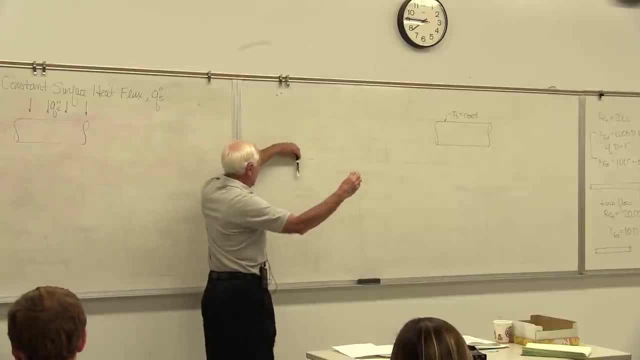 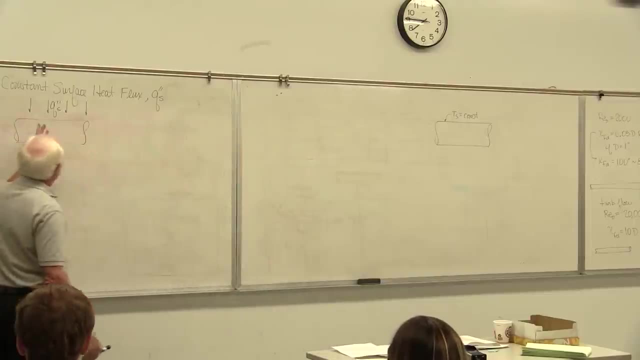 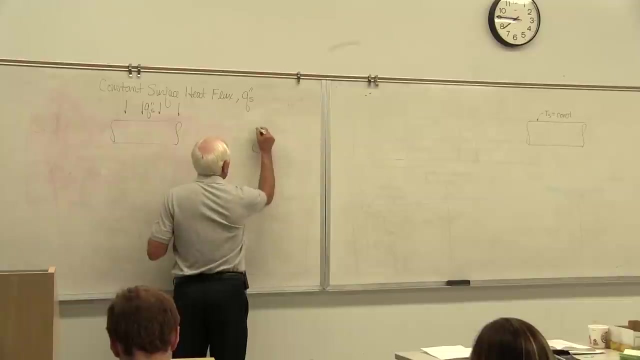 per square meter. well, that radiation hits those tubes, but just the front side in a case like that. so it's a modification of that. But that's how you get constant surface heat flux. You know, you've got a solar collector, a parabolic trough, and the idea is: here comes 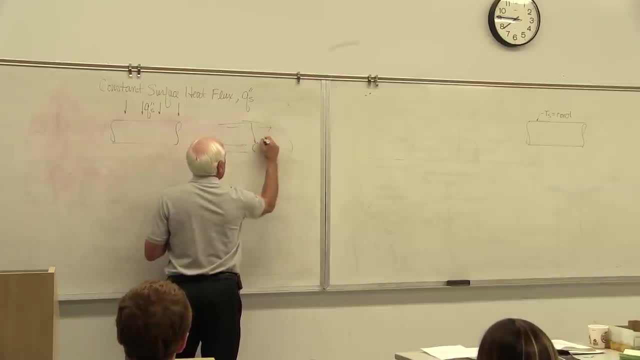 a solar radiation. it hits here, and it hits here, and it hits here. well, look at that, You're approaching this, you're approaching that. So yeah, it does occur in the real world. Okay, So this guy over here. where does this one occur? 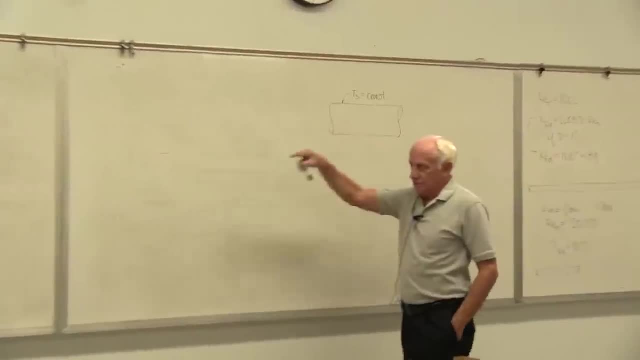 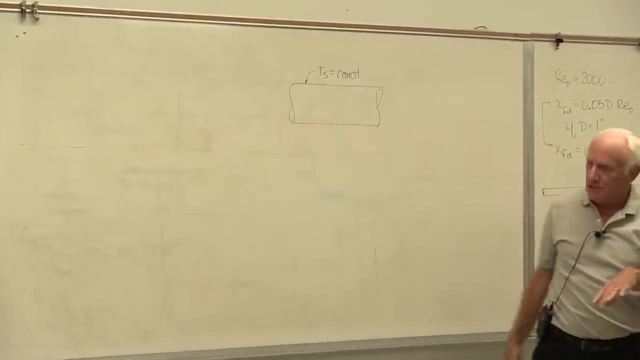 Well, this is in the condenser of the power plant. This was the boiler. I told you partially modeled that way, but now this is a condenser. You've got tubes in the condenser. this Redondo Beach power plant carrying Pacific Ocean. 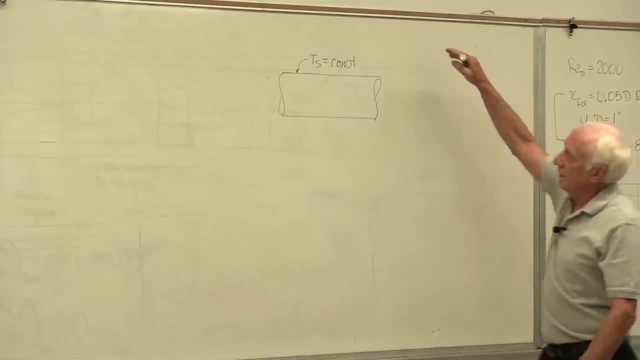 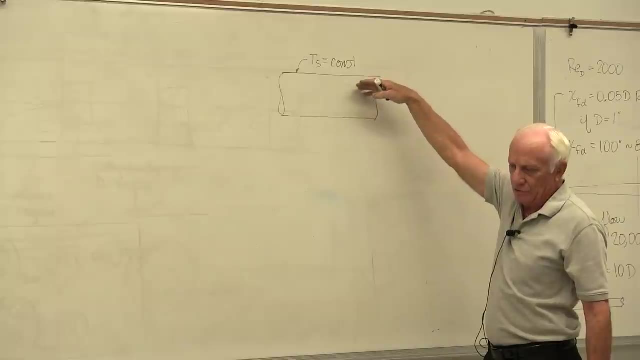 cold water in these tubes and then into this condenser comes the exhaust steam from the turbine And that steam, hot steam, sees the cold tubes. It condenses on the cold tubes. At what temperature? The saturation temperature, at the pressure in the condenser. 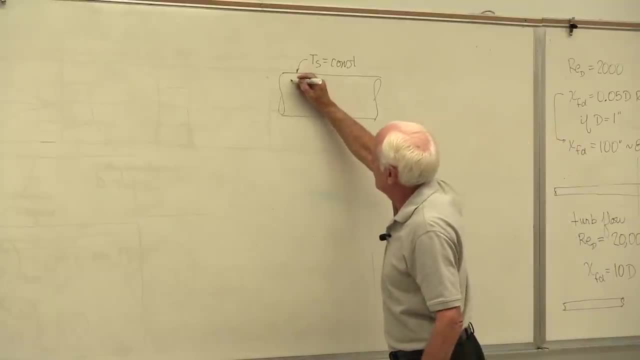 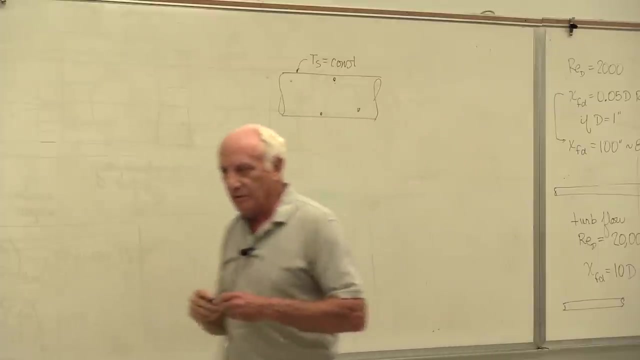 Okay, Every drop of steam that condenses, no matter where it condenses on that tube, condenses at what temperature? The saturation temperature, at the pressure in the condenser Right. Every one of these drops has the same temperature. so that's a good approximation for our T-S. 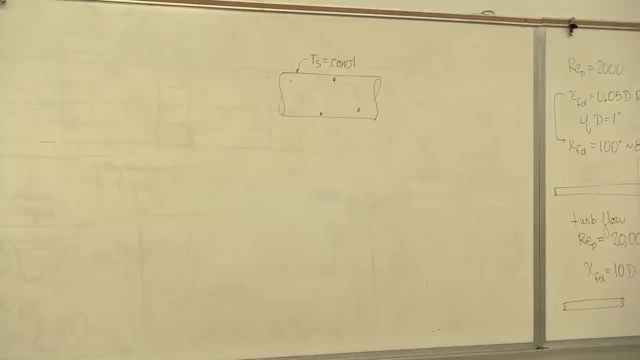 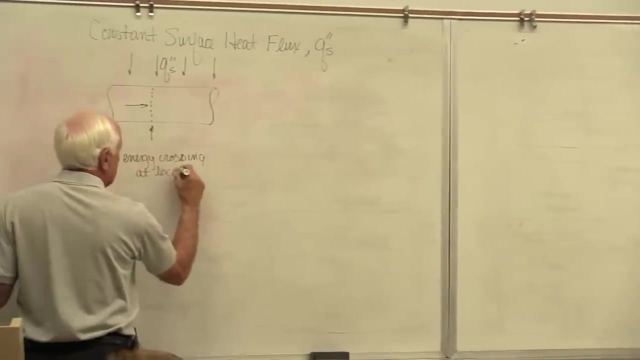 equal constant. Okay, That's just two examples of how these guys work. Okay, All right, Back to here. We want to ask the question first: how much energy crosses that line? So, at location X, how much energy crosses that line? 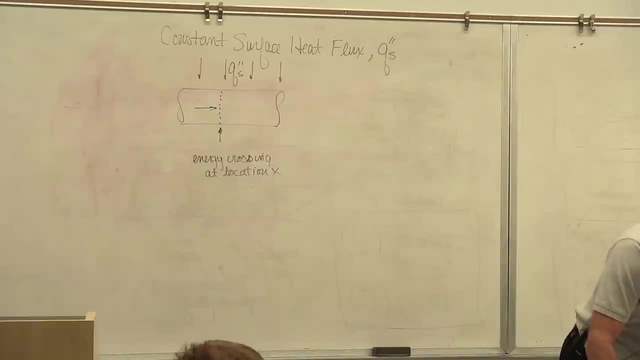 Okay, So to do that, we're going to go back to thermal, and that's equal to the integral over the cross-sectional area of the tube. rho U C, sub P, T dA. Here's where it came from. Okay, All right. 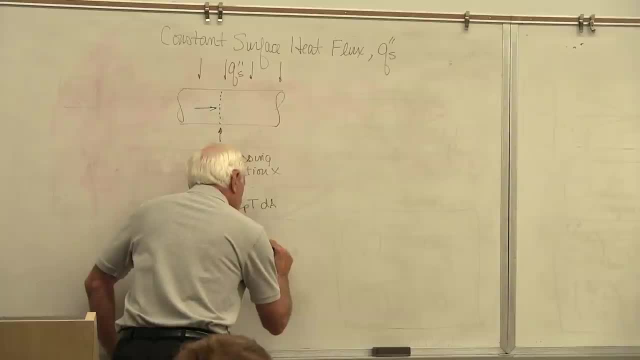 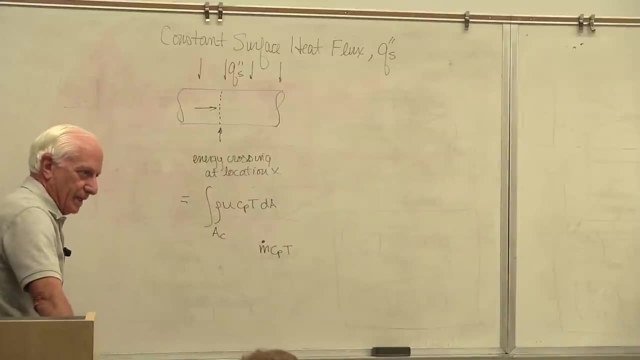 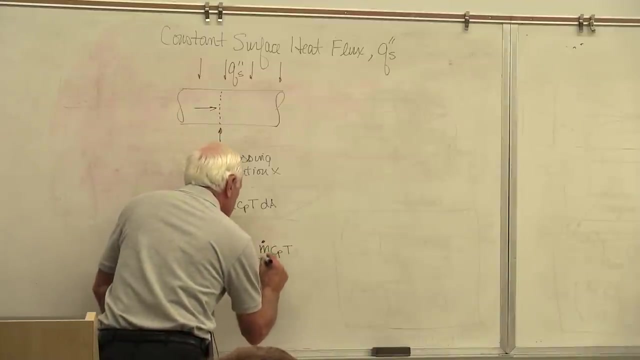 All right, So the energy being transported is m dot C sub P T. The C sub P sometimes stands for the enthalpy C sub P T. What's the mass flow rate? The mass flow rate is rho A- V. What's the velocity? 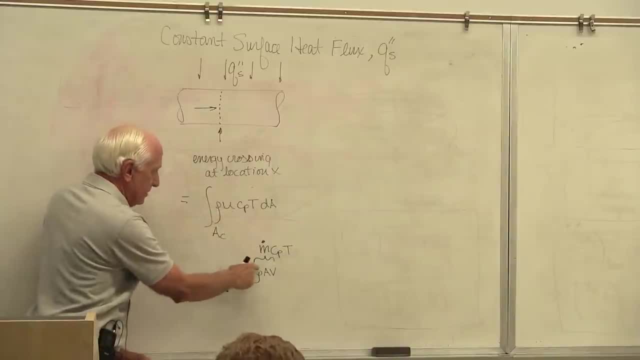 U. There's the density, rho. Where's the area? There it is dA. So this guy, this guy and this guy, all are m dot rho A V. That's the energy crossing the dashed line, All right. 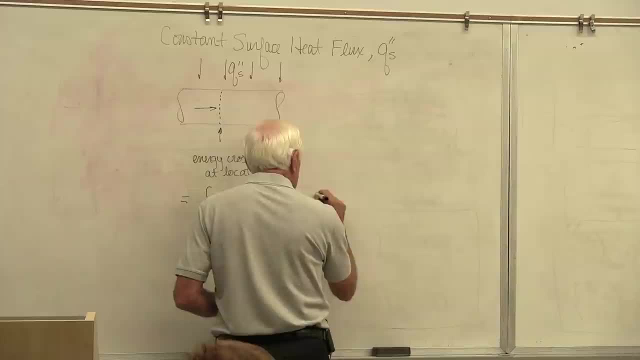 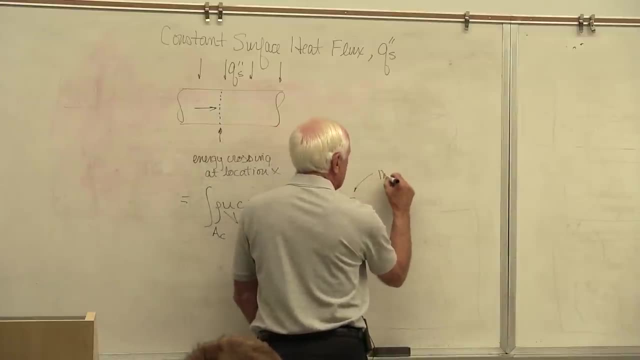 We define this as m dot C sub P, T mean. This defines T mean. So this equation defines T mean. Okay, All right, So that's WT. All right, T mean. So if you want to find the mean temperature of the fluid, what you do is you solve this. 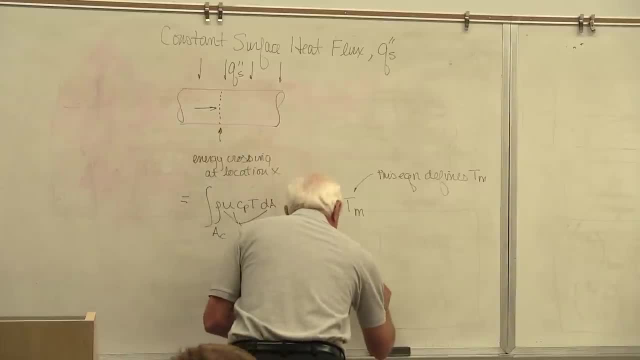 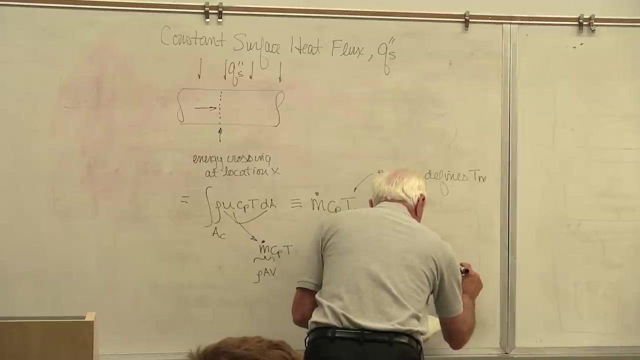 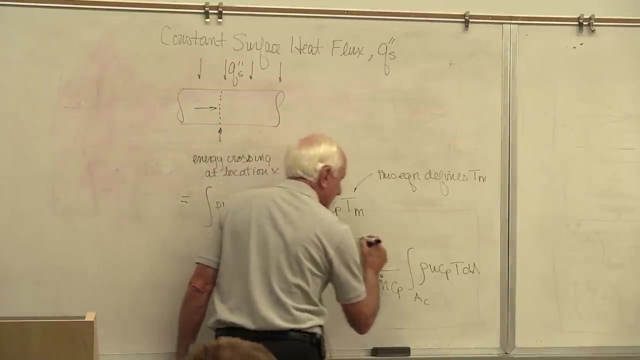 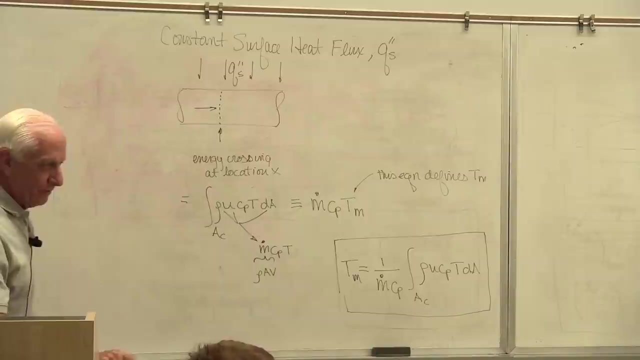 guy, T mean All right, All right. Okay, All right, All right, All right. If somebody says what's the mean fluid temperature, that's the official, integral way of finding the mean fluid temperature. But you've got to know how T varies with R. You've got to know how U varies with R. It's 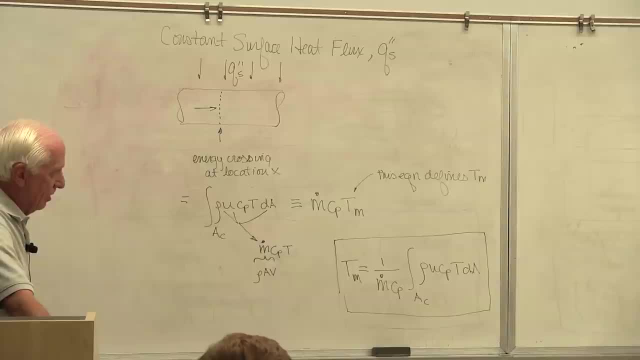 not easy. Both U and T vary with R And what's dA? dA is 2 pi R dr, The little donut-shaped area. 2 pi R dr is the differential area dA. Okay, So we did that in ME 311 for U, the average velocity, the mean velocity in a tube. 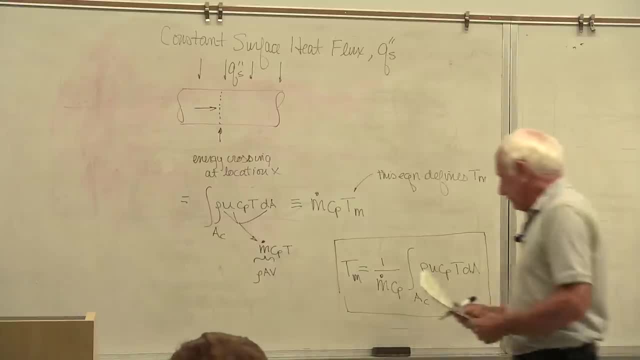 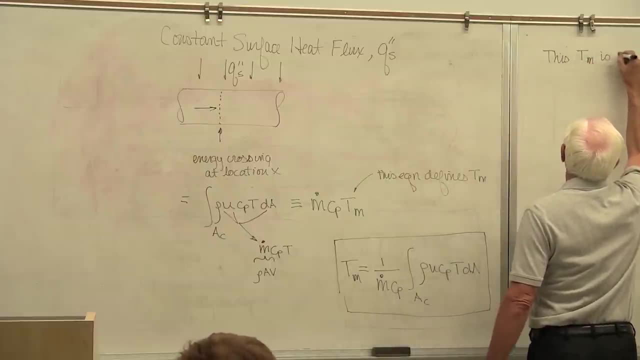 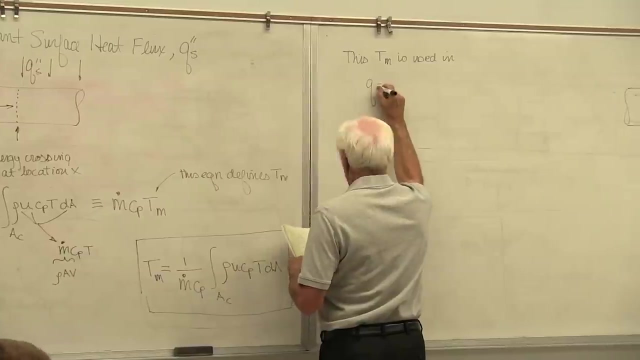 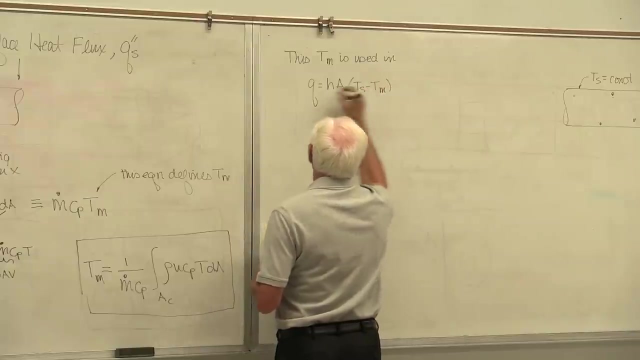 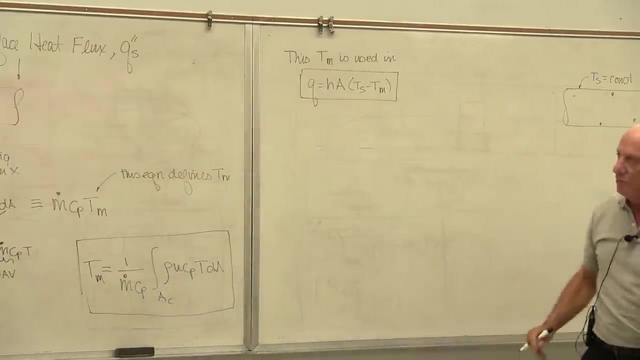 It's very similar. Okay, This Tm. why is Tm important? Well, this Tm is used in our Q. Okay, H A, T, S minus Tm. So that's Newton's law of cooling chapter one for a tube. 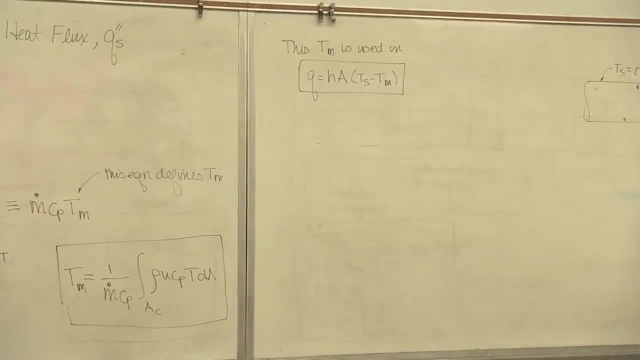 Chapter one: What's the right temperatures to use? The surface temperature, the surface temperature over here or over here doesn't matter. The surface temperature minus the mean fluid temperature. Okay, Now to see how that temperature varies. we take a little differential control volume. 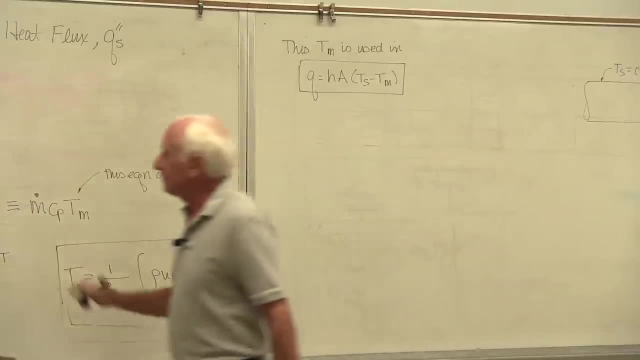 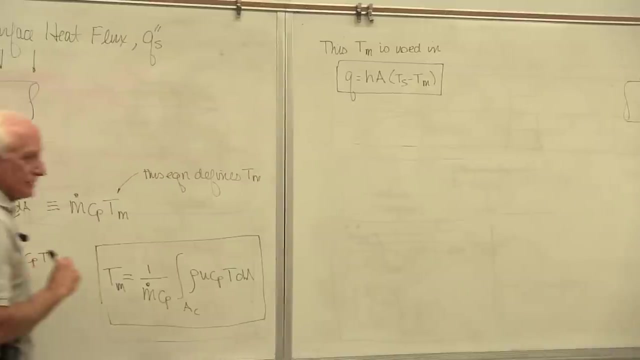 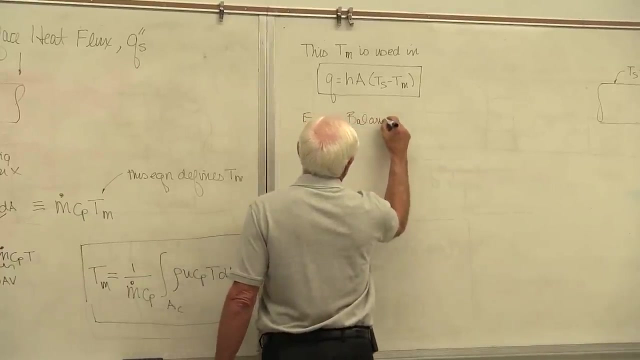 The distance is dx. Take a little differential control volume and run an energy balance on the little differential control volume. Okay, Here's the estaship. So the energy balance is supposed to be z. The energy balance is supposed to be g. 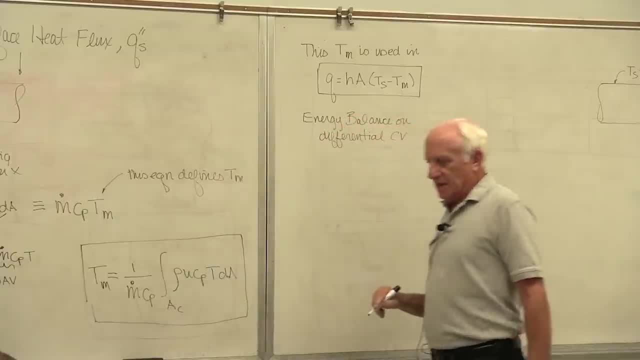 Okay, So the energy balance again for this guy. what does the energy balance says? Energy balance says: all the energy that comes into the fluid goes into raising its temperature. Okay, What energy comes into the fluid? Oh, there's a constant surface heat source. 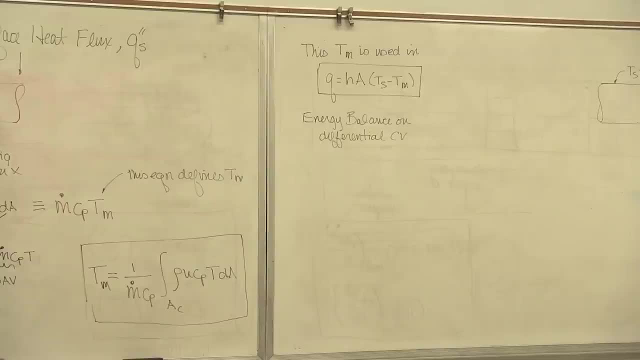 There, there. That's what comes in QS double prime That comes in multiplied by the area. okay, And what does it do? It goes into raising the temperature of the fluid. okay, So that's our M dot, C, sub P, DTM. All the energy that comes from the heat source goes into raising. 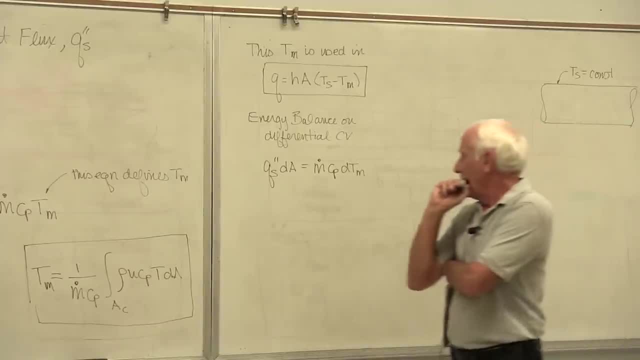 the temperature of the fluid. okay, What's DA? All right, DA, don't forget. This is the DA. is that lined area? It's a circle. Perimeter pi times D. Perimeter times DX. Perimeter times DX. 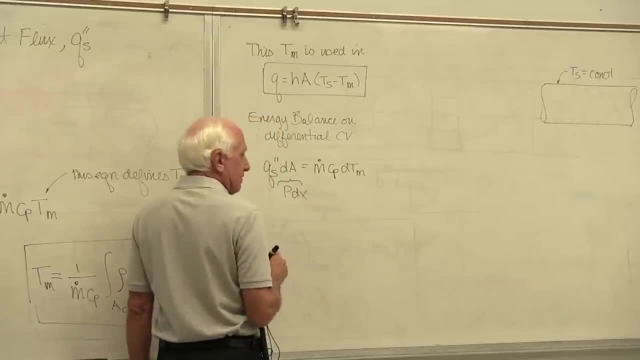 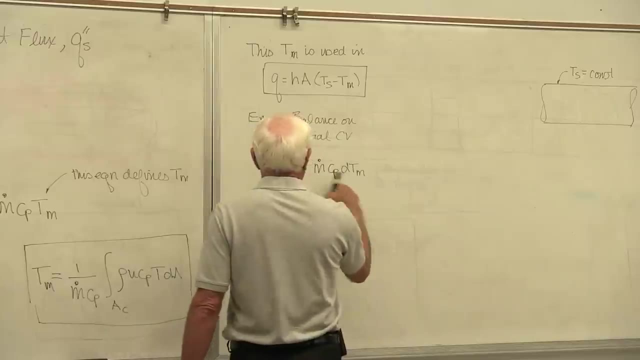 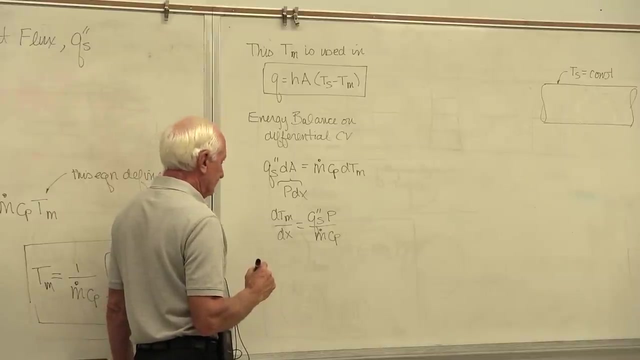 So DA is PDX. Separate the variables DTM, DX, DX. so this is QS, double prime times the perimeter divided by M, dot, C sub P. The right-hand side is a constant. okay, So integrate this guy to get. 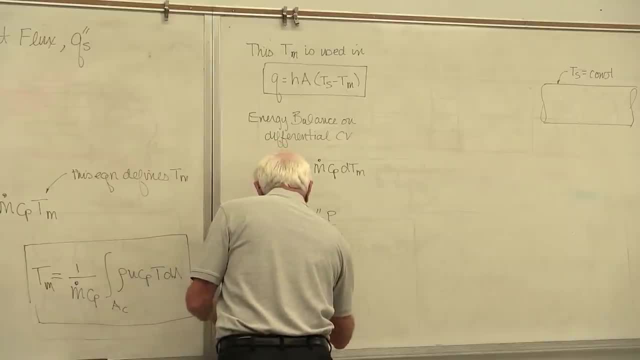 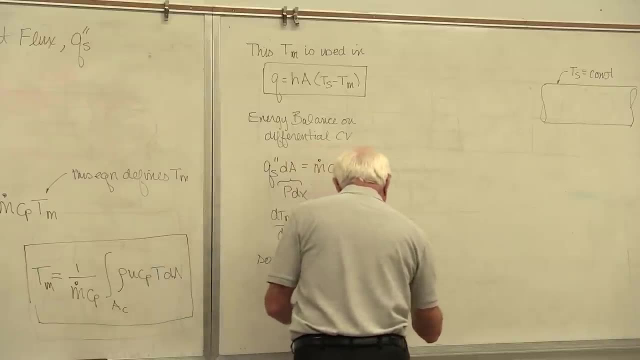 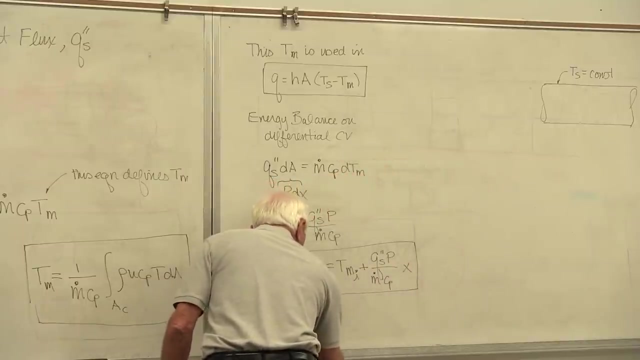 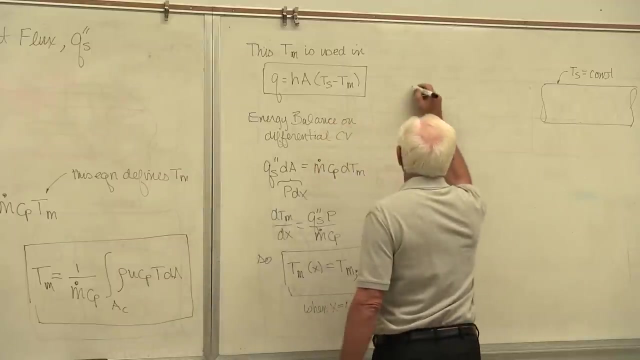 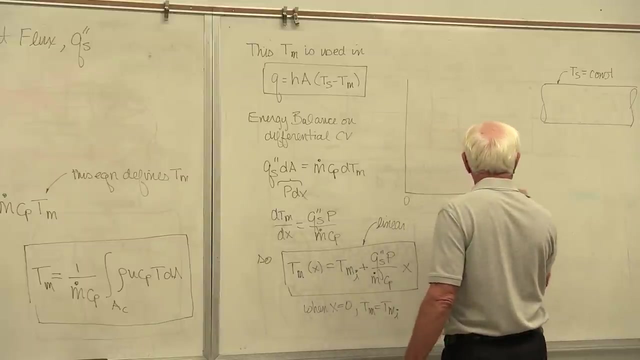 DTM as a function of X, DTM as a function of X And use the boundary condition When X equals zero, T mean equal, T mean. I Notice that that looks like a linear variation. So if I want to plot that, here's zero, here's x, and I'll just say this is the length of 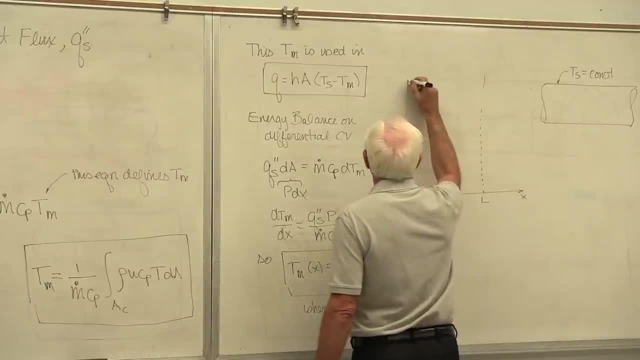 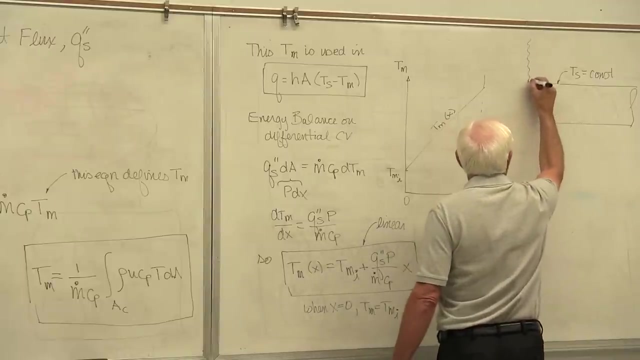 the plate L and this is the temperature of the fluid. T mean: It comes in at T mean, N. It's linear with x, it's a straight line. So here's T mean as a function of x. Now if I want to plot that, I'll just say zero, here's zero, here's x, and I'll just 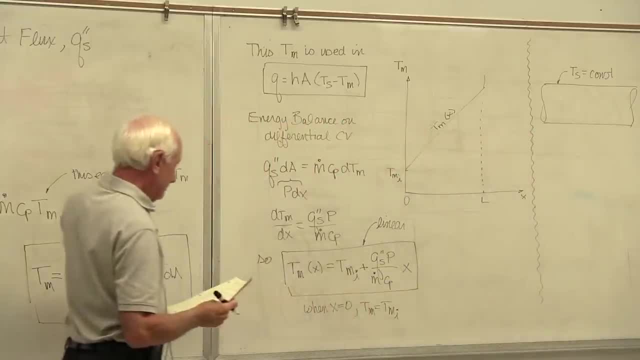 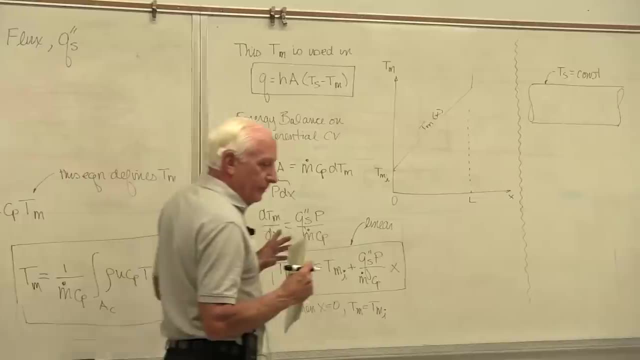 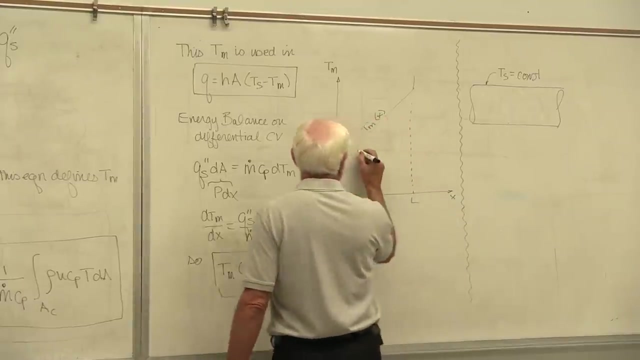 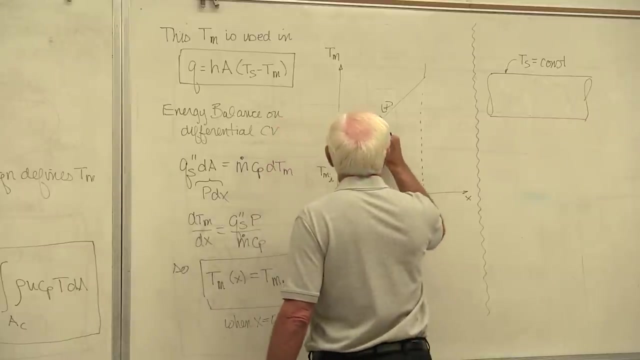 say, this is the length of the plate L And this is the temperature of the fluid T mean. Now we're not going to prove this now, but I'll just show you where the surface temperature goes. If this is x fully developed for temperature, then the surface temperature looks like this: 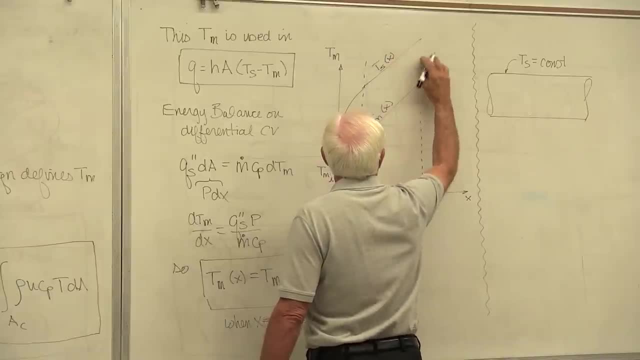 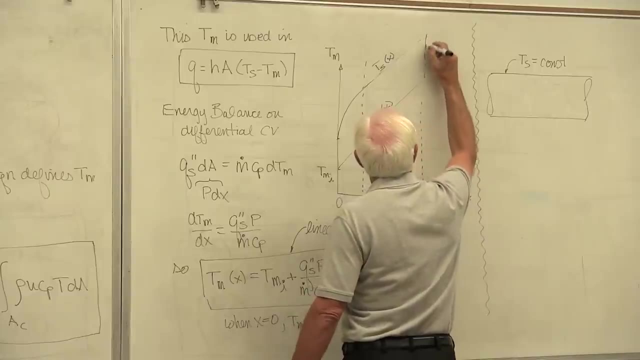 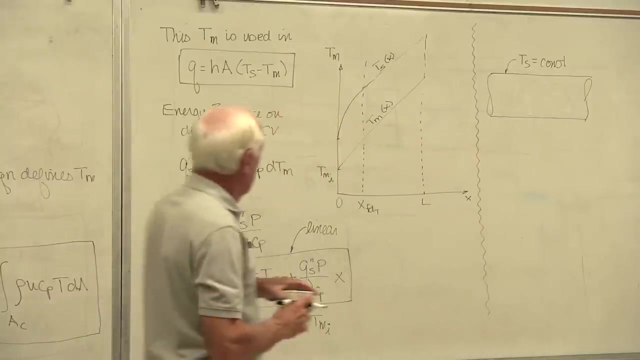 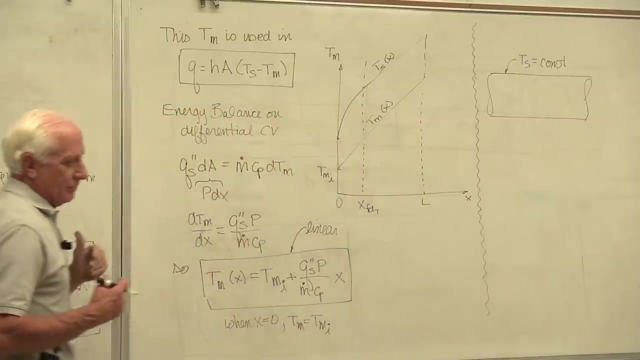 Okay, And the distance between these are the: these two lines have the same slope. They have the same slope, okay, But we're interested in the fluid temperature. So there's no equation for Ts. You won't have an equation for Ts, just I'm just showing you graphically what it what. 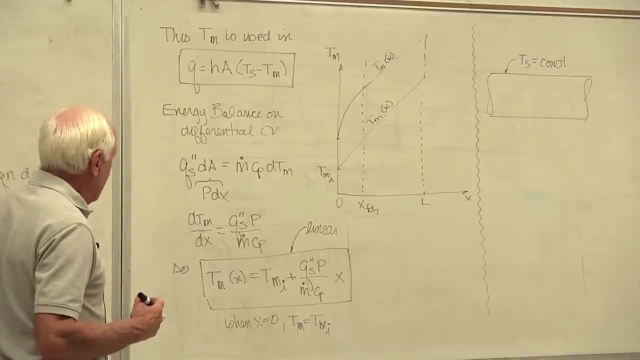 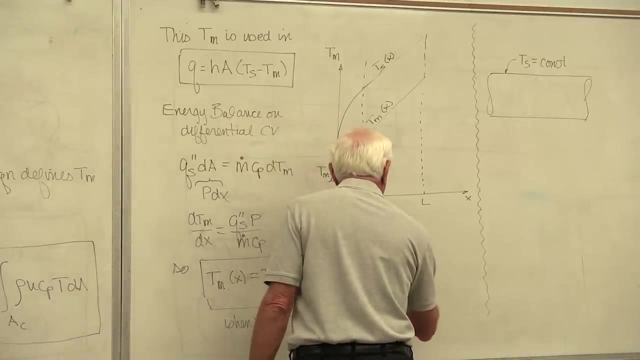 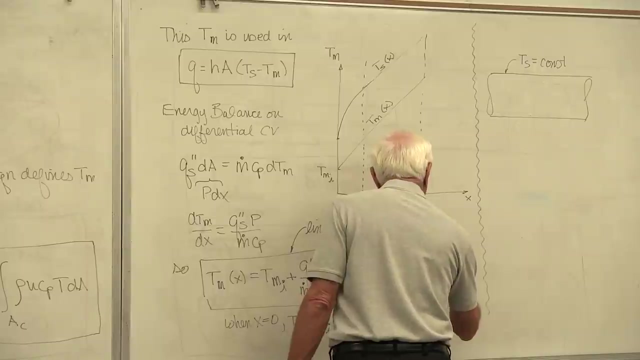 happens. Okay, Now I think that's well. yeah, okay, let's get, let's get Q. How do we find Q? Okay, Q, the heat transfer to the fluid: M dot, C, sub, P, T M out, minus T M in. 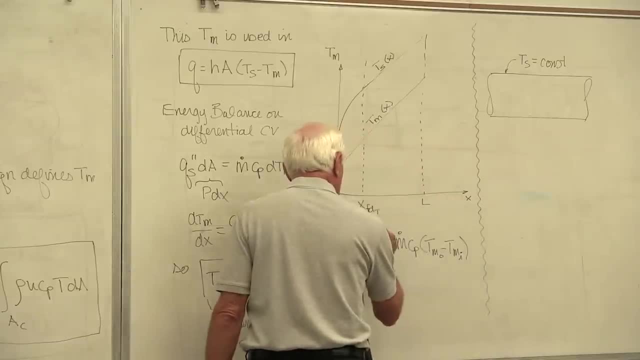 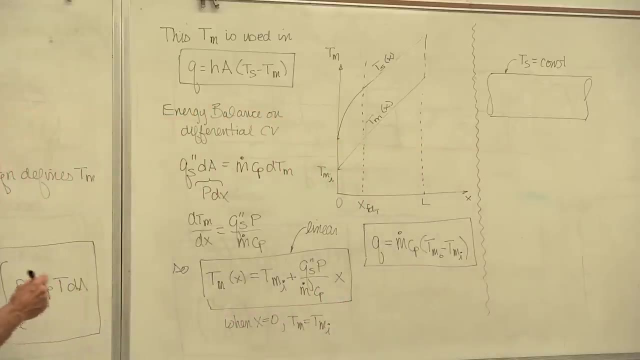 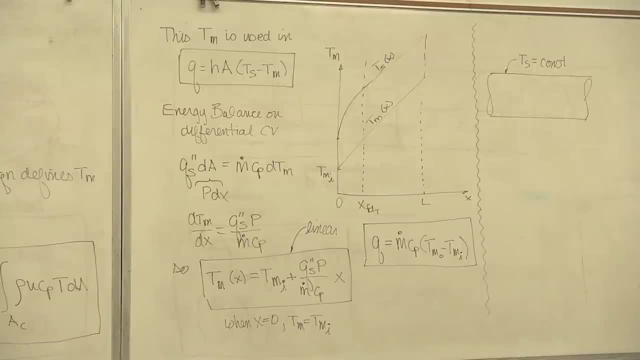 The other equation gives you how much heat has been transferred to the fluid. Okay, First you've got the real Christmas tree, And then you've got M dot X, And so whatぇ Now? second case: TS equal to constant. okay, We can do it somewhat the same way. Here's: 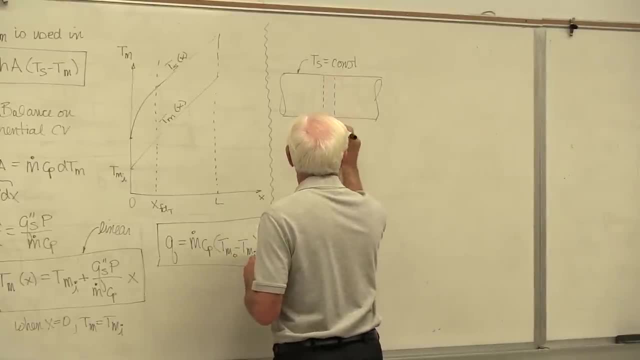 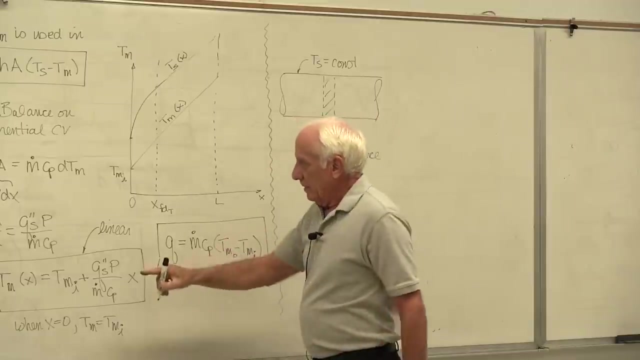 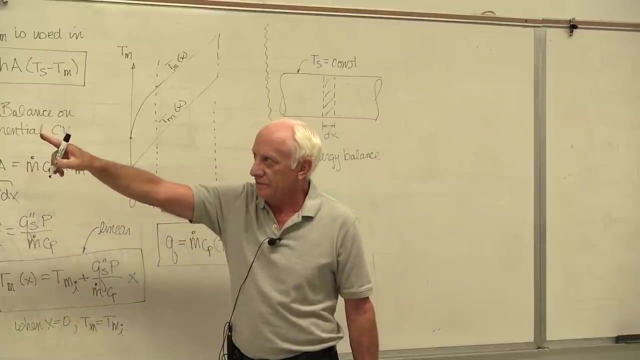 our little differential fluid element. The distance is DX. We run an energy balance on that little fluid element. Okay, here, right here, What comes into the fluid? Okay, It's not a constant surface heat flux, It's now a constant surface temperature, So it's convection. 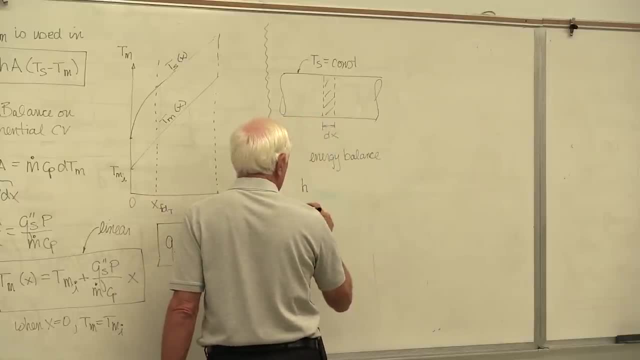 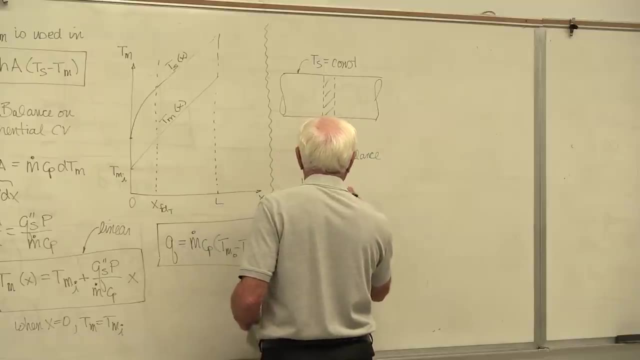 So what comes in is convection H- okay, times the differential area times TS minus H- Okay, Minus T- mean Differential area is perimeter times DX. This is convection in. And what does that energy do? It goes into increasing the temperature of the fluid, which is what 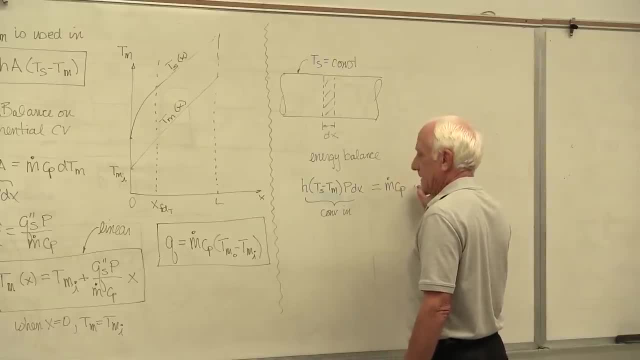 M dot C, sub P, DT or TM DTM. All right, Okay. So this is convection in. And what does that energy do? It goes into increasing the temperature of the fluid, which is what M dot C, sub P, DT or TM DTM. 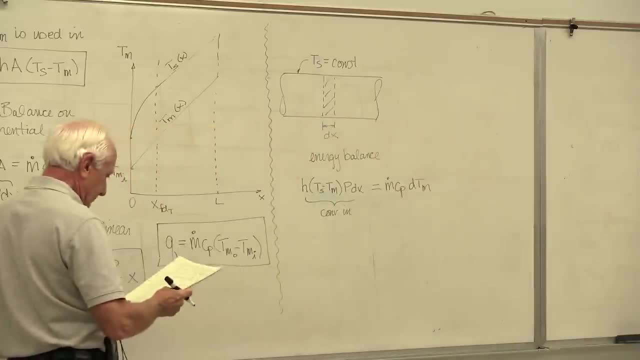 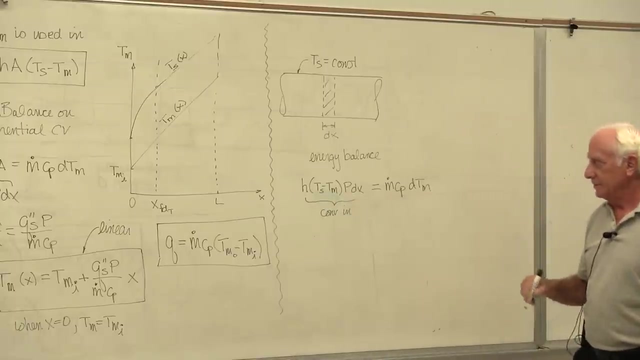 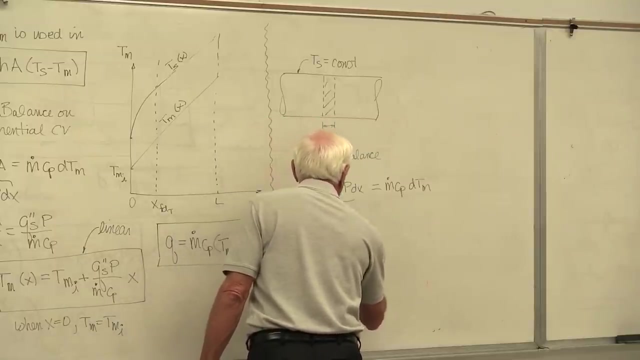 And now what you can do is you change variables, because that's TM and that's TS minus TM. So you change variables and you go ahead and solve this guy. It's going to be: you're going to have DTM minus T, Okay. 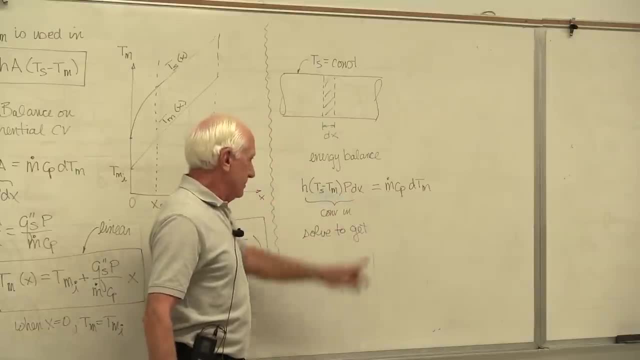 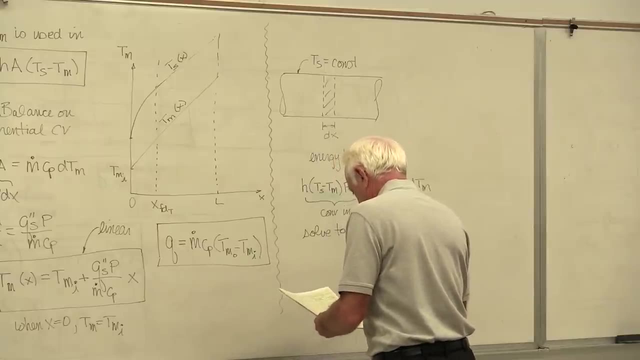 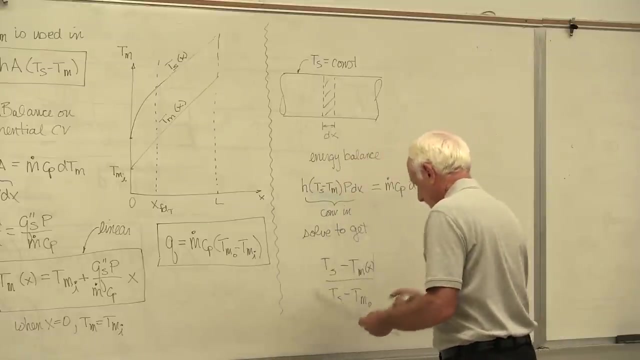 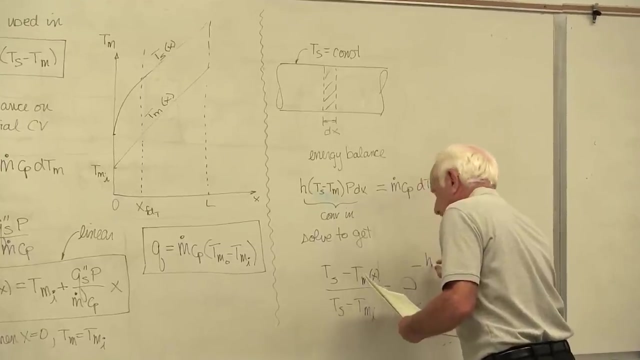 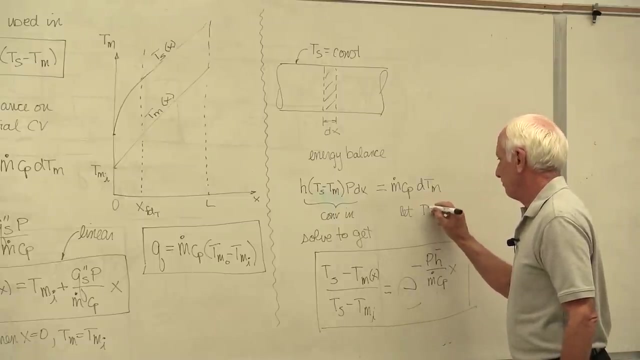 Okay, Okay, DT plus T DX. You're going to solve that. Okay, And you end up getting this equation And Thank you. You want to get these two guys to be the same, so you let TS minus TM equal delta T, So that's. 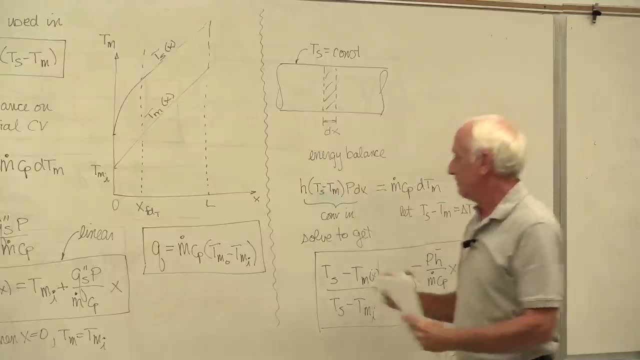 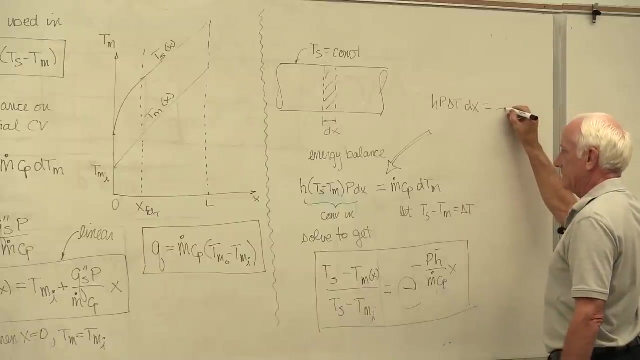 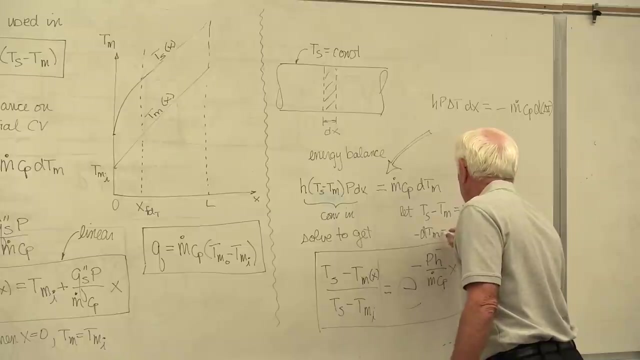 a delta T. there I'll show you. HP delta T. DX. equal minus M dot C. sub P D delta T. D TM. equal D delta T. Take the differential of both sides. Don't forget that the surface temperature is constant. The differential is zero Minus. 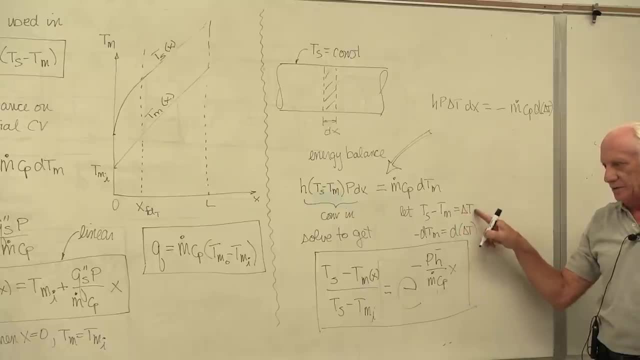 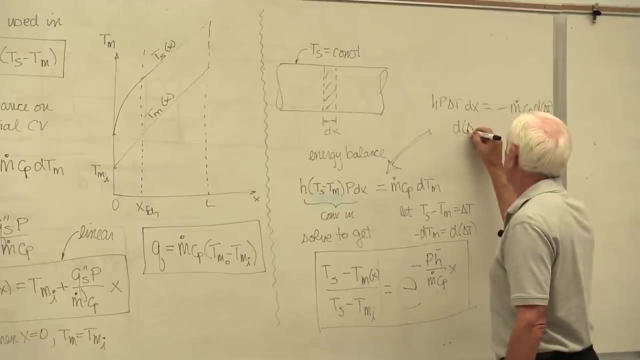 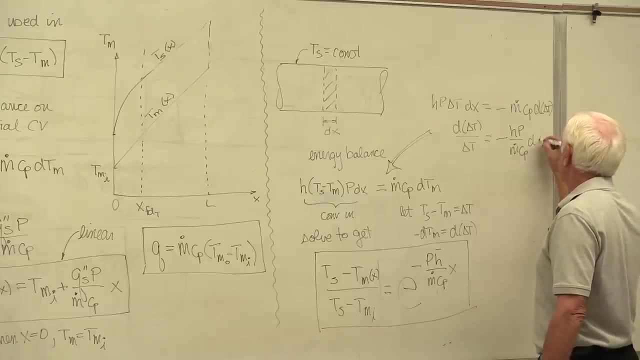 D TM equal D delta T. You want to separate these guys. D delta T over delta T is equal to minus sign HP over M dot C sub P D delta T. All right, Thank you. D delta T over delta T is equal to M dot C sub P DX. That's all the gory details Go. 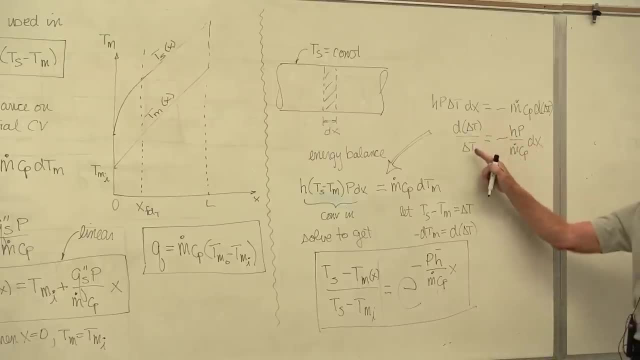 ahead and integrate both sides. Integrate DX over X. What do you get? Natural log. Take the inverse of natural log. What do you get? Exponential function? There's where it came from. Okay, What did we do? All we did was change the variable to make the differential. 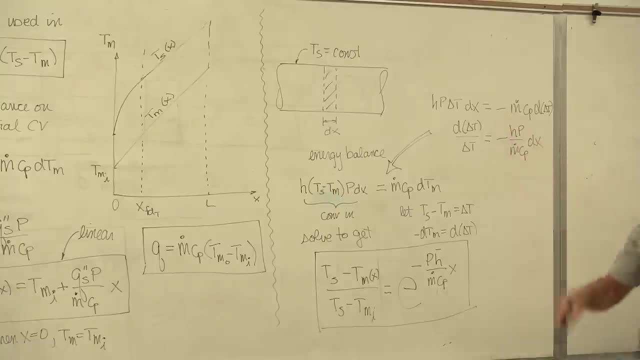 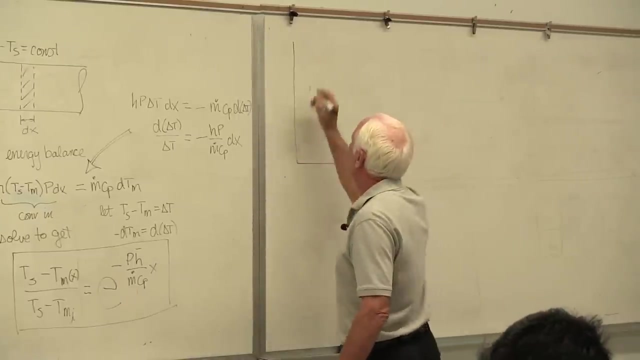 equation. look neater and cleaner There. Okay, Now let's go back to the differential equation. Let's look at that. All right, Now we're going to get Q, our Q. Let's draw the graph. first of all, This is the mean temperature of the fluid. This is X, The tube is L long. 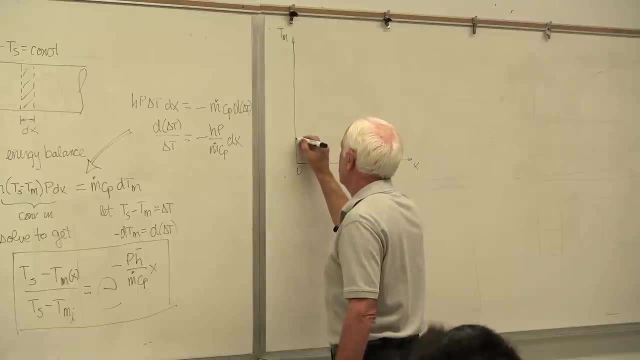 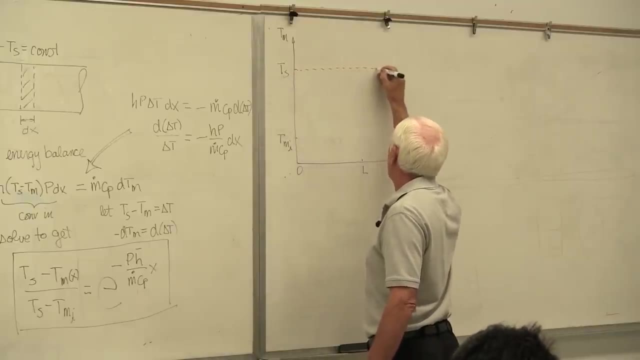 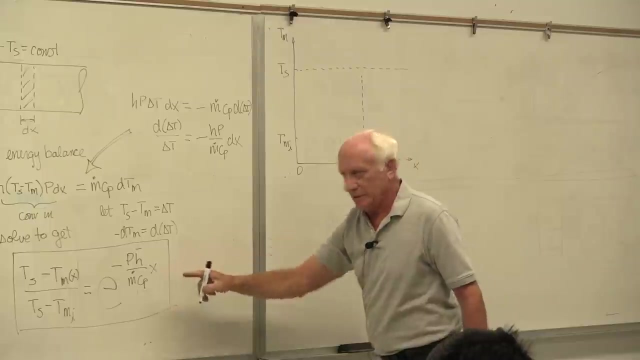 There's L, Here's zero. The stuff comes in. at T, mean N. The tube surface is kept constant. at TS It's kept constant. The fluid temperature increases exponentially. Exponential increase, Don't forget. Constant tube Heat flux. Linear variation of temperature. 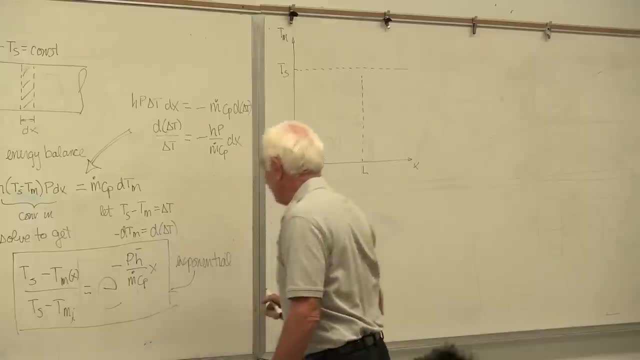 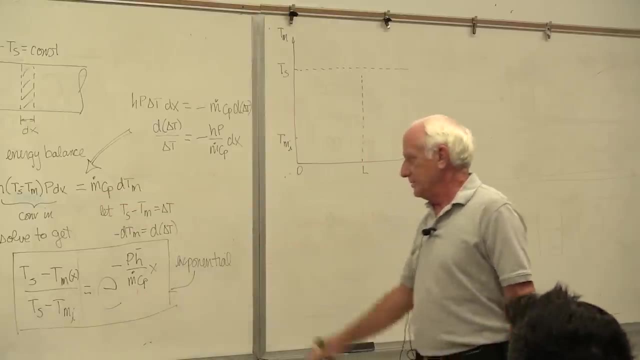 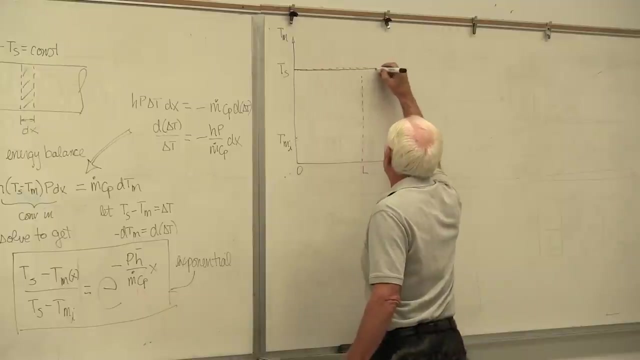 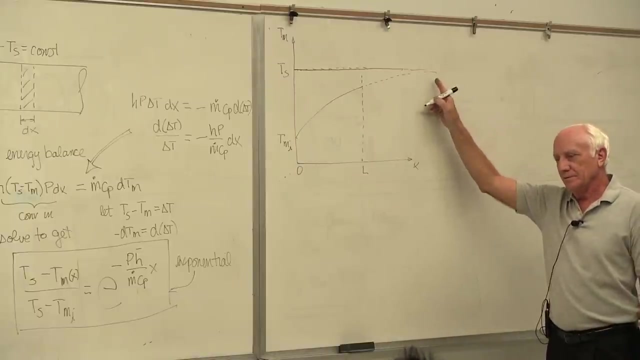 This one Exponential Here is the surface temperature of the tube. The stuff that comes in is cold, For instance. It heats up to something, to temperature E Dimensions've all gone to T and P heats up If it's long enough. if the tube's long enough, eventually the fluid in the tube 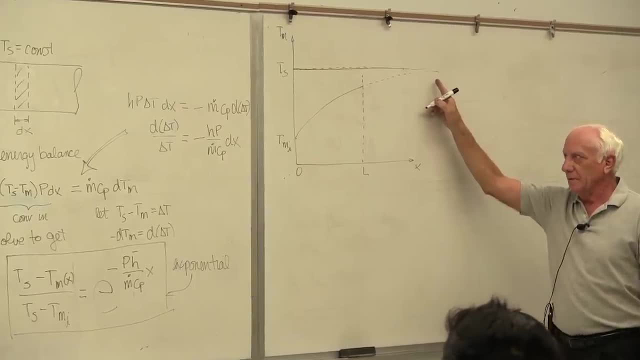 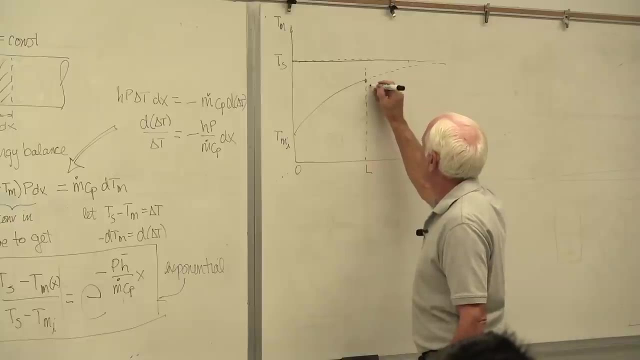 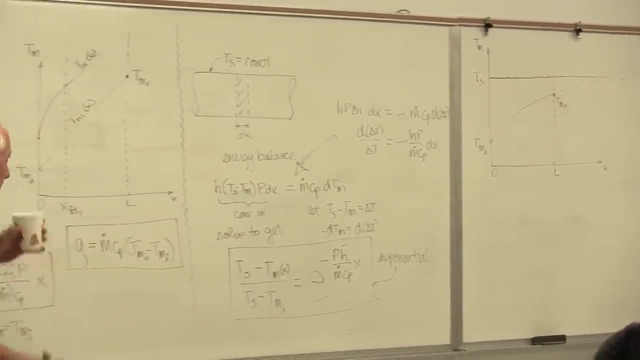 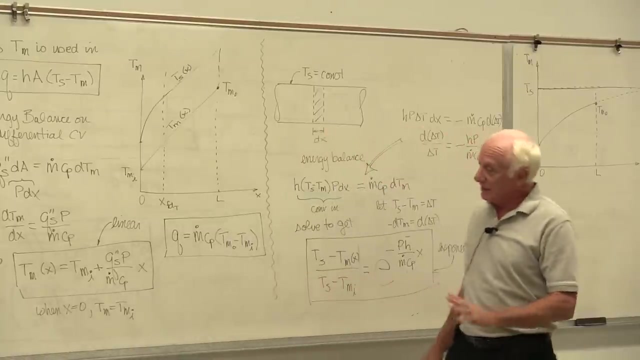 will get to the same temperature as the tube surface. If it's not that long, stop right here. It comes out at that temperature. That's T mean out. There's T mean out Over here. there's T mean out. Okay, Pretty different. I mean one is linear, The other one's exponential. 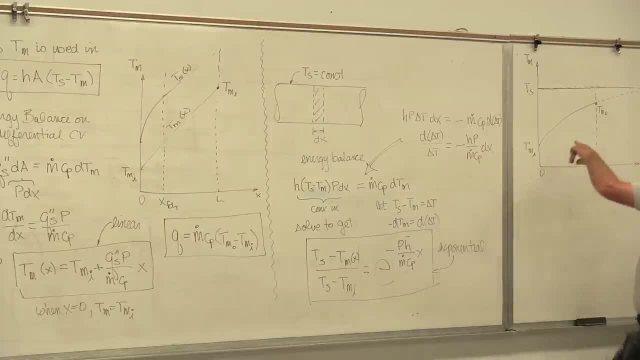 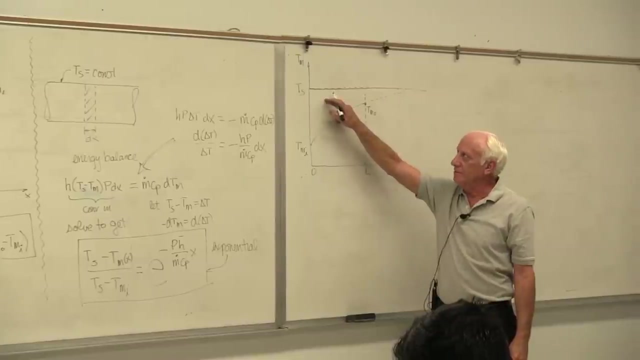 This is like: the tube surface temperature is constant. This is, like I said, a condenser. Do you have to worry about anything too much here? No, The hottest the fluid can get is the tube surface temperature. The hottest the fluid can get is the tube surface temperature Over here. oh, you better be careful This. 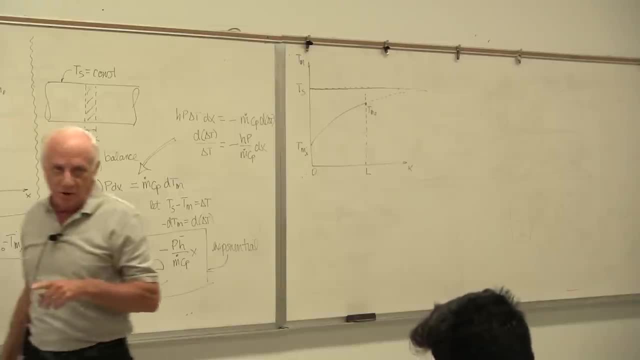 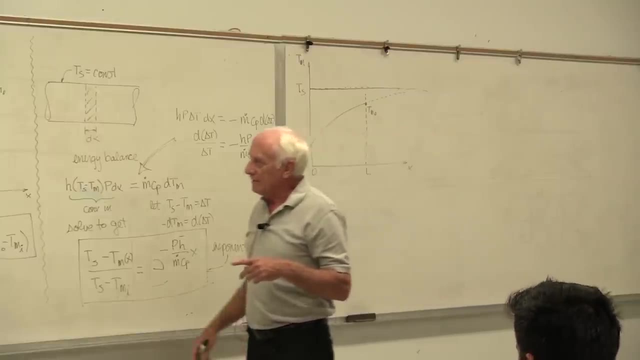 could be a boiler And maybe there'd be a tremendous boiler explosion because something bad happened. What can be bad? Well, maybe you're changing as this increases. Maybe you reach a point where you're going to get a lot of water. You're going to get a lot of. 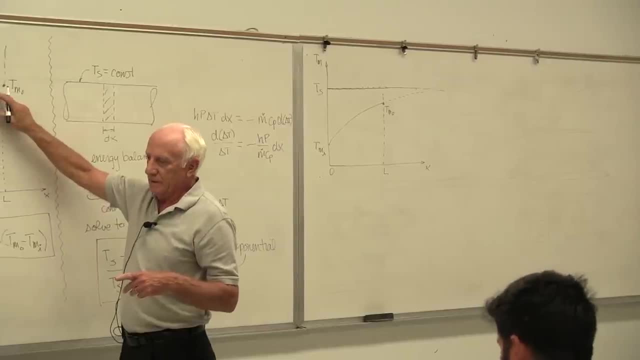 liquid, But you're not going to get a lot of water. You're going to have a lot of liquid, And maybe you're not going to get a lot of water. So you're going to go down to the point where the liquid water suddenly vaporizes and turns into superheated steam and gets. 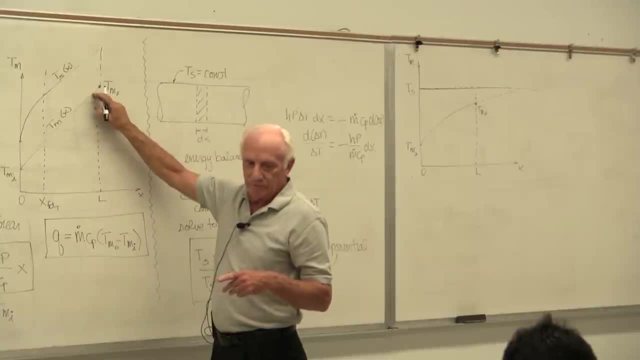 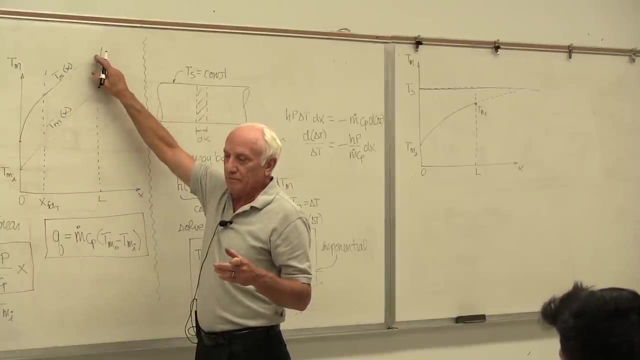 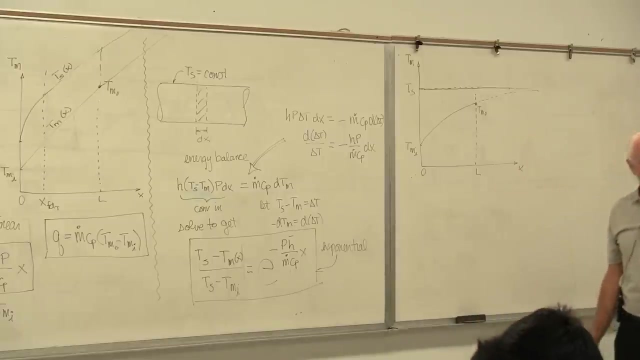 so hot, you have a boiler rupture, explosion, And also maybe the tube surface gets so hot, the material fails. tube rupture Because these guys, I'll tell you, these guys- never do stop. They don't approach anything asymptotically, They don't stop. Okay, You better be aware. 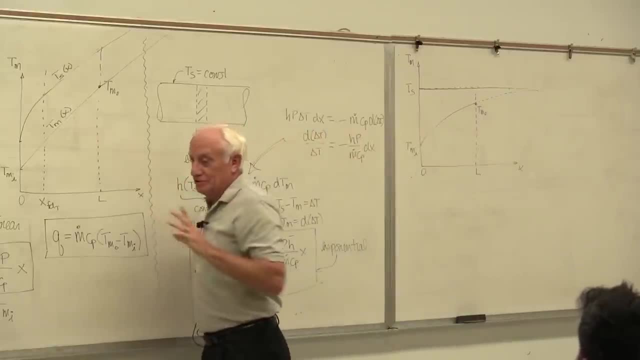 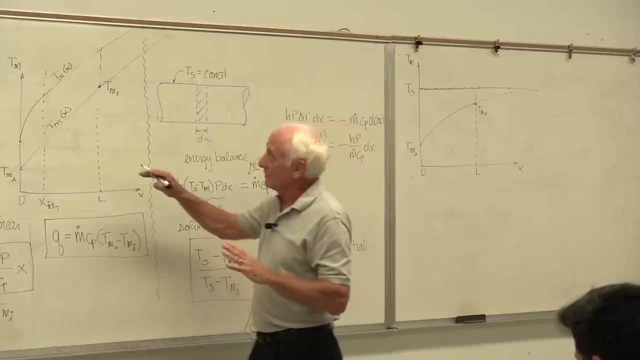 then This guy could be danger. But of course you do want to in a boiler, you do want to get superheated, you know. So it's good to a point, but you've got to be careful That tube surface temperature gets too hot and things could fail. 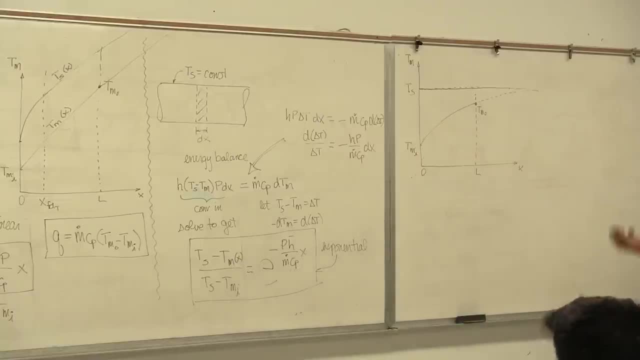 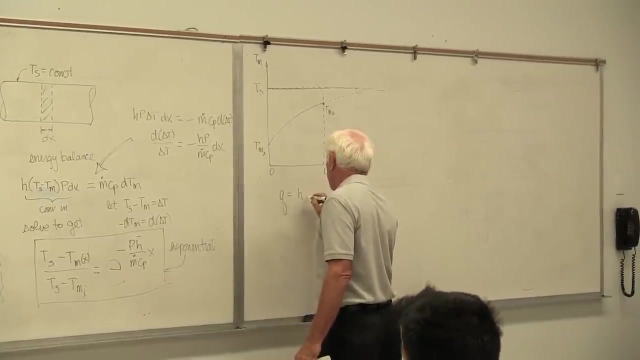 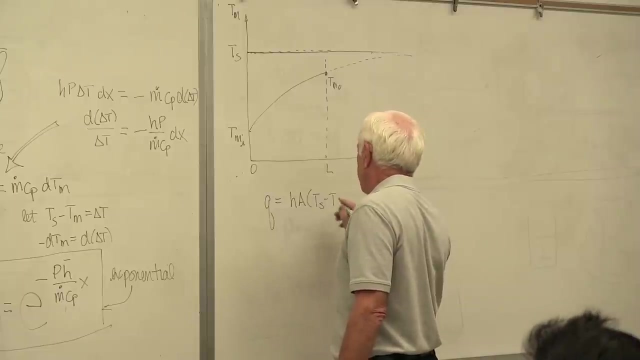 The tube could break open rupture. Okay, so again different things going on here. Now let's take a look at how we get Q over here. Okay, Q equal H, A, delta, T, T, S minus T mean. T surface is hot, T mean is cold. 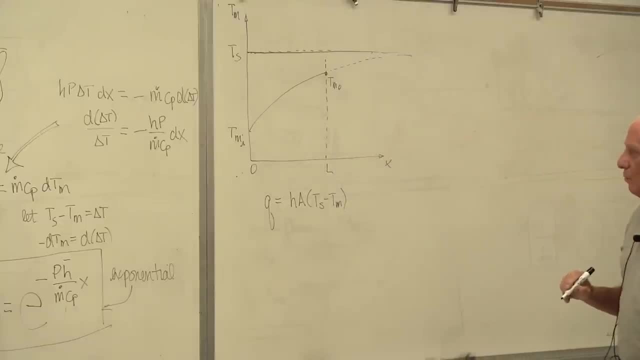 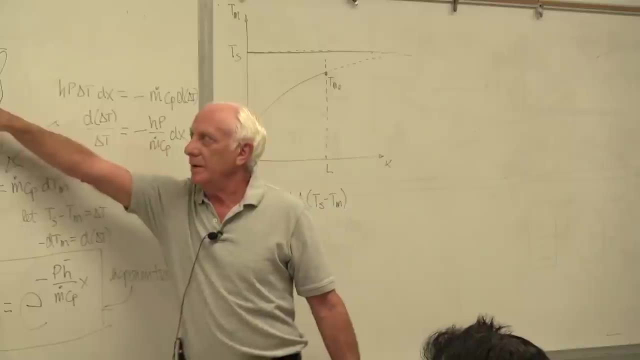 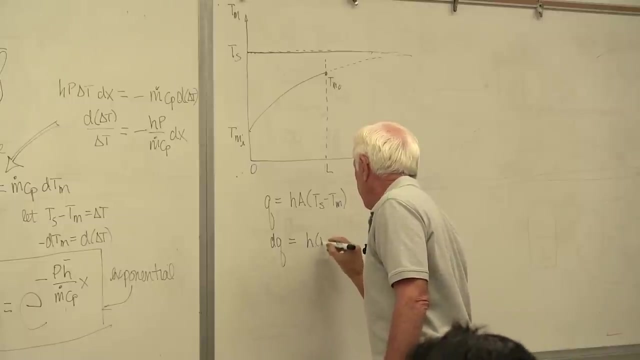 Okay, if I want to get my little DQ right here, okay, DQ in that little differential area is E, Equal to H, T, S minus T, M times my differential area And my differential area. there is circumference: pi D times the length X. 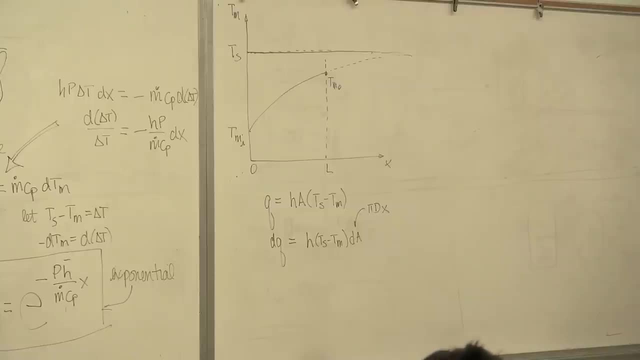 So D A is pi D X. Do you think this guy, when I integrate both sides now, You think I can pull him outside the integral sign? Uh-uh Over here in the fully developed region. can I pull out the T, S minus T mean fluid. 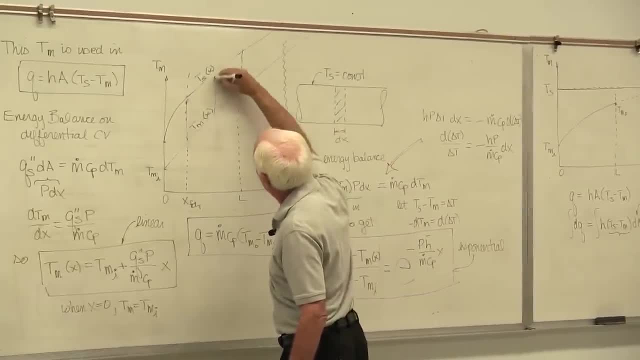 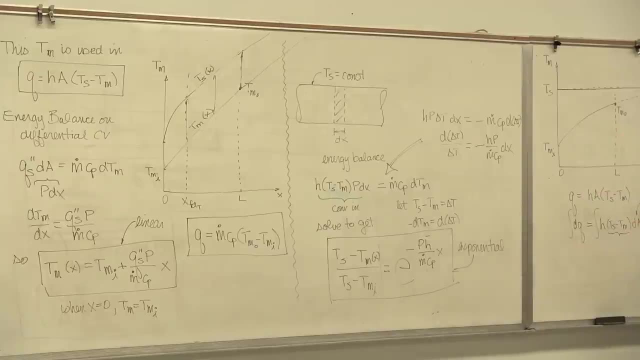 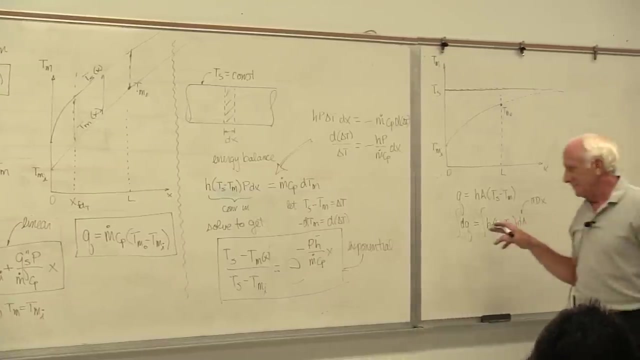 Yeah, because that is the same. no matter what X you're at, that is the same amount: T S minus T M. It can come outside the integral sign Here. it can't do it, Can't do it. So what do you have? 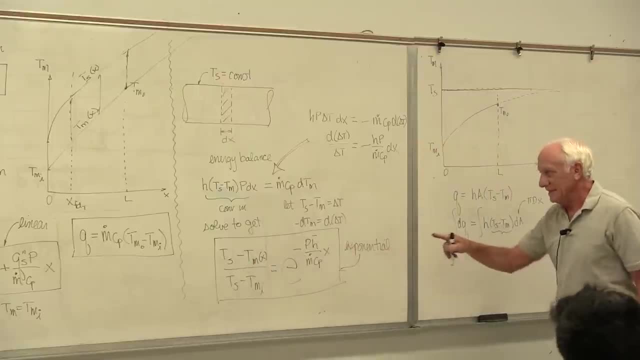 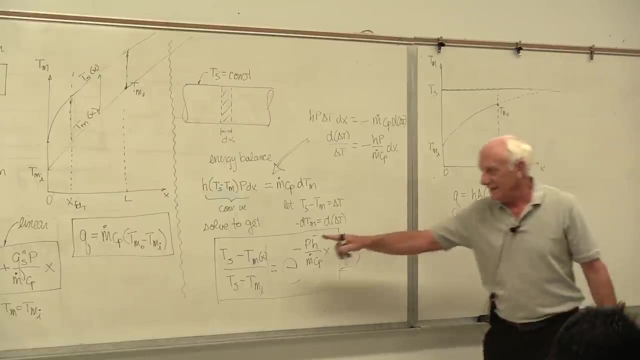 You have to do. see that T S right there, Minus T M. See that T S minus T M. Yeah, that's what you got to do. You put this guy into here and you carry it out. all the gory details of integration. 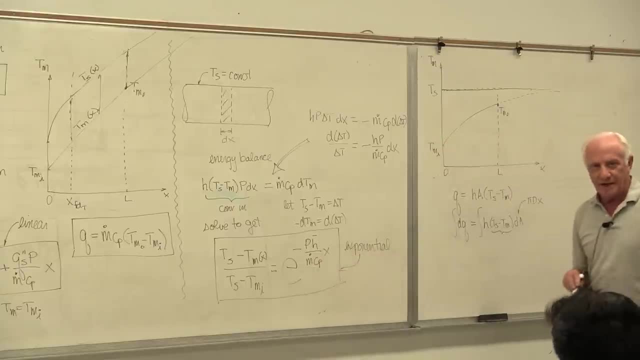 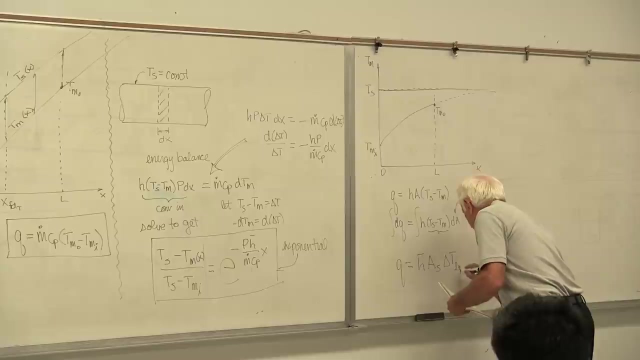 And when you integrate the exponential function, natural log, natural log. So what comes out is going to be a natural log. Here's what it amounts to: Q, Q equal H bar, the average H Surface area of the tube, A S times delta, T, with a subscript lowercase L, M. 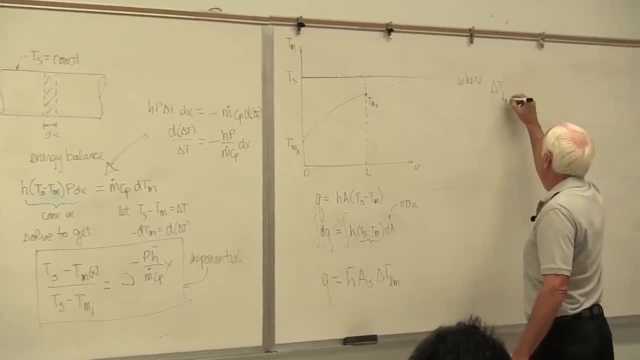 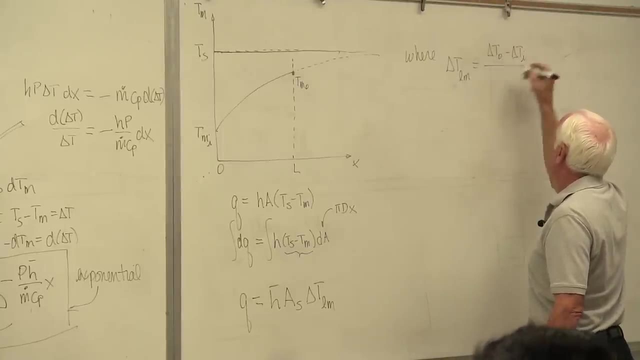 Where delta T lowercase L M equal this Delta T out minus delta T in divided by, there's a natural log. now, when you integrate it, natural log, Delta T out minus delta T in divided by, there's a natural log. now, when you integrate it, natural log. 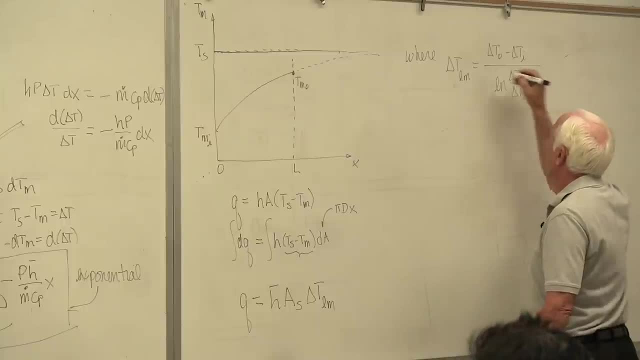 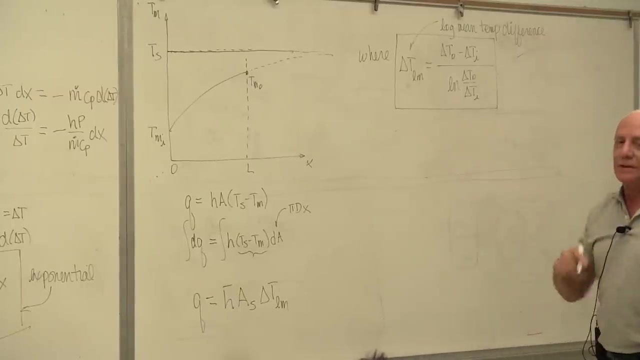 Delta T out over delta T in. That is called the logarithmic mean temperature difference or just the log mean temperature difference. It comes out of the integration. Okay, so it came from. And where do you put it? You put it down here in the equation. 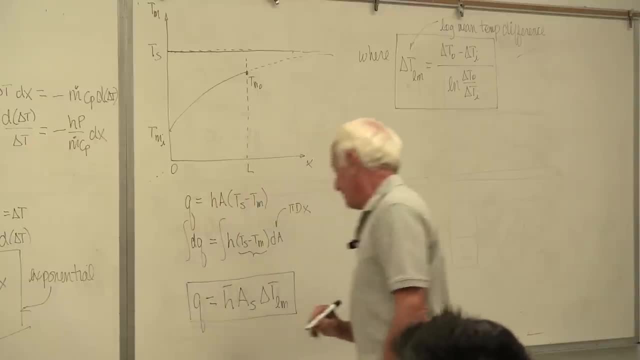 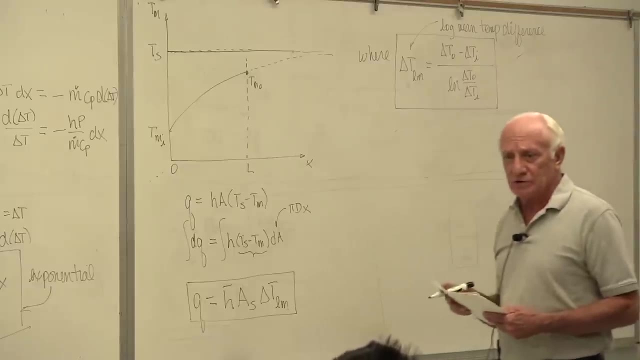 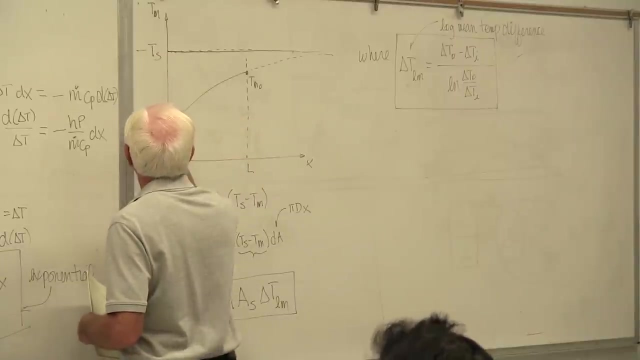 In the equation to get Q, What's delta T? The O stands for outlet, The I stands for inlet. What's delta T inlet? Okay, it's right here That's delta T inlet And where's outlet. That's from here to here. 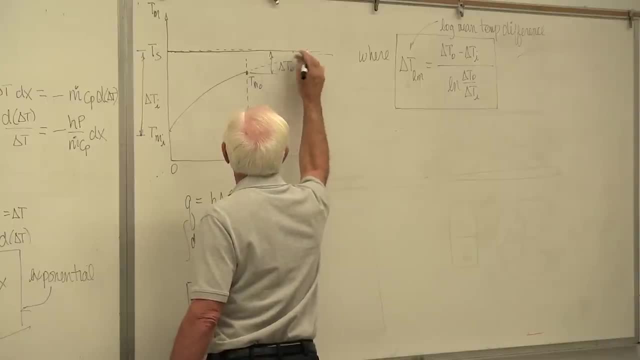 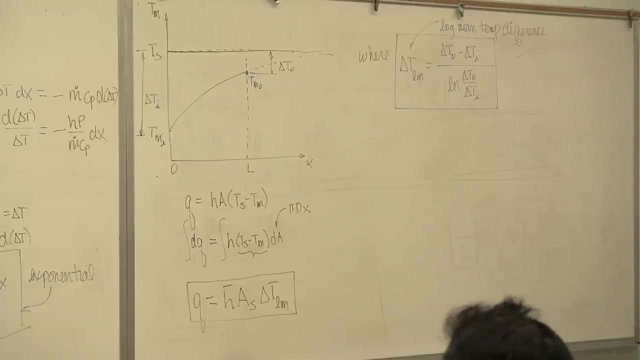 That's delta T outlet. There's how you find those two guys. All this stuff leads into heat exchanger analysis too. It's like a heat exchanger, obviously, a boiler, a condenser- Okay, It's more complicated than this guy- constant surface heat flux. 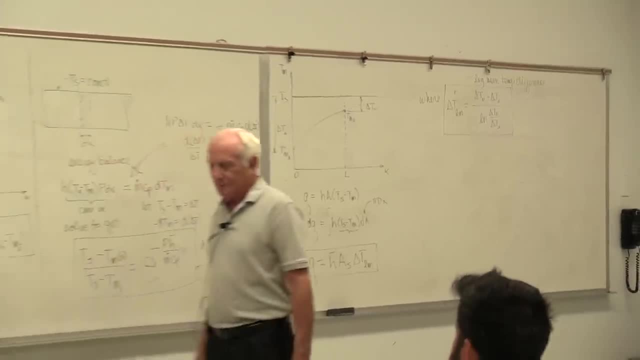 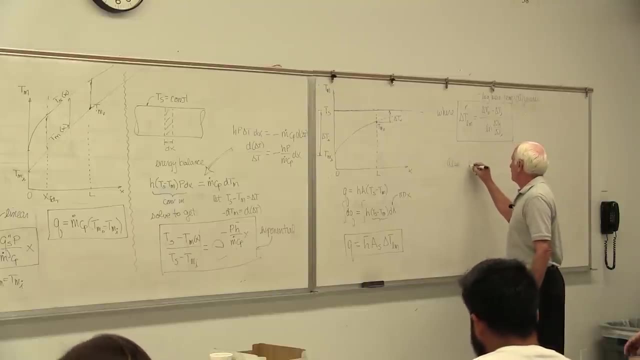 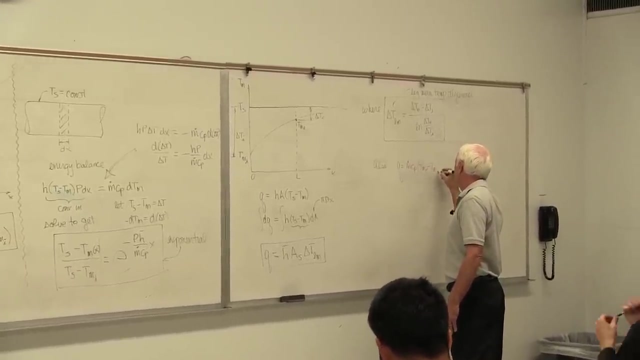 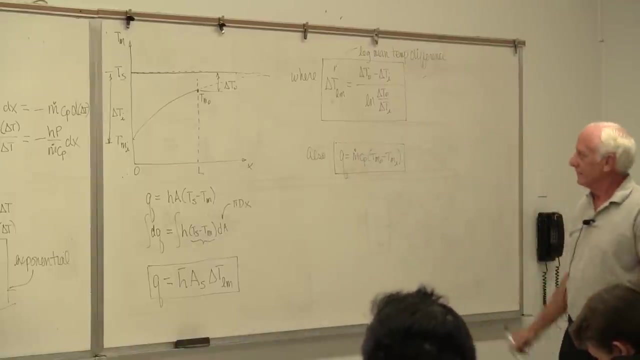 There's this guy: M dot C sub P, delta T. Of course, if you want to, you could also say: Q equal M dot C sub P. T mean out, minus T mean in, because that equation works for all these guys. It's here. 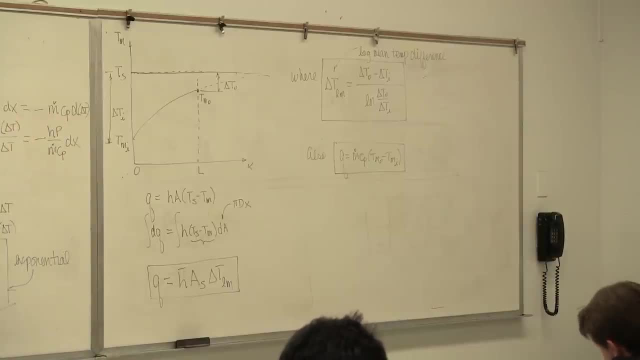 It's here: thermo M dot delta H, enthalpy M dot C, sub P delta T. So now we've got three main boxed equations. Let's look at them. For constant surface heat flux, how do you find the temperature anywhere along the tube? 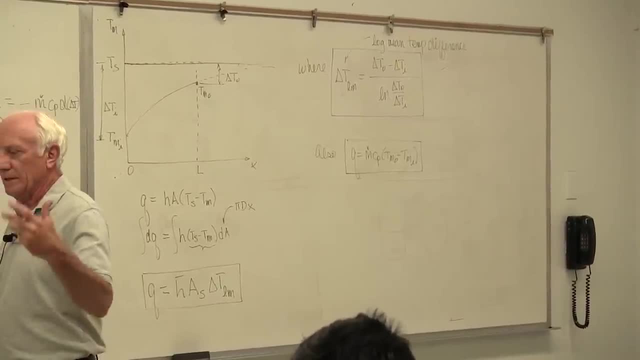 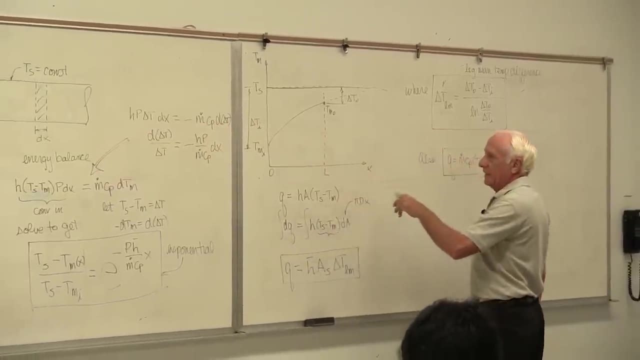 Here it is. How do you find the heat transfer that's occurred, or the heat added to the liquid, the fluid? Here it is Constant-tube surface temperature. how do you find the temperature at any X value? Here it is. 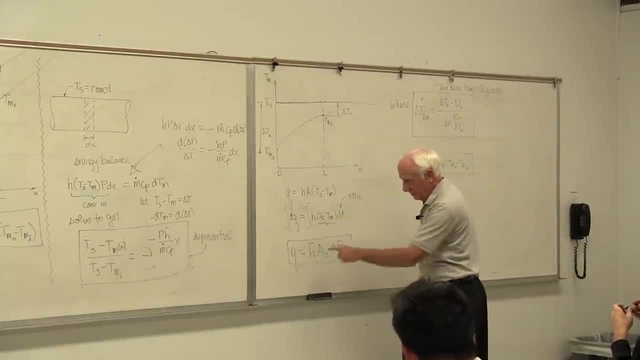 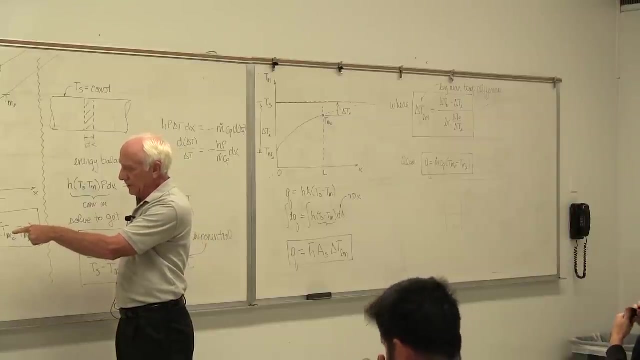 How do you find the heat transfer? either this equation or this equation, Okay. Okay, Over here I'm going to find the temperature at the end of the tube X equal L and the heat transfer from zero to L. Do I need to know the convection coefficient? 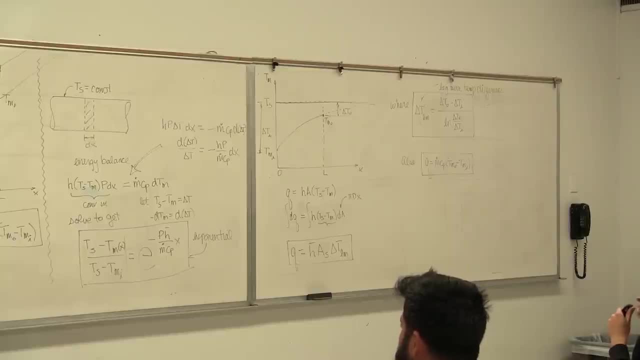 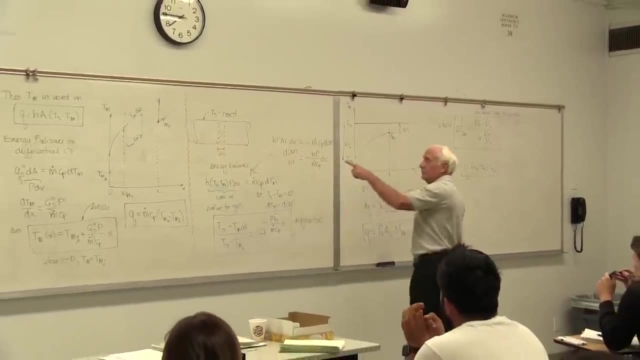 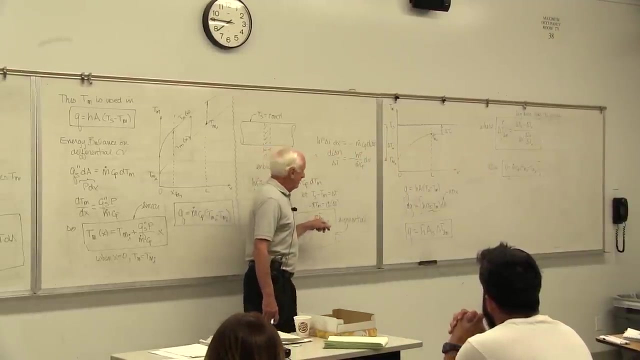 Look for H. No. Look for H, No. I don't need H. Constant-tube surface temperature. I want to find the temperature at the end of the tube. Okay, Look for H, Oh yeah. Look for H, Oh yeah. 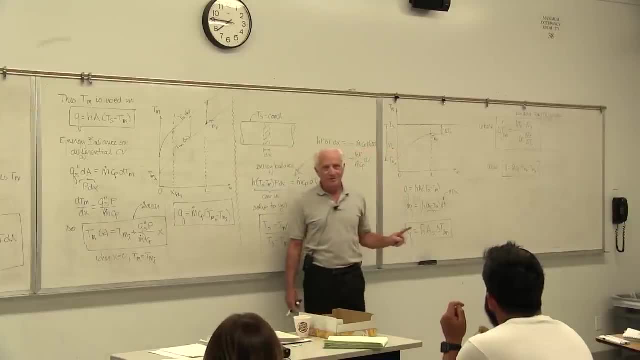 The heat transfer. Look for H. Oh yeah, You get the difference. You get the difference. You've got to find the H to find this temperature here. You don't need H to find Q, because you've got a choice Okay. 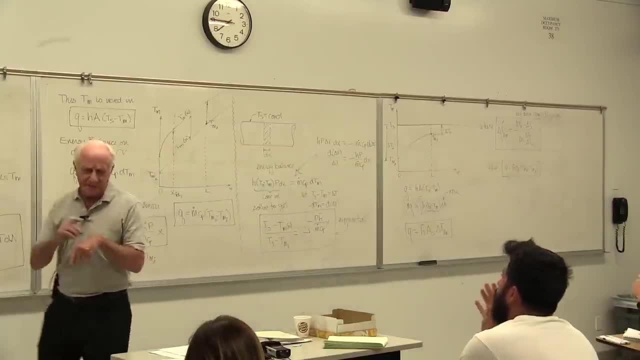 So just be aware of that. We're going to find H's no matter what. We'll find H for both cases next time, But for right now, just so you know, you don't need H for this guy to find Q and T Over. 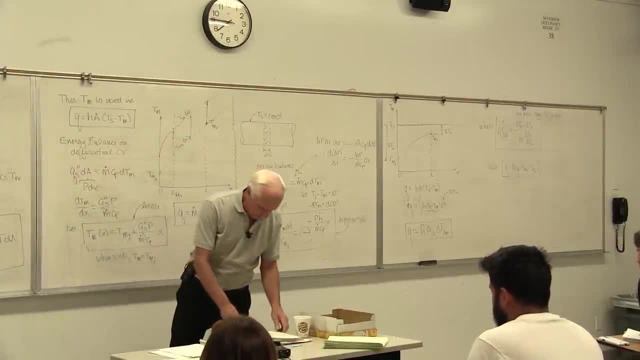 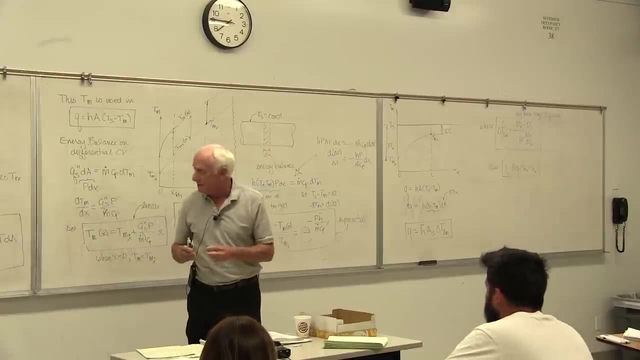 here you do need H. Okay, Okay, H to find this guy for the temperature. Okay, Now I'm going to go over homework, So we're going to pick this up next time and we're going to find the H's next time. So this is. 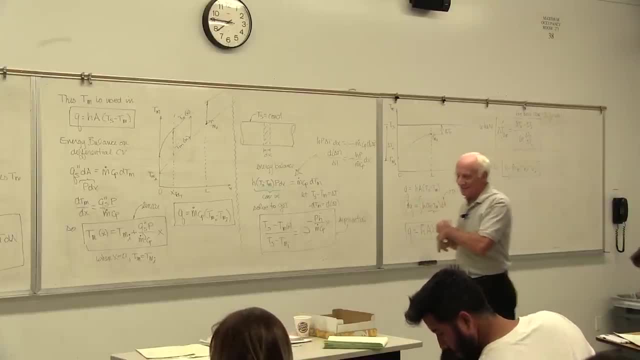 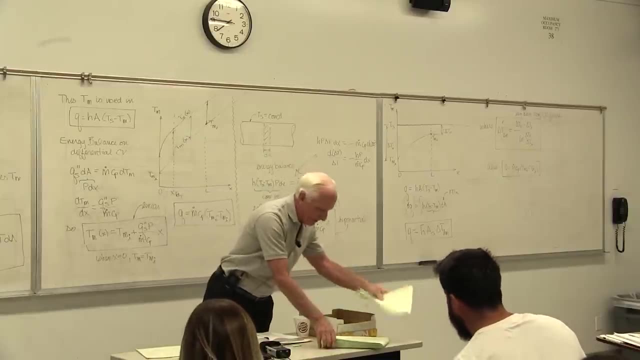 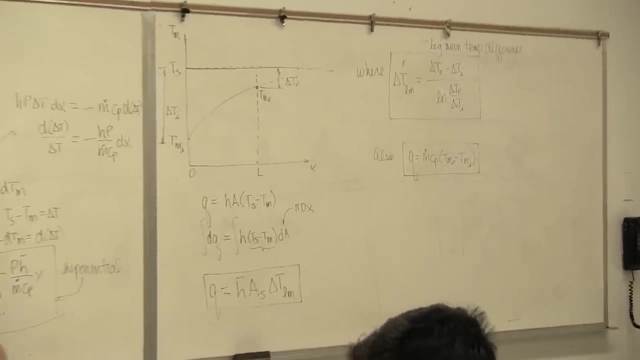 pretty much where we are in Chapter 8 right now. Okay, So let's shift gears and go to homework. If you came in late and didn't pick up your homework, it's up here in front. Okay, And we turned homework in today too. Set number 12.. All right, Just so you know. let's 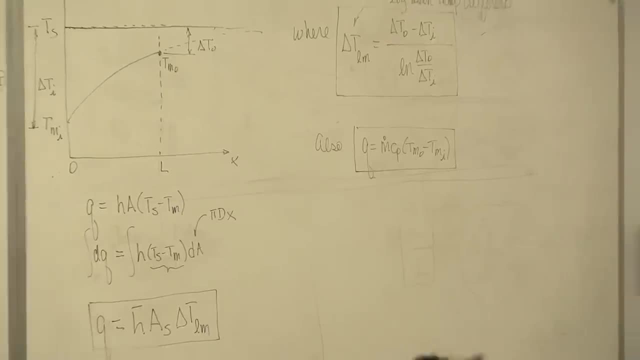 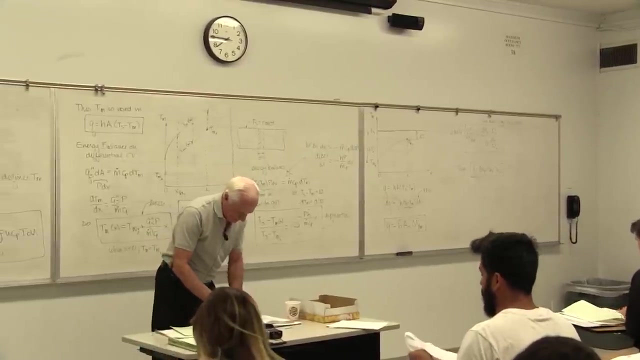 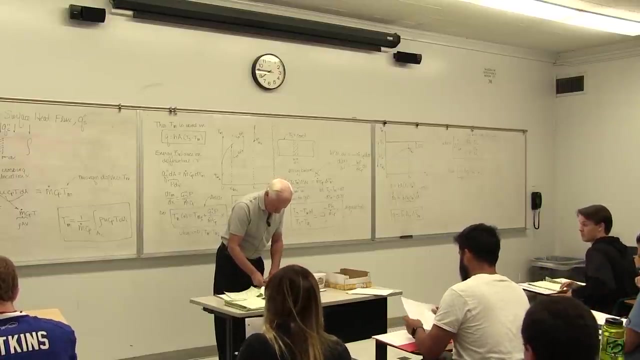 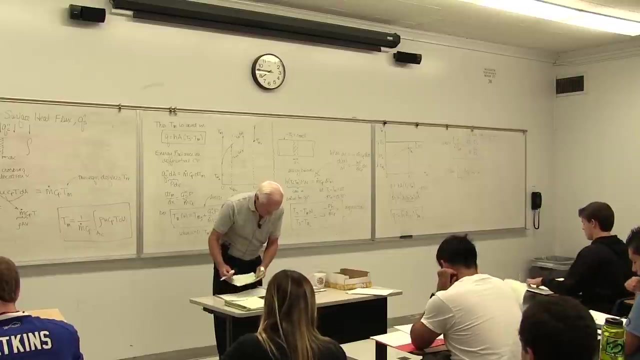 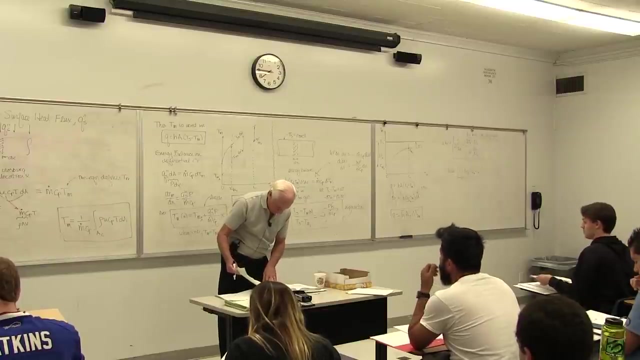 see, I guess I looked at I graded 612.. Let me see what I've got here. Yeah, 612.. They gave a picture. No, Okay, Okay, Yeah, Let me just read it again here. Oh, yeah, There, it is Okay, All right. 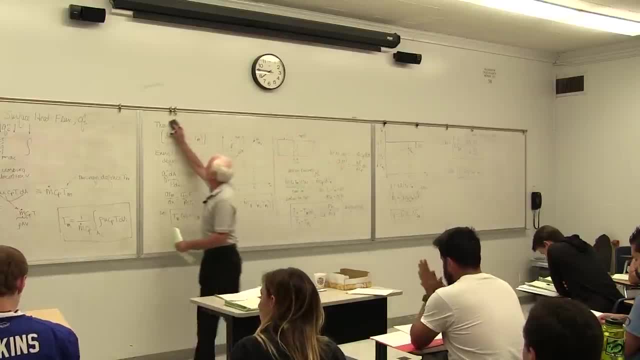 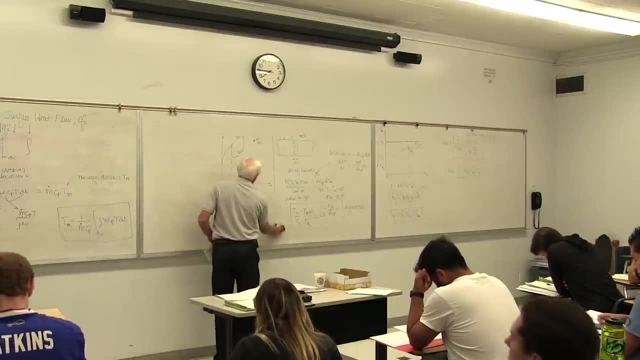 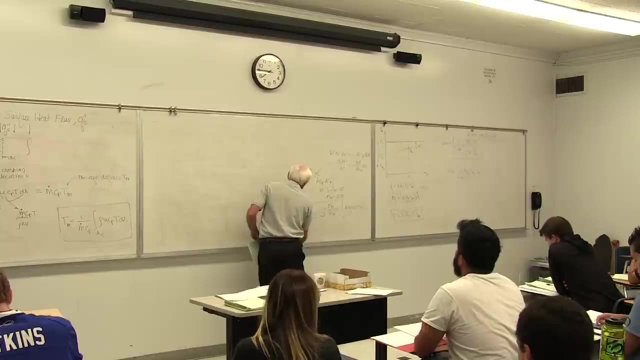 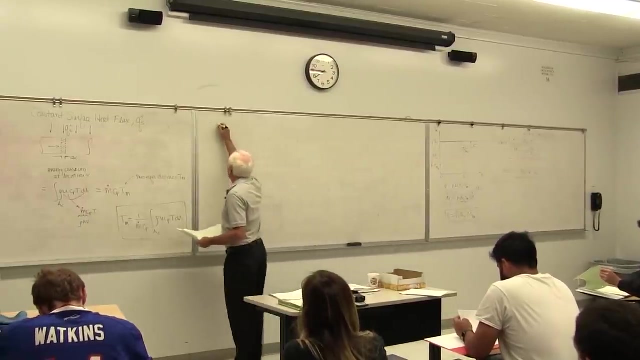 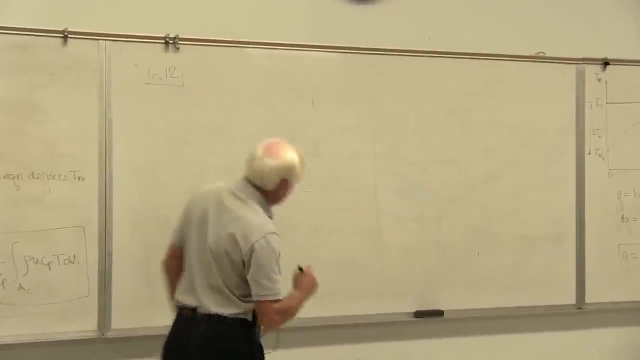 They gave a temperature profile, So let's look at 612.. Okay, All right, Okay, All right. They gave a temperature profile, So let's look at 612.. Okay, All right, Okay, Okay, Okay, All right. This is a flat plate. Yeah, Flat plate. flow like this And we have the approaching. 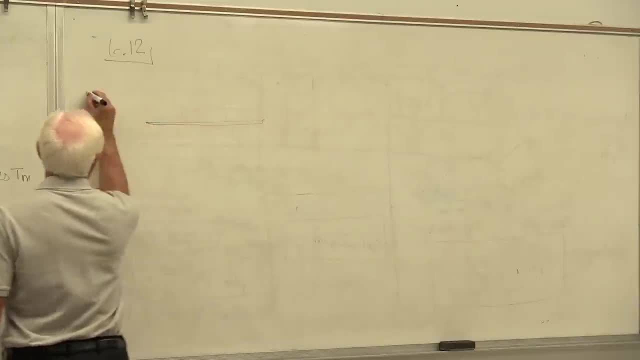 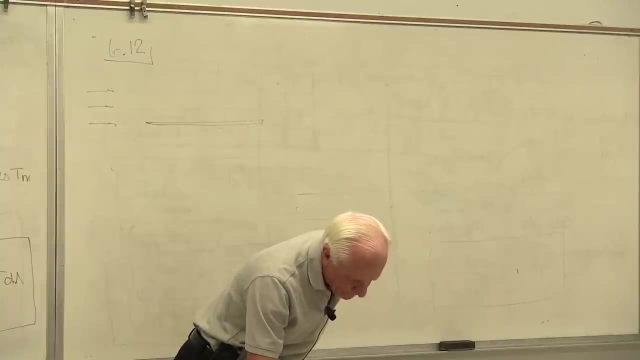 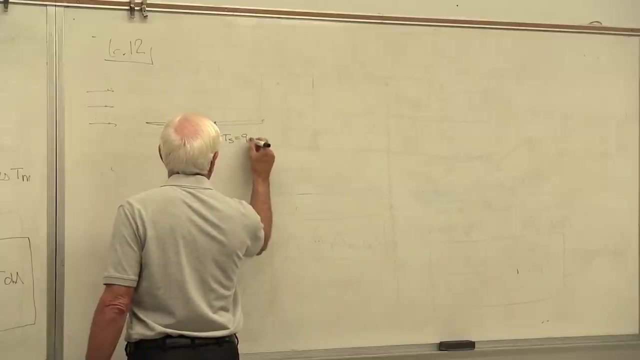 fluid stream and we have the approaching flow. All right, Okay, Till we go to the next lesson. All right, We're going to go to our next lesson. Okay, All right, Okay, have 30 degrees. Okay, T oh, T S. T infinity is 30, T? S is 90. So T? S is 90. T infinity. 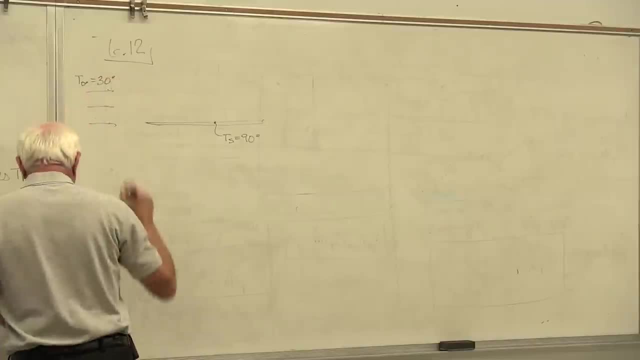 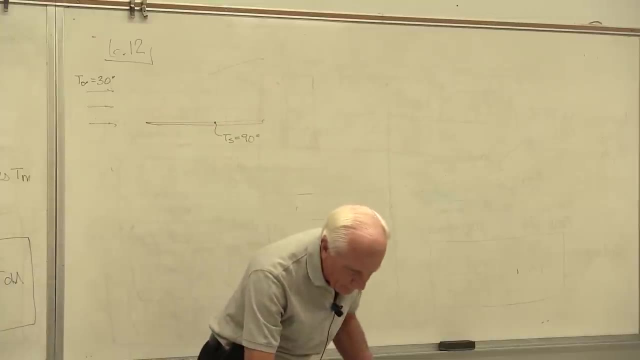 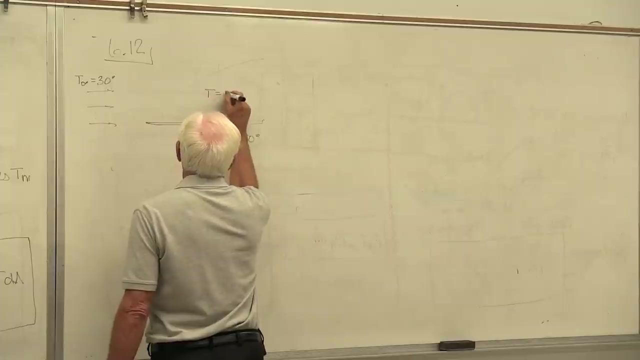 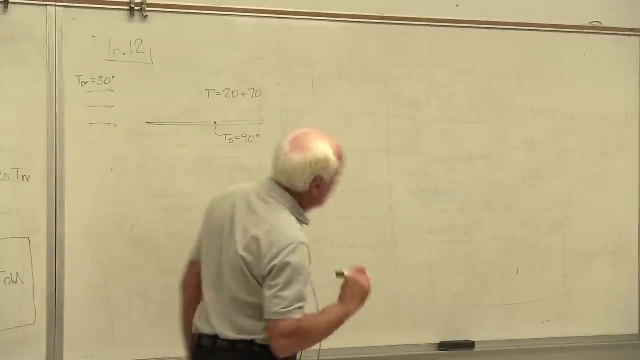 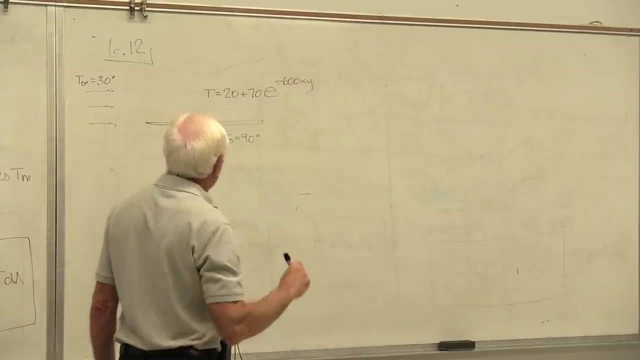 is 30.. Okay, He tells us that the temperature in the boundary layer T is 20 plus 70.. E to the minus 600 XY. Okay, So temperature is a function of X and Y. We're measuring X from here. We're measuring. 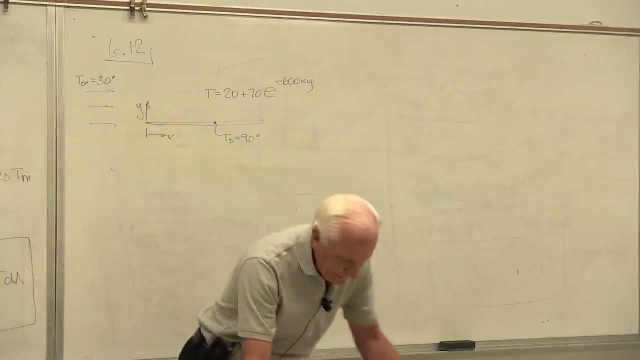 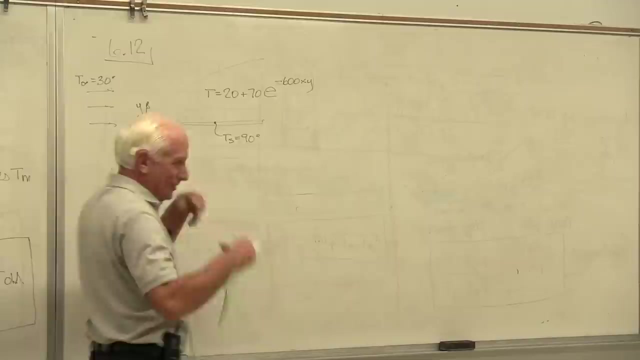 Y from here. Okay, I think this is okay. I'll just read it. It says: obstacles are placed in the flow which intensifies the mixing with increased distance. X from the leading edge. Somehow he's put something on that plate which causes more mixing, I don't know what. 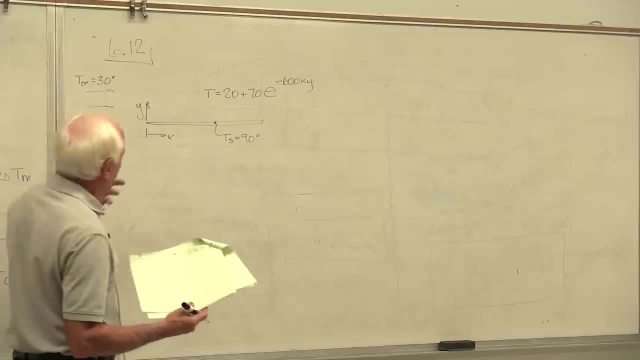 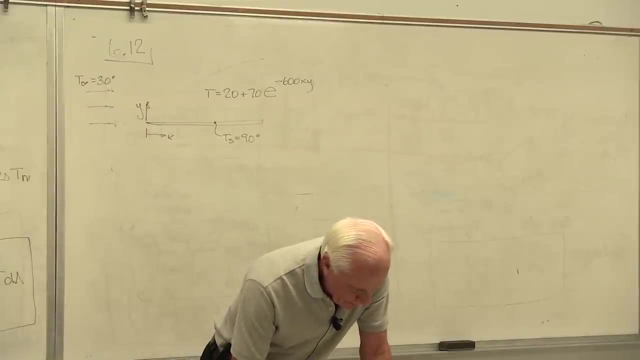 they are Little bumps on there or something. So the further down you go, the more mixing occurs. So he's artificially done something to the surface. Okay, Determine and plot the manner in which the local convection coefficient H varies with X. then evaluate the average. 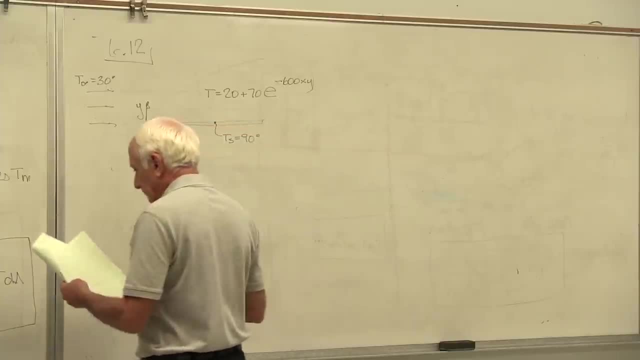 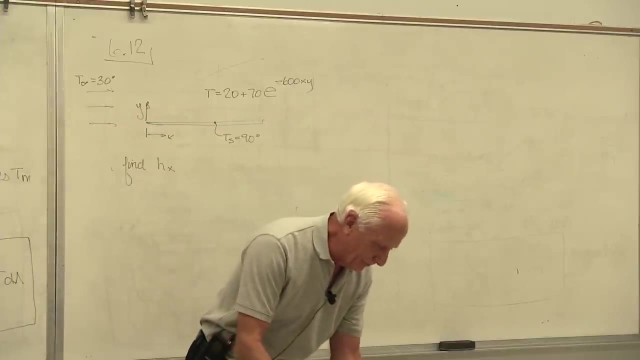 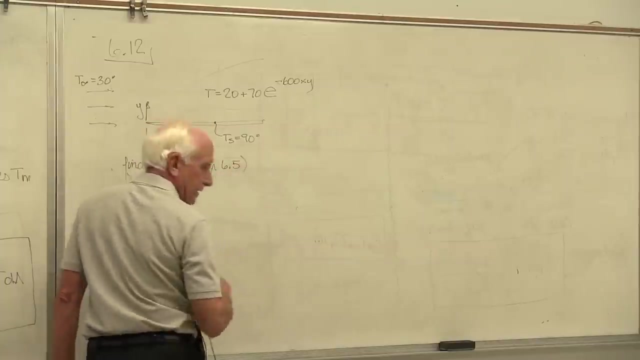 coefficient over the whole plate. Okay, So find HX. Okay, Now you can go through all that again if you want, but the equation in the textbook I'll look at here, Equation 6.5,. he says that HX equal minus K, partial T with respect to: 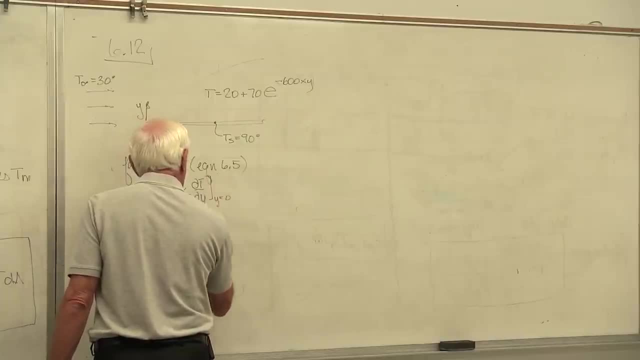 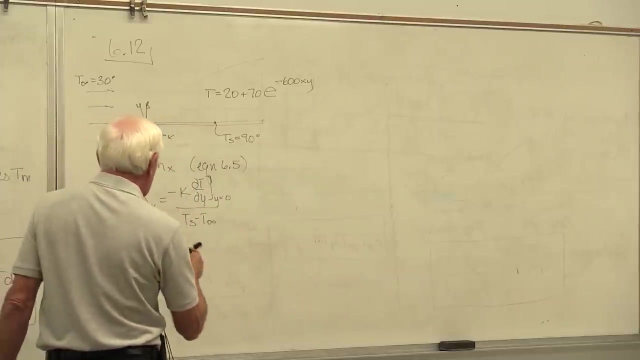 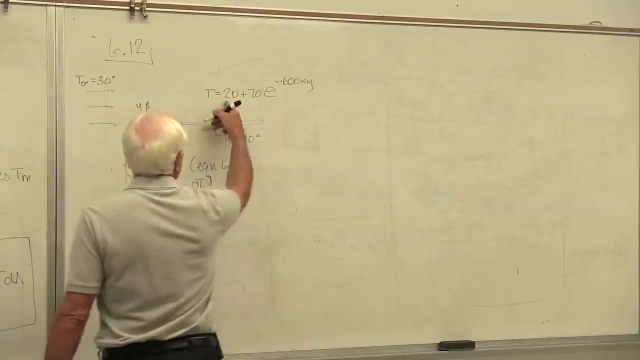 to Y, at Y equals 0 divided by TS minus T. infinity. Yeah, Okay, that's part A. then you have to find this guy. So there's this guy. Partial of T with respect to Y constant: 0, 70 minus. 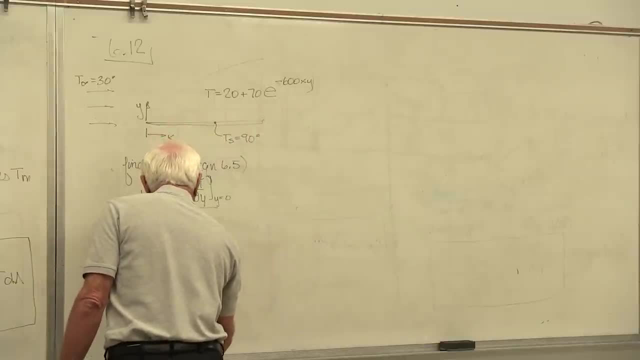 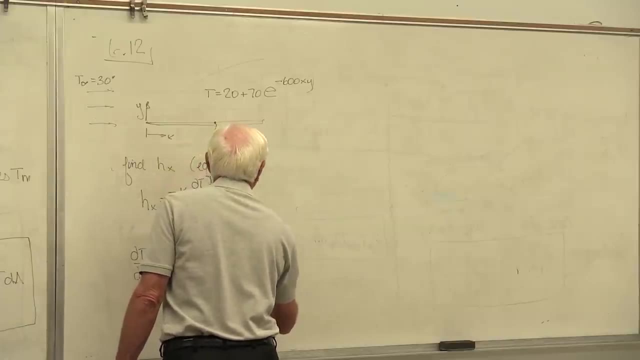 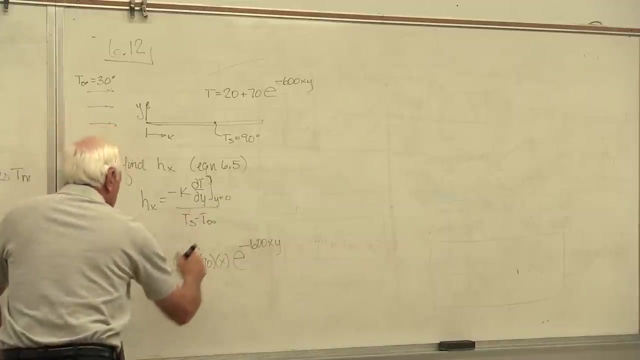 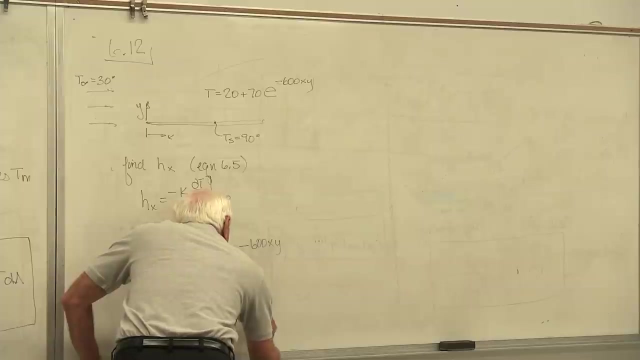 600 times X times 70.. E to the minus 600XY. Now do what it says: Partial T with respect to Y at Y equals 0. 600 times 70, E to the minus 600XY, 70 times X times E to the minus 600XY. But this says: where Y equals 0. Y equals 0. E. 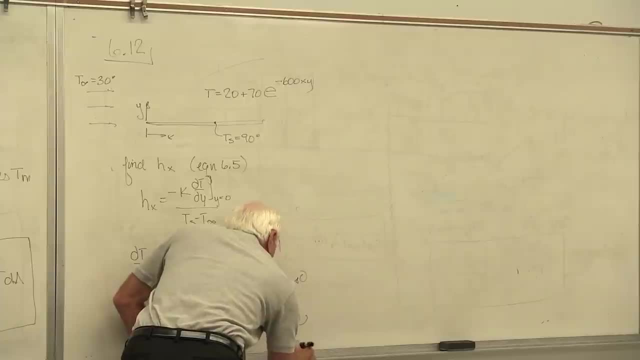 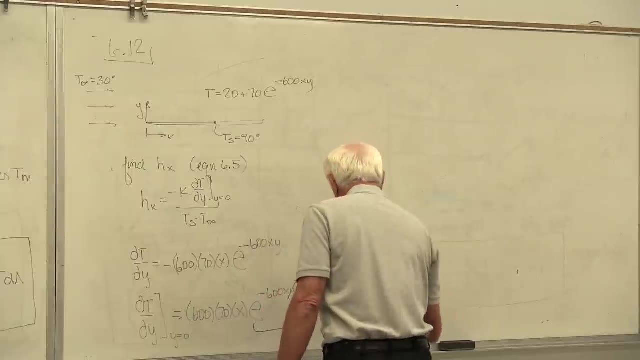 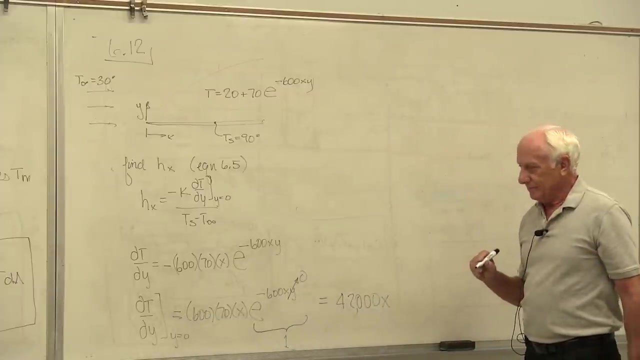 to the 0 is 1.. So DT DY at Y equals 0, is equal to 42 times the three 0s times X. Okay, What I'm saying is: don't get sloppy in your math, They come back and bite you. 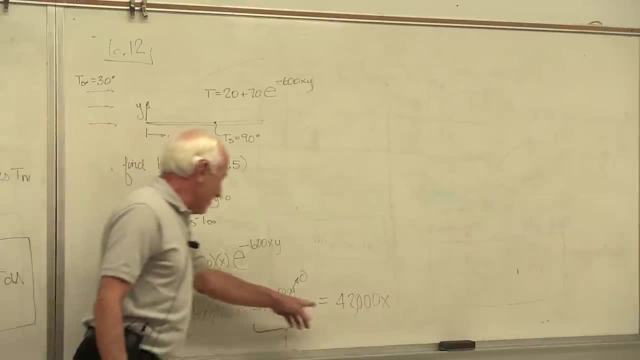 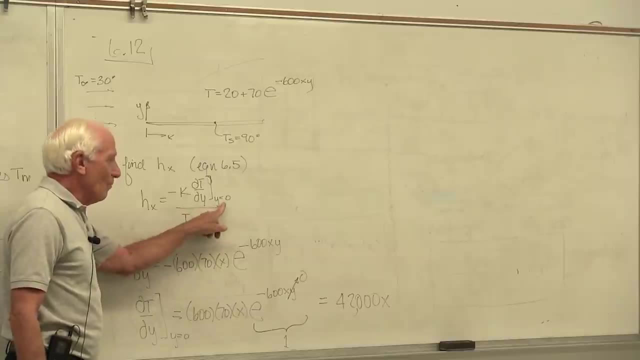 I saw a lot of people that said DT DY is 42,000X. Oh no, it's not DT DY. is this whole long thing? This thing says: once you get DT DY, but get DT DY first, Then once. 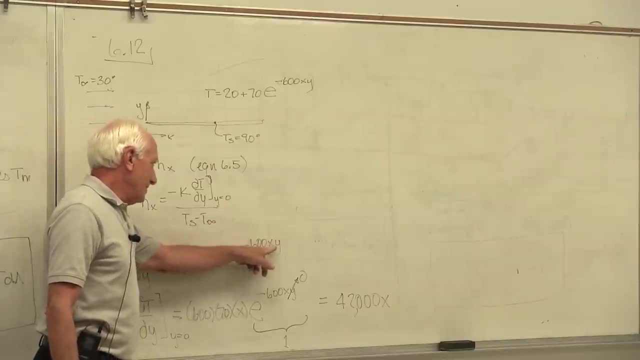 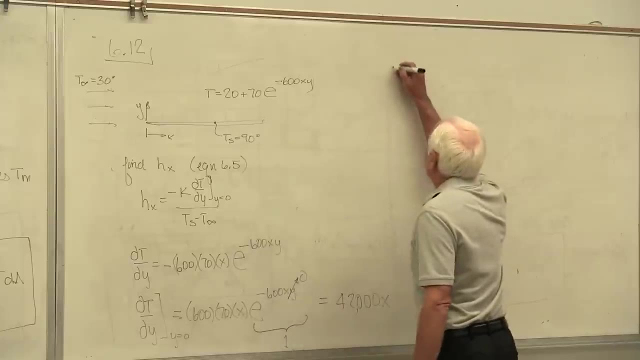 you've done that, then you put Y equal to 0.. You can take shortcuts, but you better be careful, because DT DY is not 42,000X, 62,000X. Okay, now I plot it: HX versus X: 0.. Here it is right. here We start: X equal 0, it's 0..